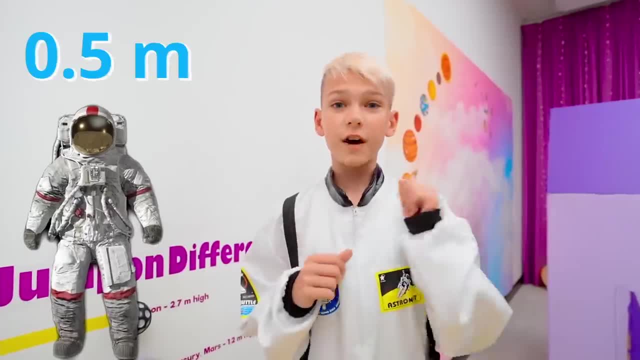 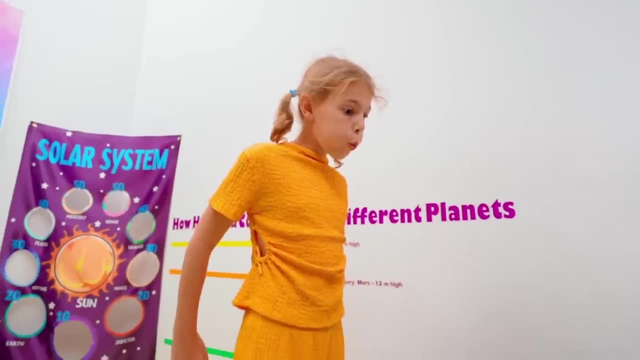 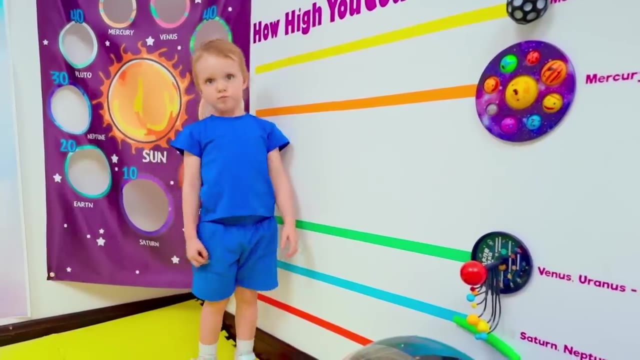 That's why an average human can only jump up to 0.5 meters. That's why you can jump on other planets. Sounds interesting? Let's go. Woohoo Dance, Wow Dasha. You just jumped as high as you can jump on Saturn and Neptune. 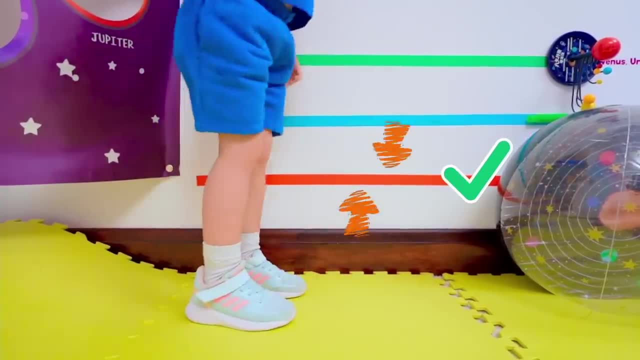 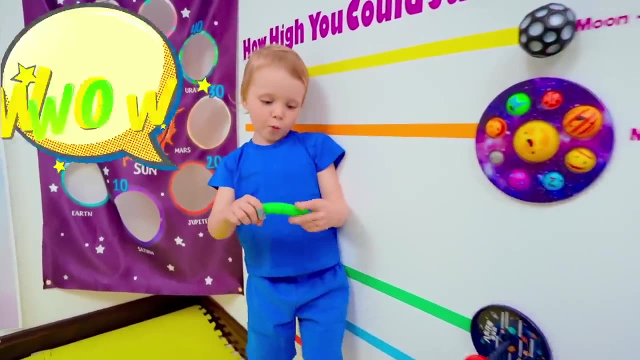 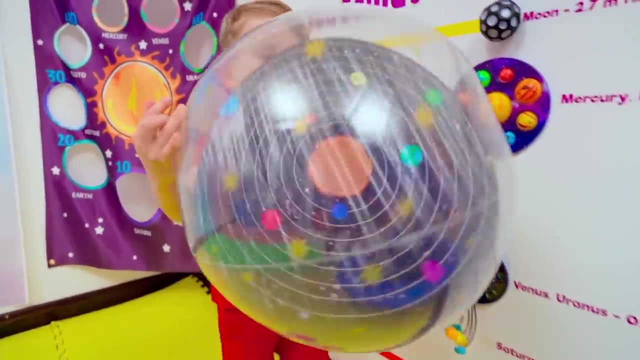 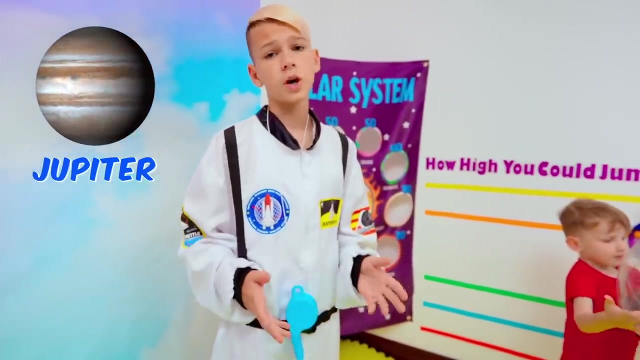 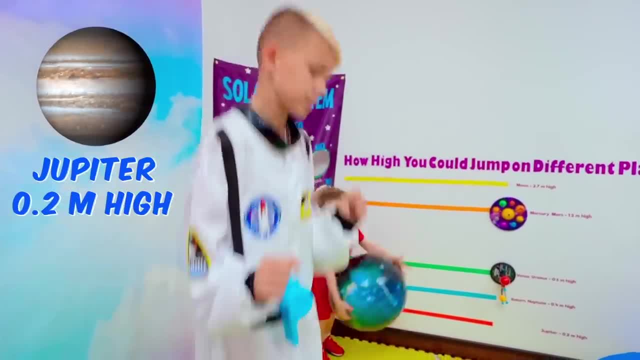 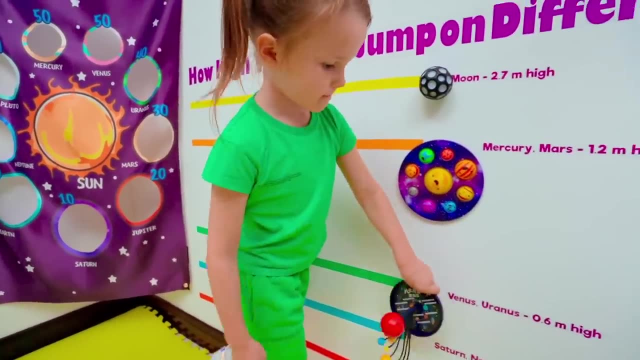 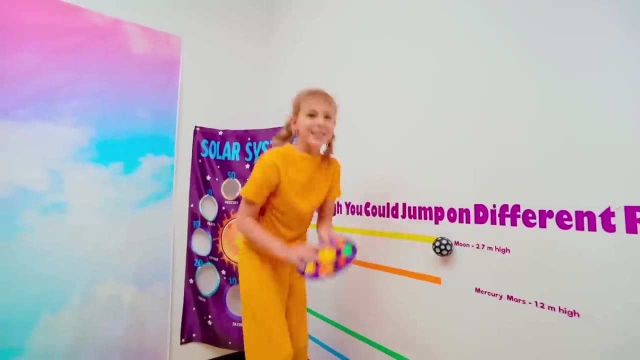 But if you want, you can hop on 0.2 meters. I want to jump to the moon and back. Oh yes, Almost, Whoo, Uh-huh. Oh yes, Wow, Woohoo. Iron, dangerous duck. 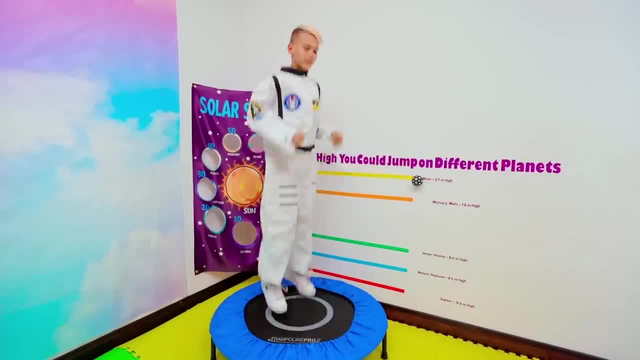 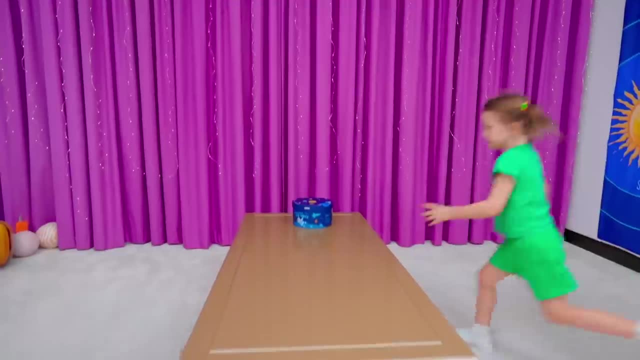 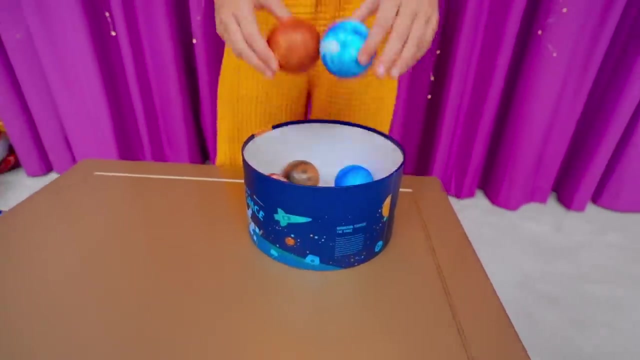 lactose intolerant, YUM. Go Go, Go. Yeah, Go Go Go. Let's play a multiple challenge with mini planets. Sounds good, Let's do it. Wow, Oh yes, Go Go Go. 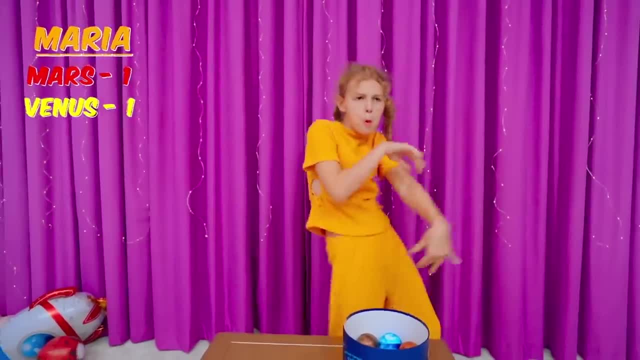 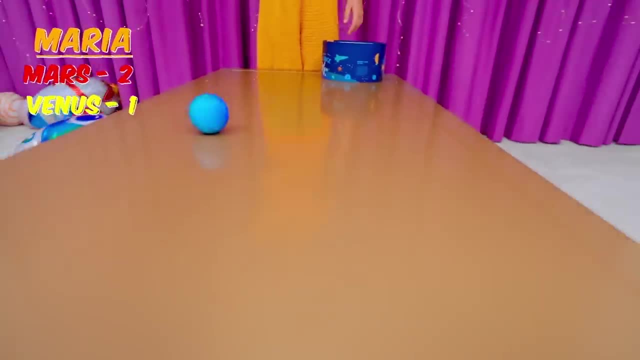 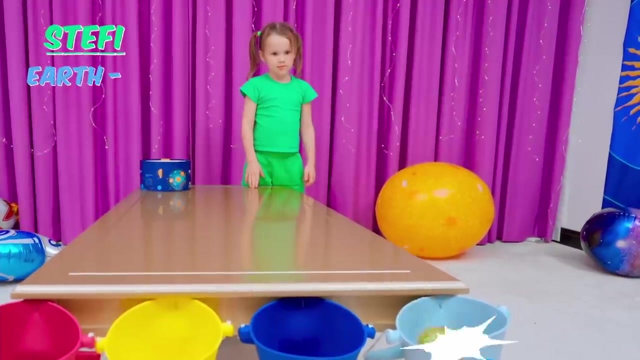 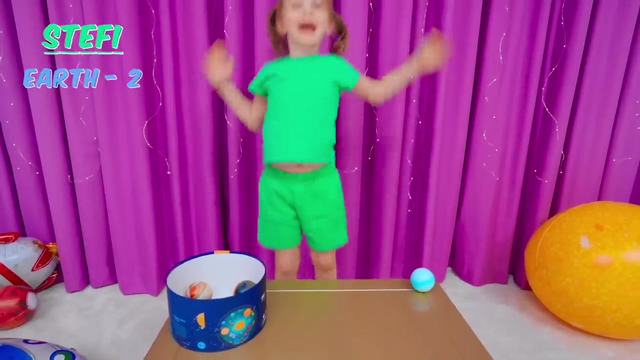 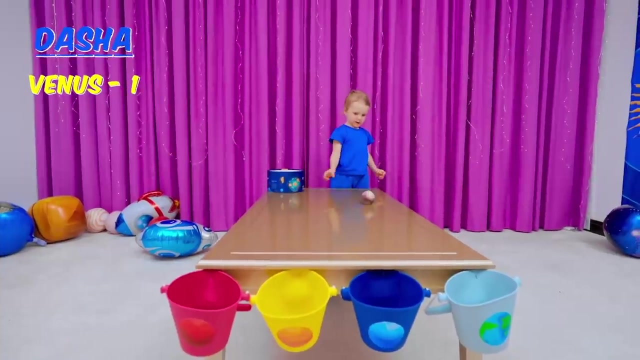 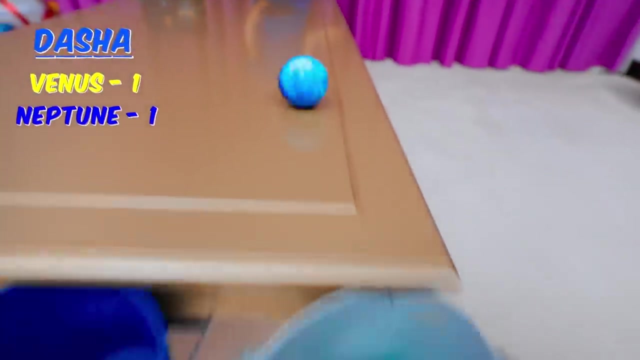 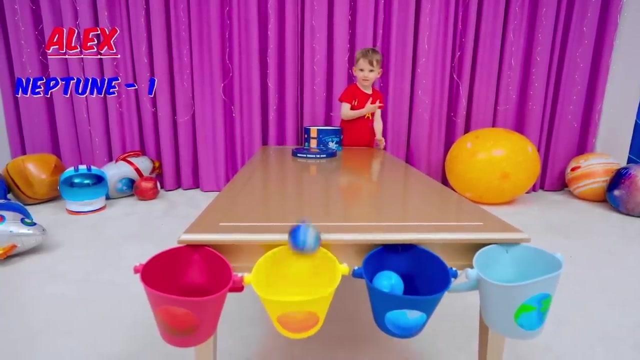 Go Go. Oh, go go go, Wow, Let's go. What Whoa Yeah, Wow, Go Go Go, Let's go Go, go go, Wow, Woo-hoo-hoo Excellent. 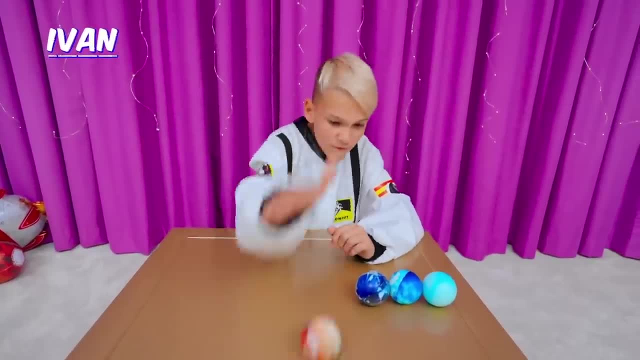 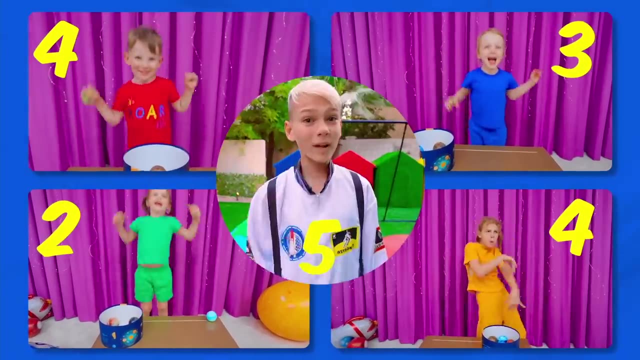 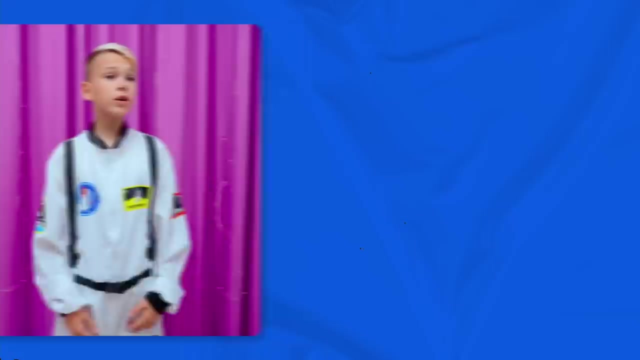 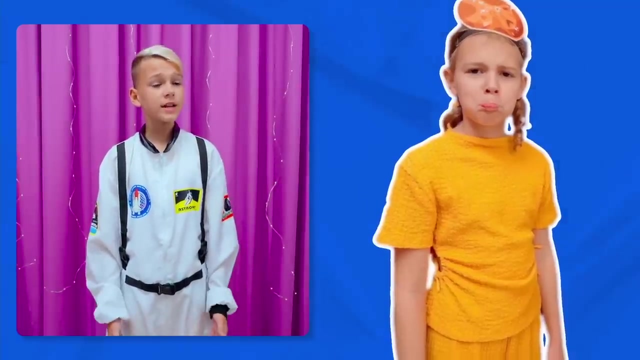 Woo-hoo, Woo-hoo, Woo-hoo-hoo, Hmm, Huh, Wow. I'm going to ask questions about the solar system and the planets. You have to answer them correctly. If you don't answer questions correctly, you have to cut a ribbon from the planet. 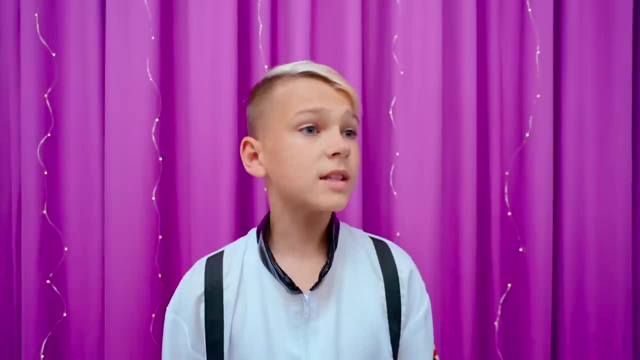 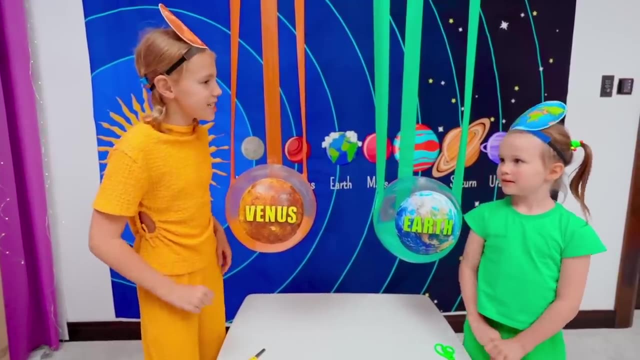 Oh yeah, okay, You have 10 seconds to answer a question. Is everything clear? Yes, Are you ready to find out who will be first? Let's decide with rock paper scissors. Rock Paper Scissors- Shoot. 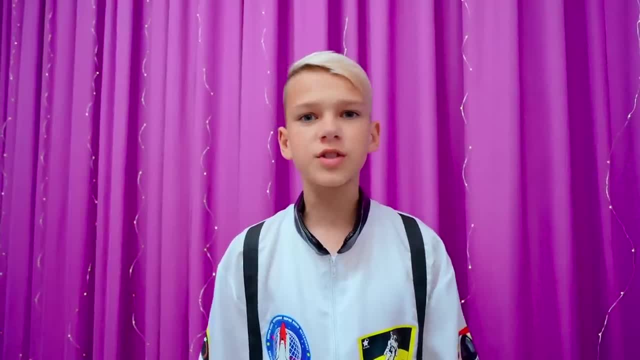 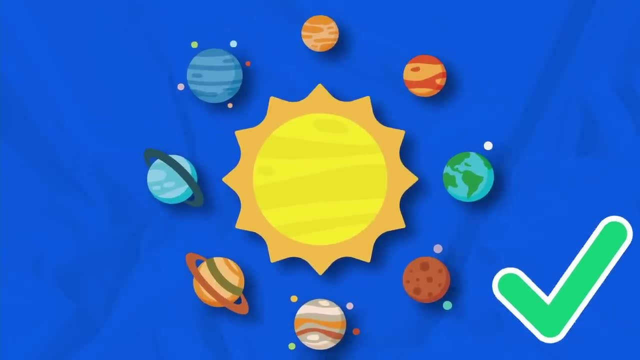 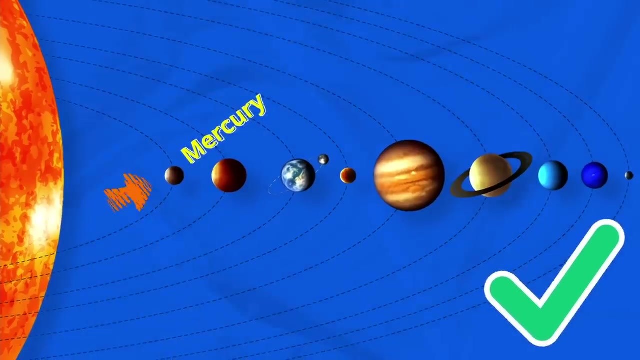 I'm first. How many planets are there in the solar system? There are 8 planets in the solar system. Nice, Correct. Which planet is the closest to the sun? Mercury. Well done, Steffi, Go, go go. 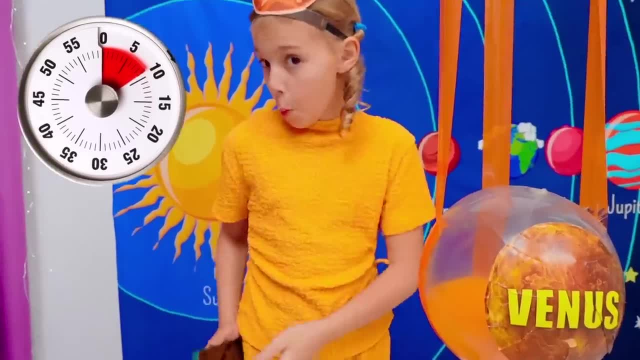 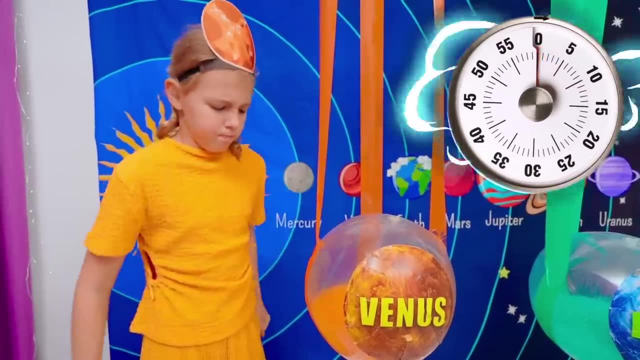 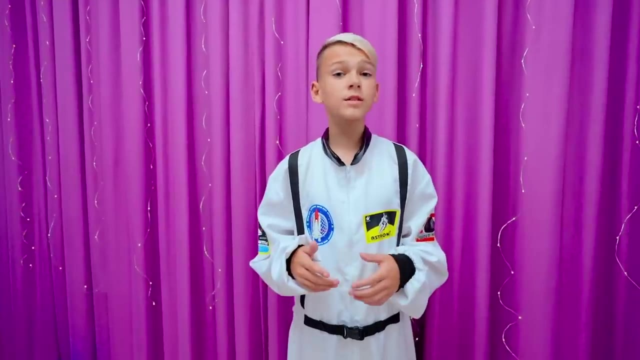 Which planet is the farthest from the sun? Hmm, Huh, Hey, Uh-uh-uh, Uh-uh-uh. Oops, no way, Neptune. What galaxy is the solar system located in? Something about Milky Way? I know Milky Way. 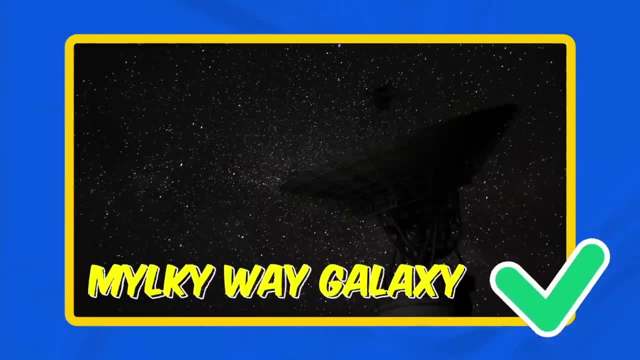 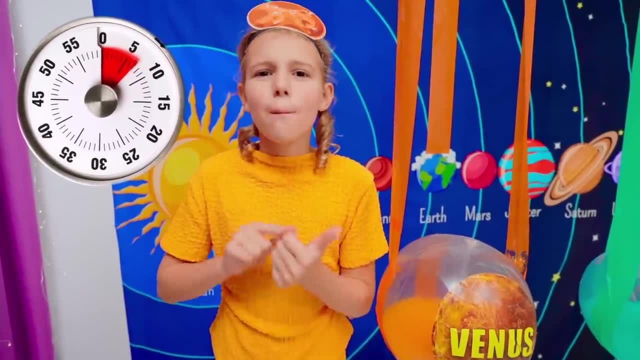 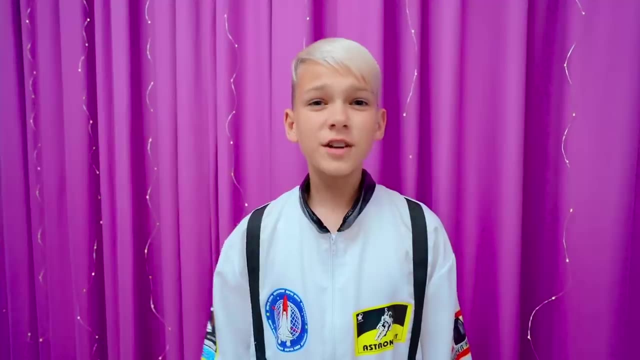 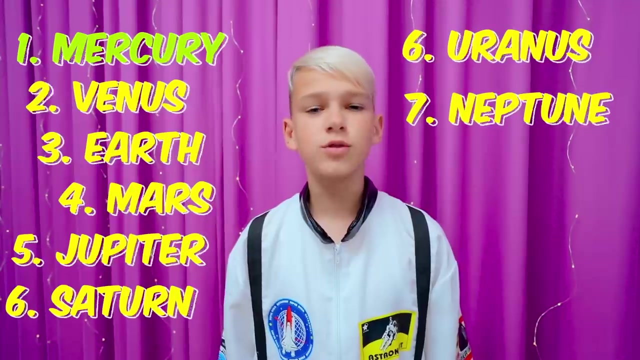 Yes, the Milky Way galaxy. Now name the planets in their order: Earth, Mercury, Venus, Mars, Jupiter, Saturn, Uranus, Neptune. Well done, Maria, But first comes Mercury, then Venus, then Earth, Mars, Jupiter, Saturn, Uranus and Neptune. 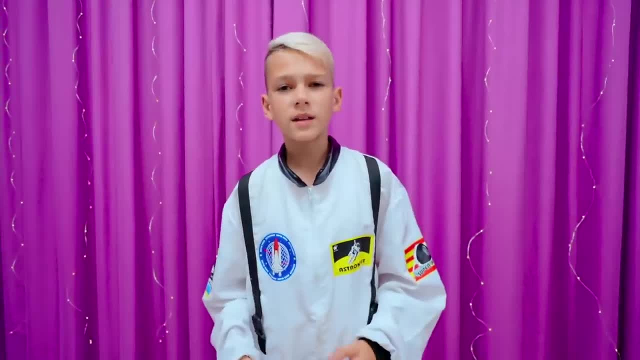 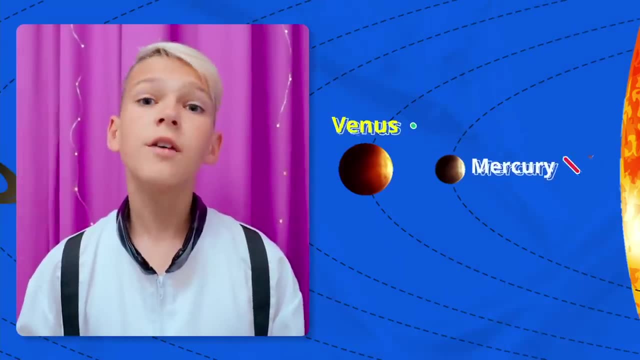 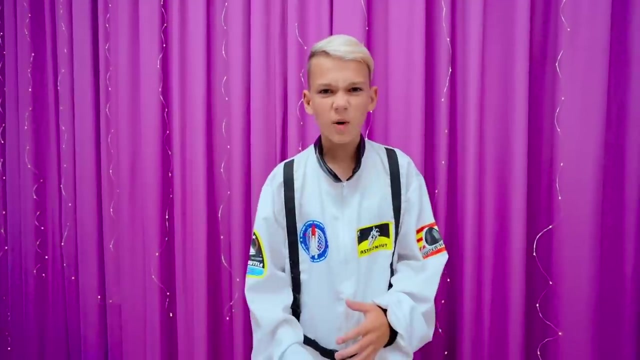 No way. Which planet is the hottest one in our solar system? Mercury. Even though Mercury is closer to the Sun than Venus, Venus is the hottest one in our solar system. Now, which planet is the fastest one? Maybe Mars. It's so red, probably because it's moving so fast. 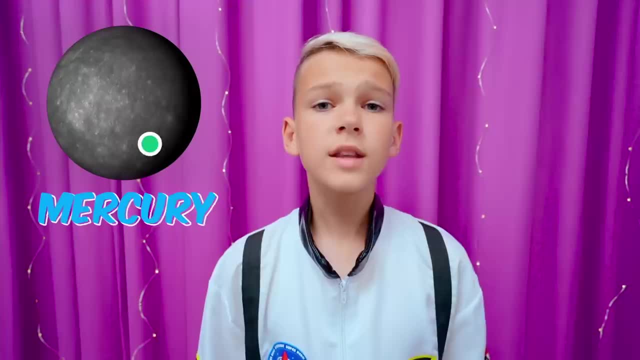 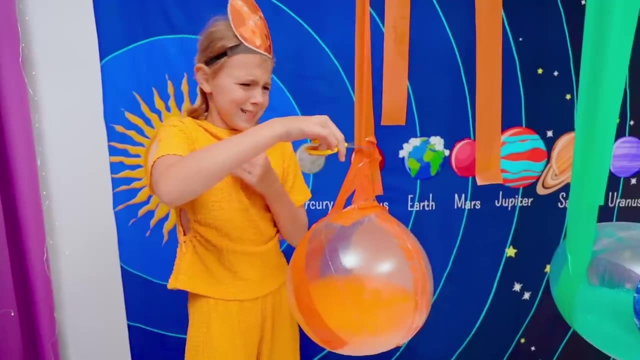 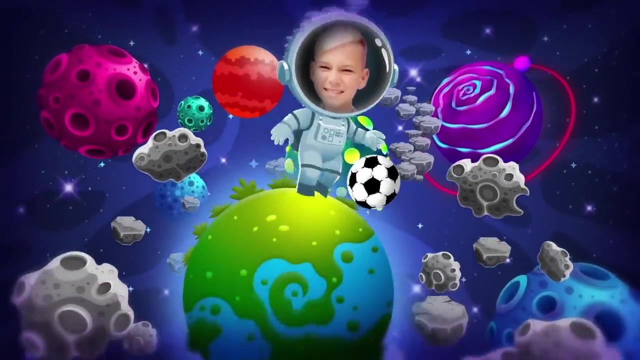 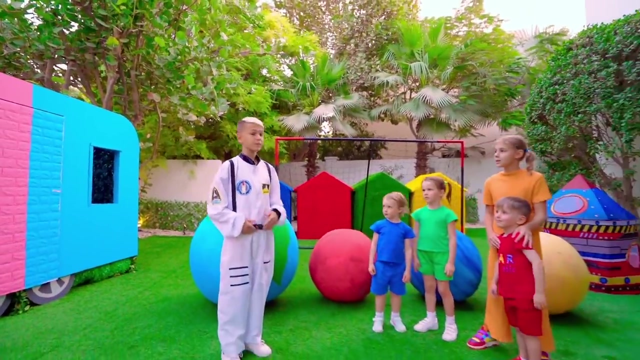 Unfortunately, no Mercury. This planet has the shortest year in our solar system- 88 days- and is considered as the fastest. No way, Yes. Now I want to show you the difference between the sizes of the planets: It's in balls. 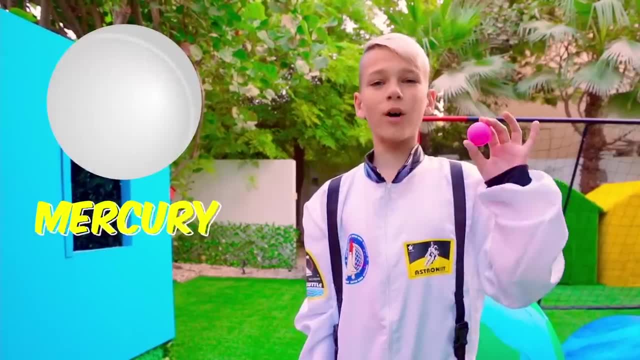 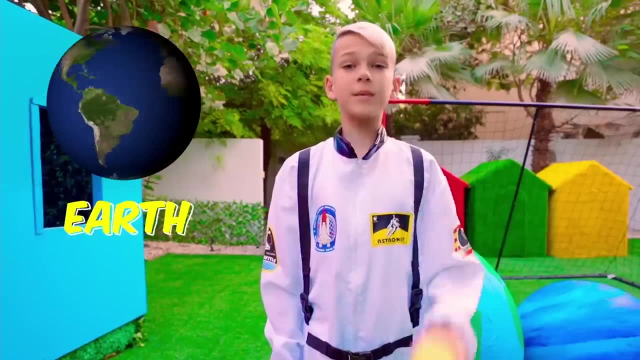 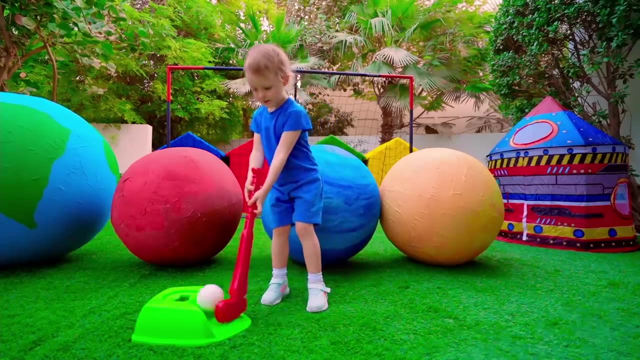 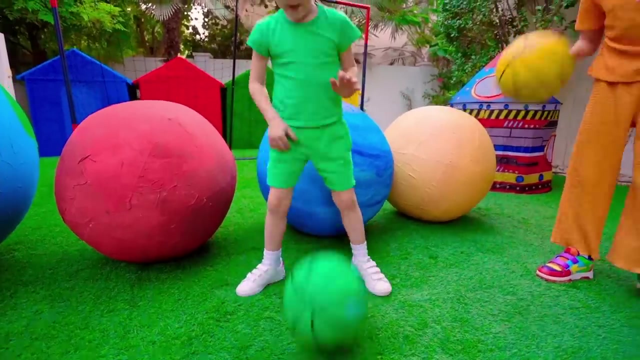 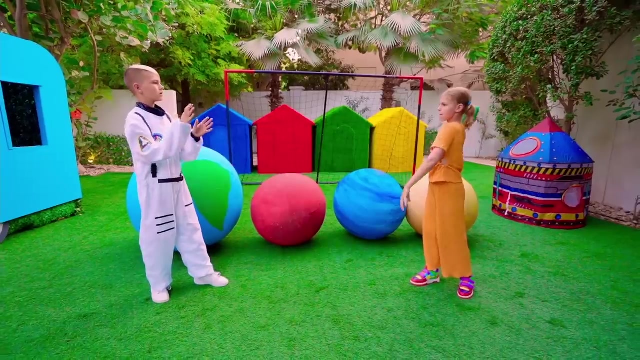 Okay, Mercury is a pink ball. Venus is a tennis ball- Oh yes, Earth is a baseball, Let's go. Mars is a golf ball, Excellent. Jupiter is a basketball. Oh yes, Saturn is a football, Let's go. 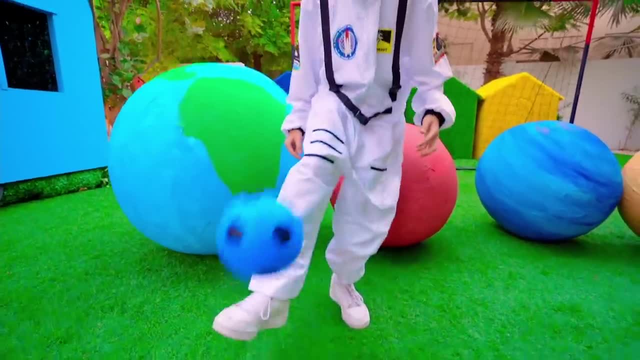 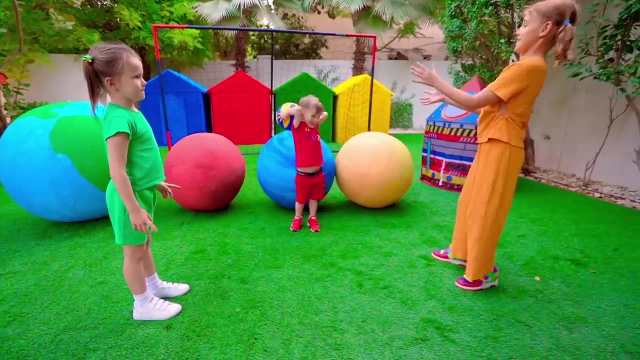 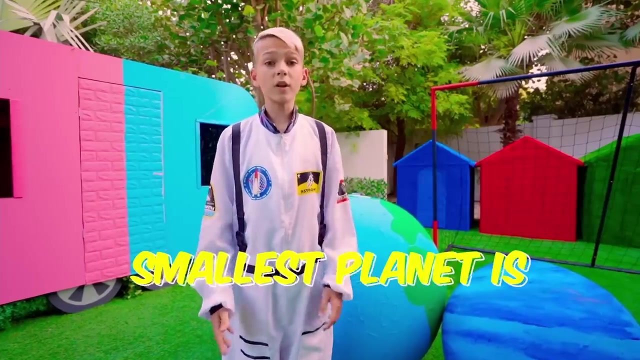 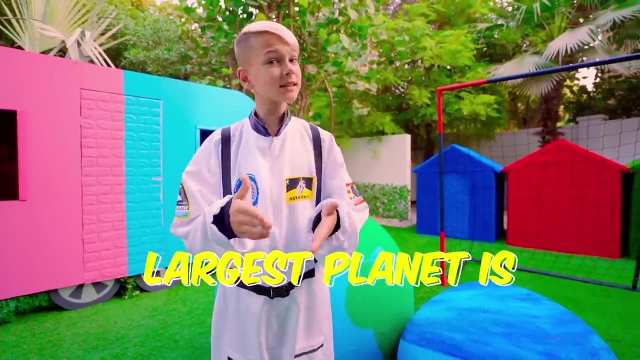 Uranus is a soccer ball- Wow, Awesome. Wow. Neptune is a volleyball- Great And the smallest planet in the solar system is Mercury And the largest planet is Jupiter. You have mastered all the information very well, Well done. 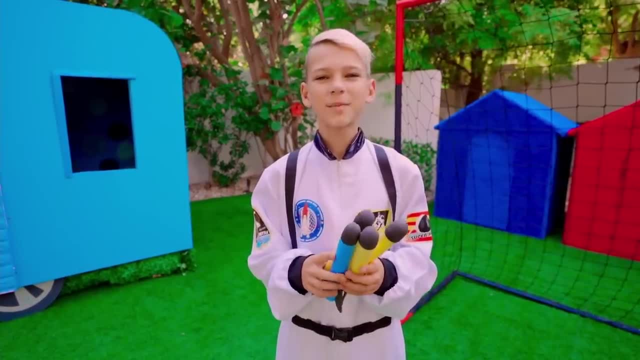 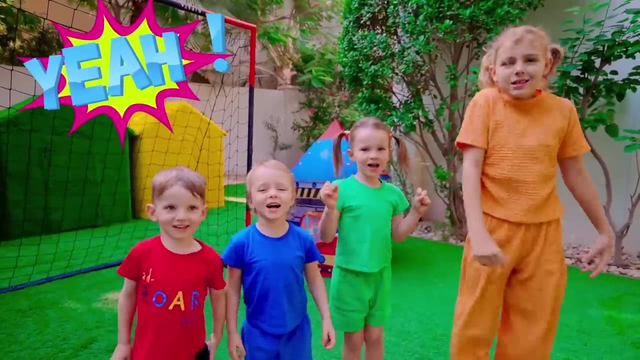 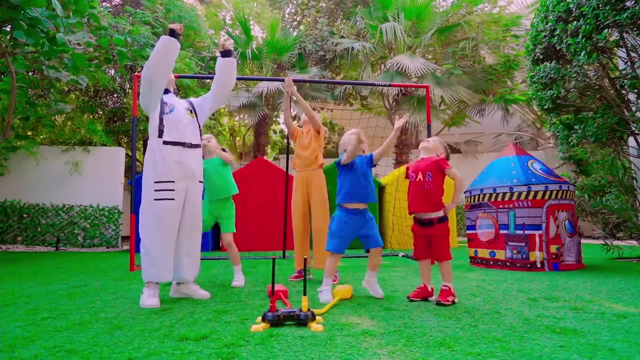 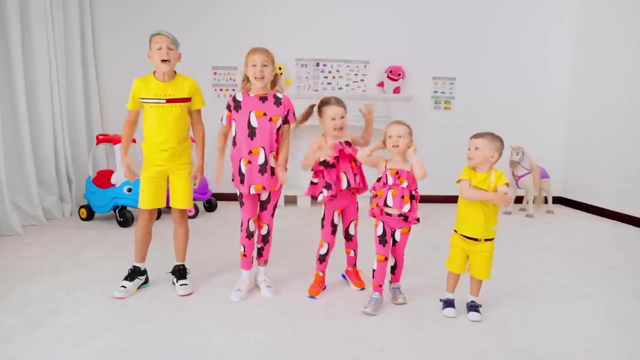 Today, we have learned a lot of interesting information about the solar system and the planets. Are you ready to launch your rockets to the space? Yeah, Woohoo, Let's go. Oh my gosh, Oh my God. This is wonderful. 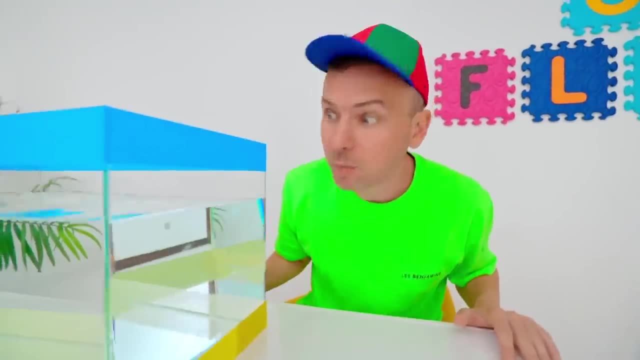 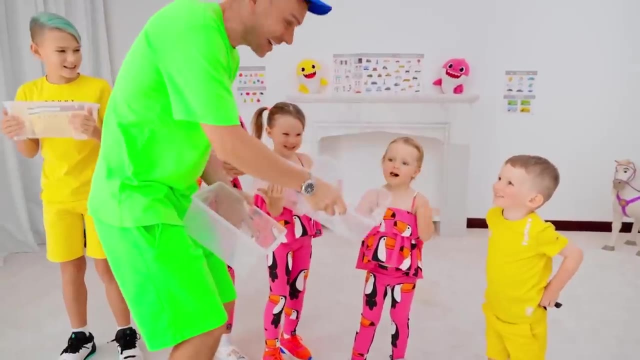 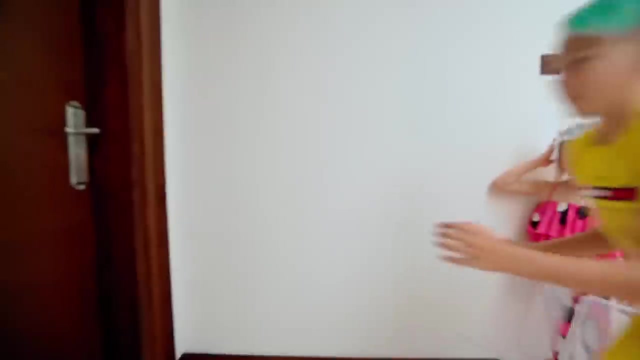 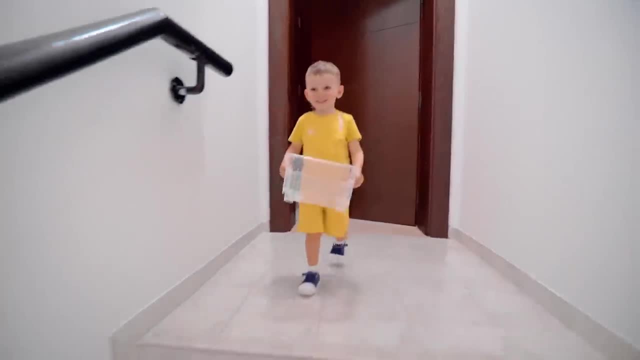 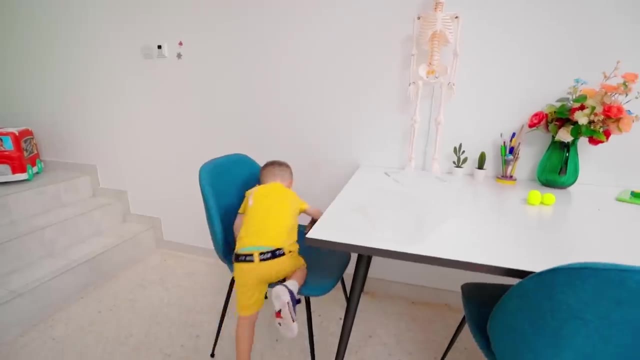 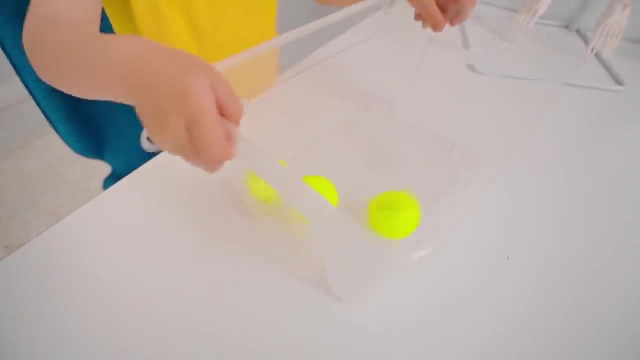 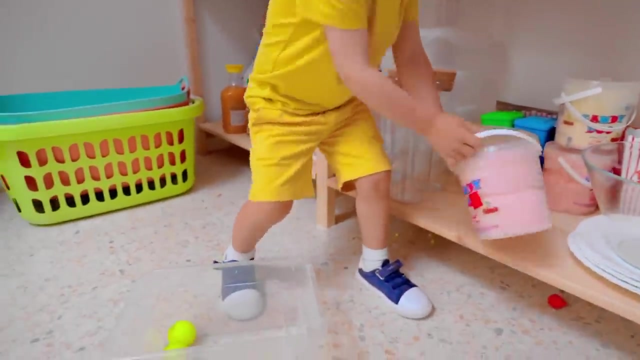 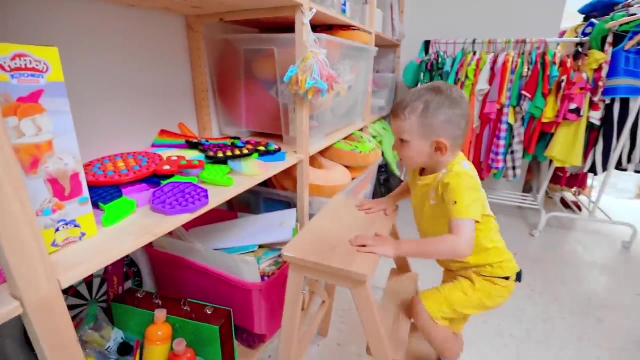 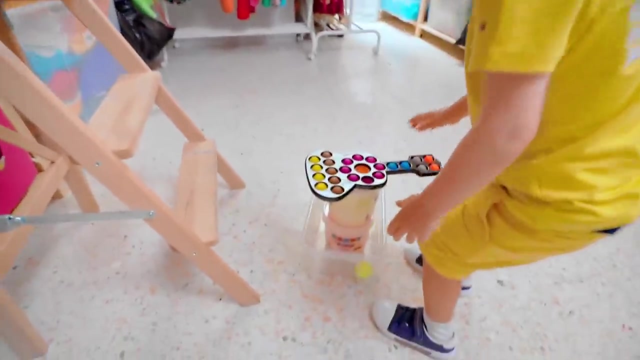 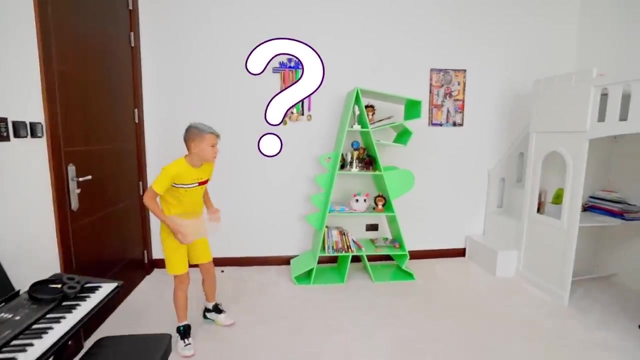 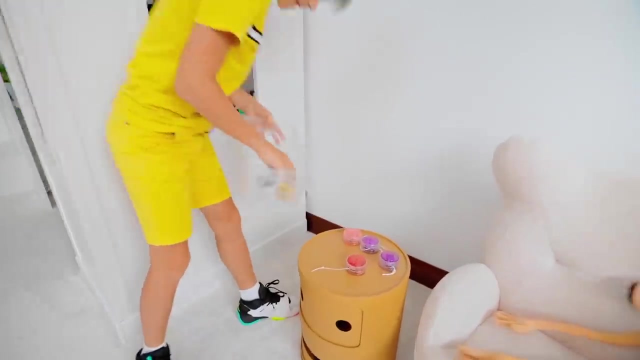 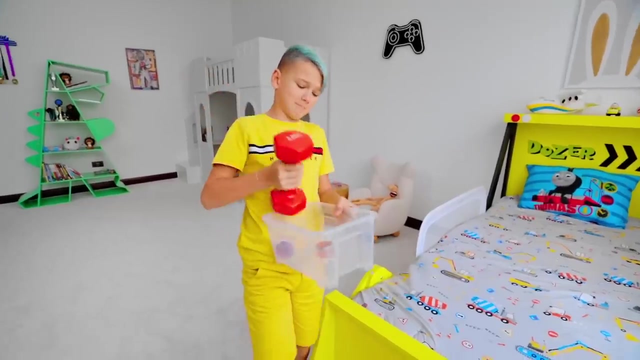 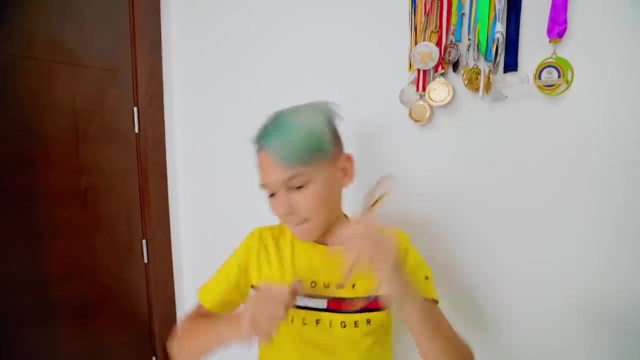 And here Yeah, Balls Cotton candy. Aha, Pop it, Aha, Peter, pop it, Aha. Hmm, what should I take? Yo-yo, Oh, dumbbell, Oh a medal, Yeah, Cactus. 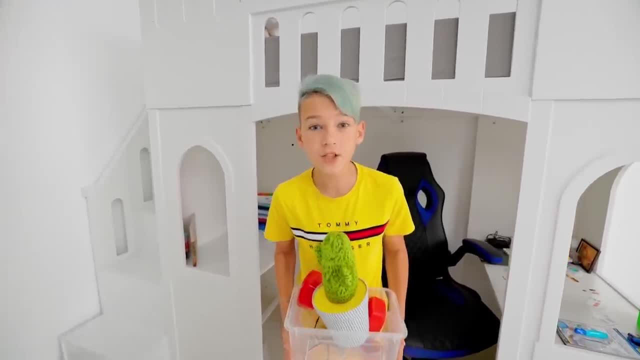 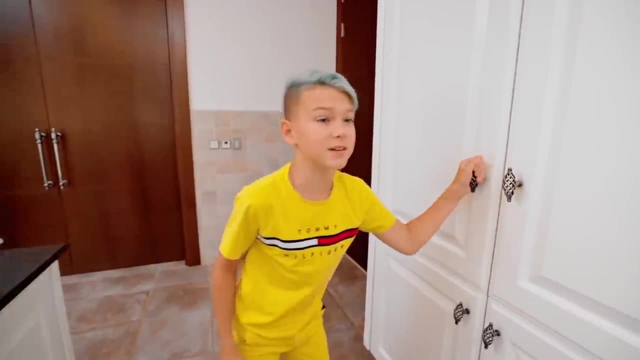 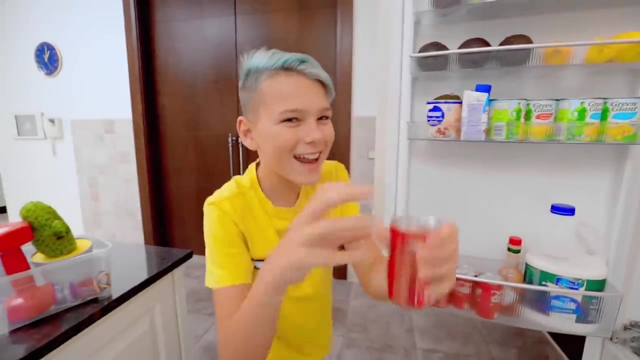 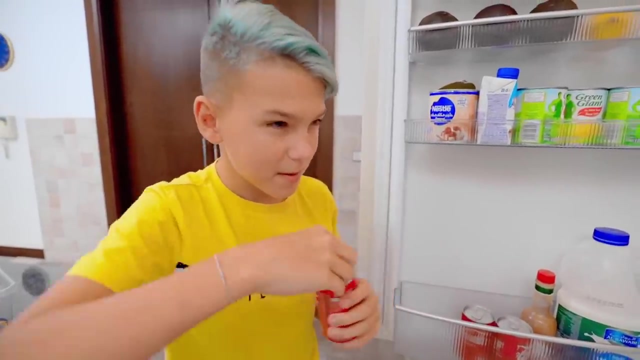 I think that's it for this room. Now let's see what is in the fridge. Fridge, Let's see what's there. Aha, Hmm, Oh, Coca-Cola, Hmm, Hmm, Let's check if it sinks or floats in here. 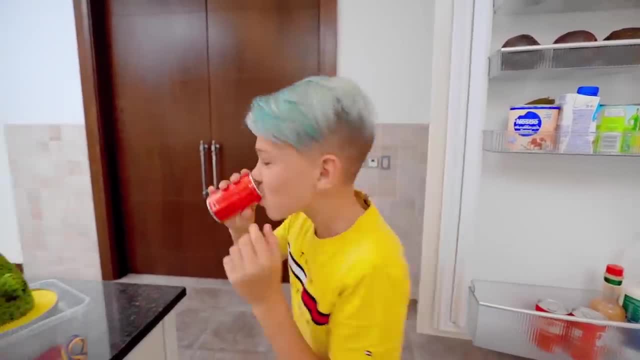 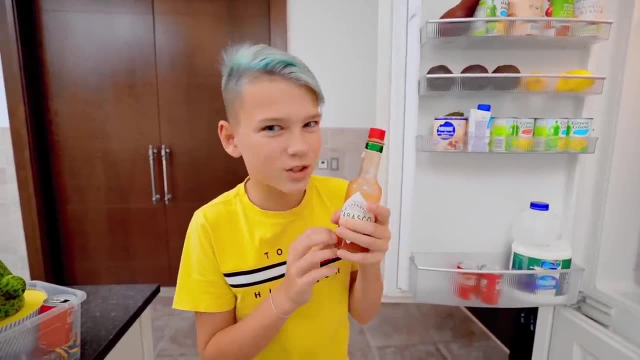 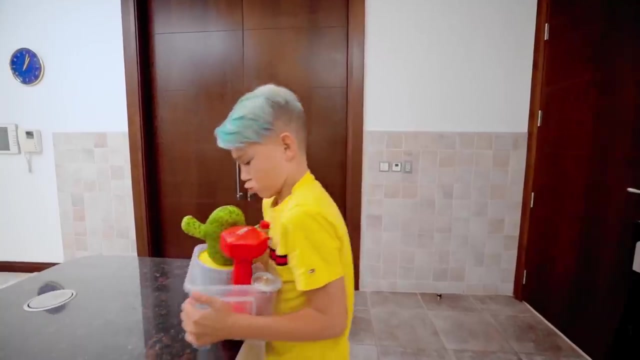 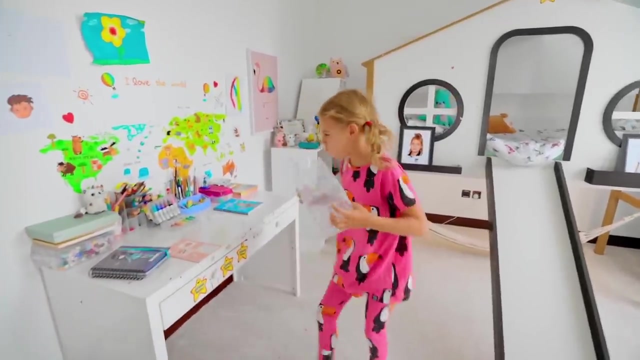 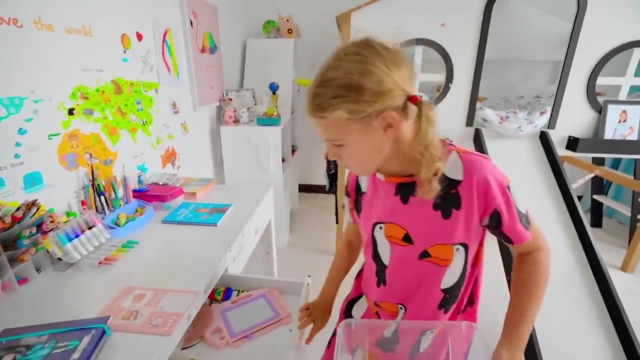 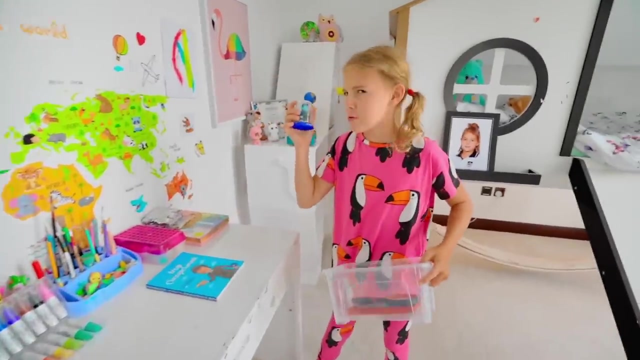 I think sink. Woohoohoo, Topasco, Have you tried it So spicy? Aha, Done, Let's go. Hmm, what should I take? Hmm, Hmm, nice pencil case, Magnifying lens. Hmm, Will it sink or float? 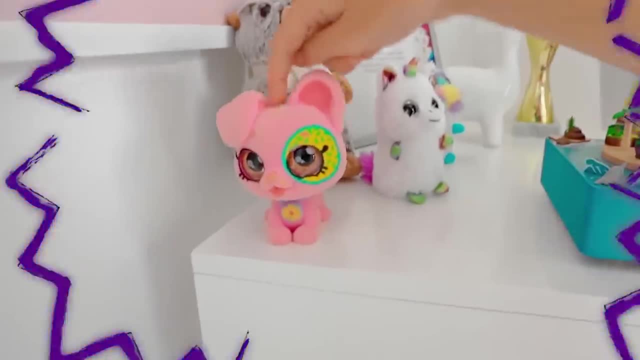 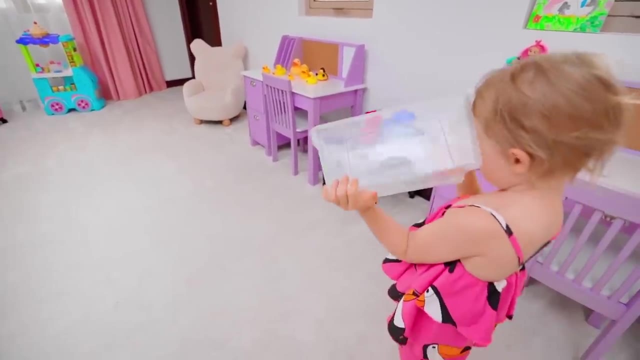 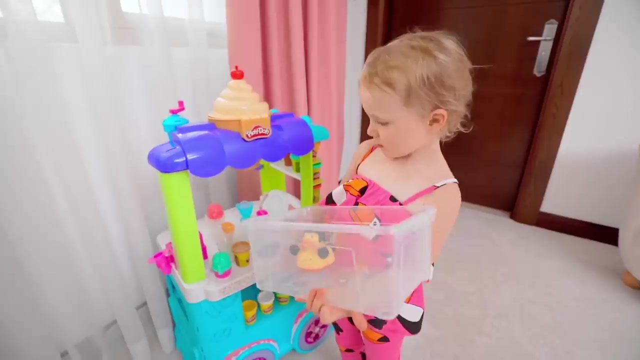 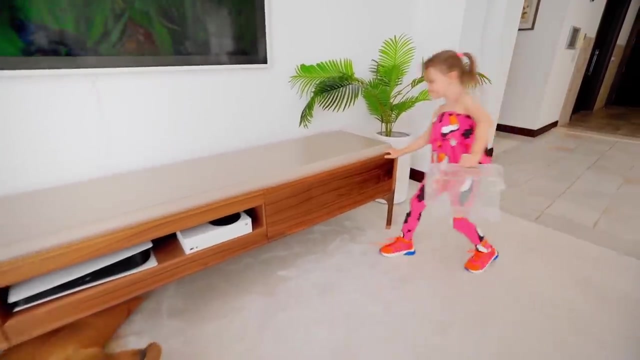 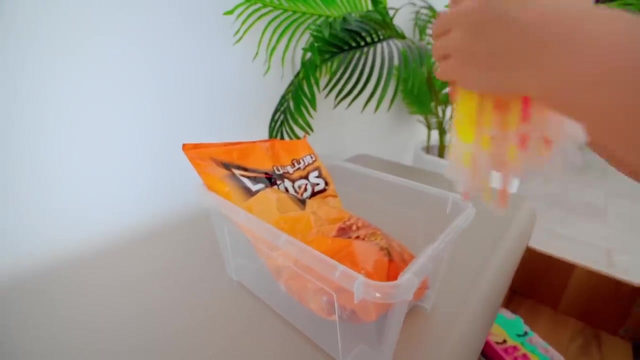 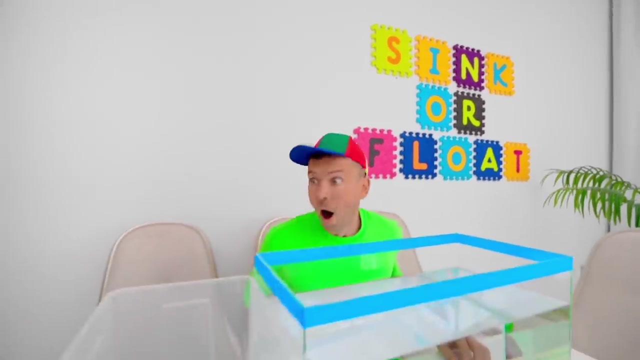 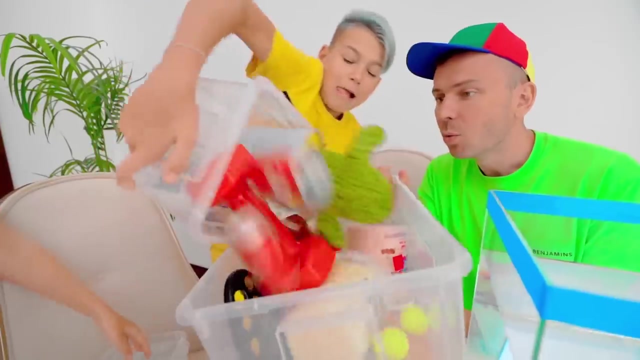 Hmm, Meow, Done Babs. Aha, I love play-doh. Aha, Hmm, Hmm, Aha, Yeah, Yeah, Yeah, Yeah, Yeah, Wow, Put them all in here, Wow, Wow, Alex. 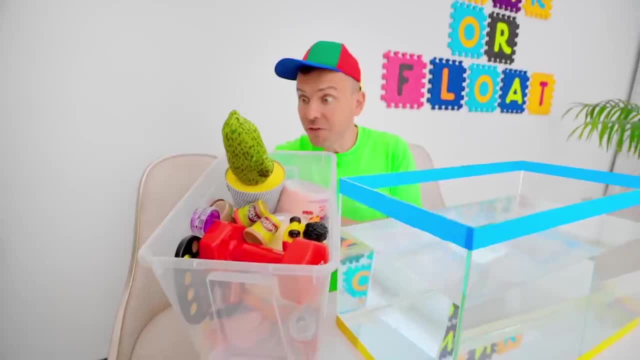 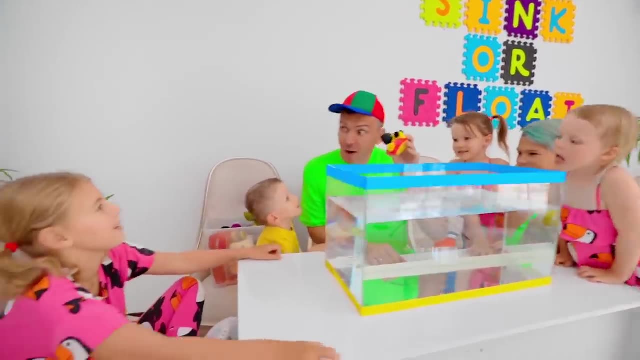 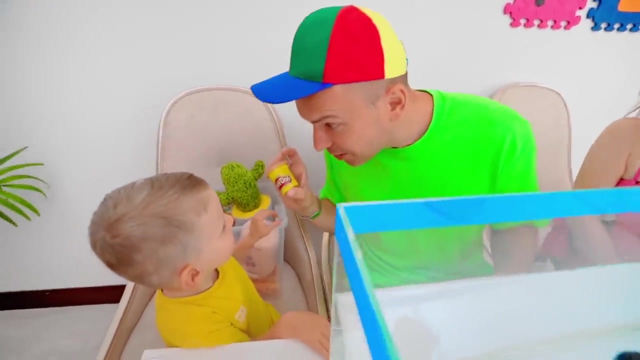 Wow, Wow, A lot of things. Let's see if they sink or float. Let's see if they sink or float. Maria, what do you think? Will it sink or float? Float, Wow, Float, Wow. Play-doh, What do you think? 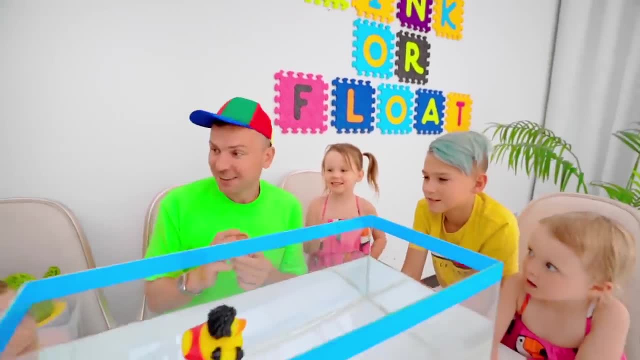 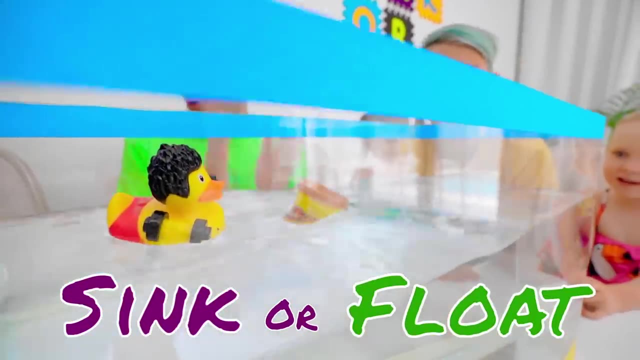 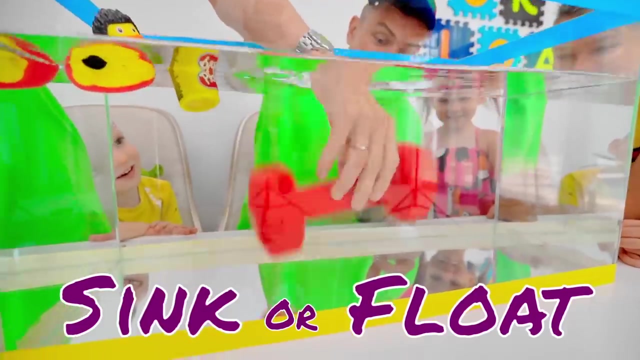 Will it sink or float? Sink, Float, Let's try. What do you think, Maria? Float, One, two, three, Wow, Float. What do you think? guys Sink, Are you sure? Of course, Dasha. what do you think? 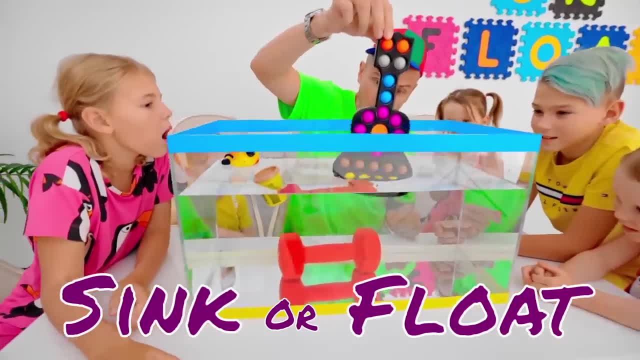 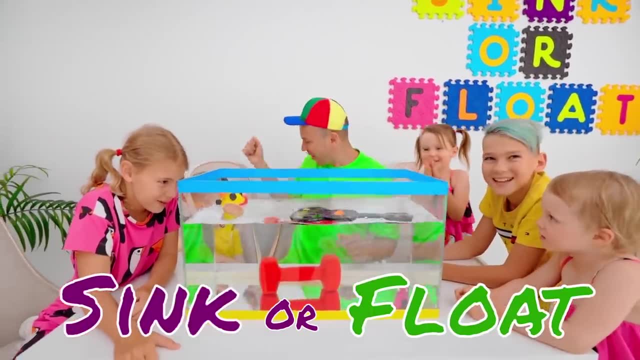 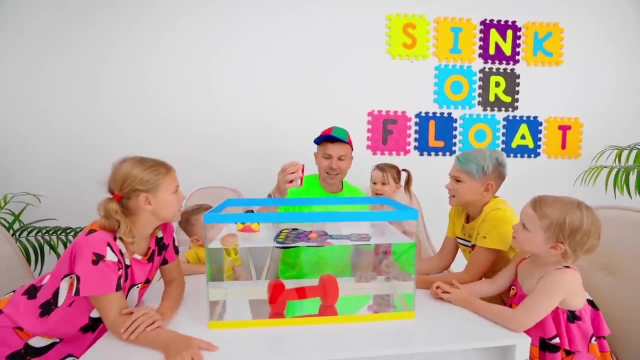 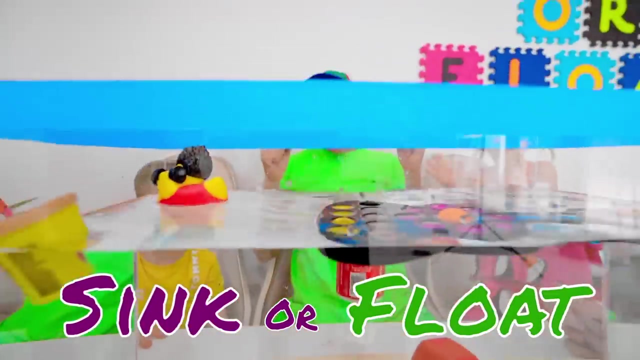 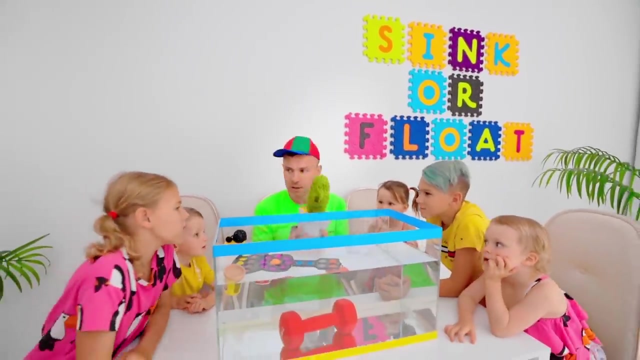 Sink or float Float, Sinks, Sink Float, Float A Coke, What do you think? Sink Float Float? Wow, Wow, Wow. It's heavy. What do you think? Sink, Sink Float, Sink Float. 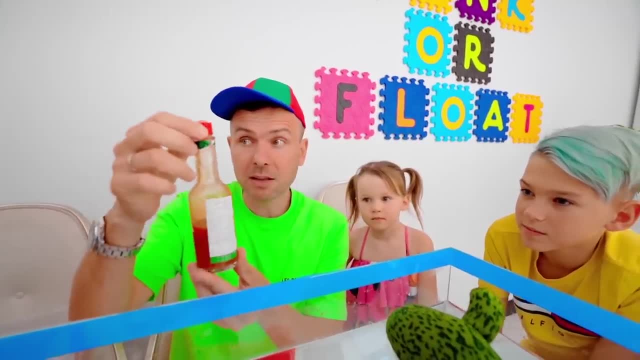 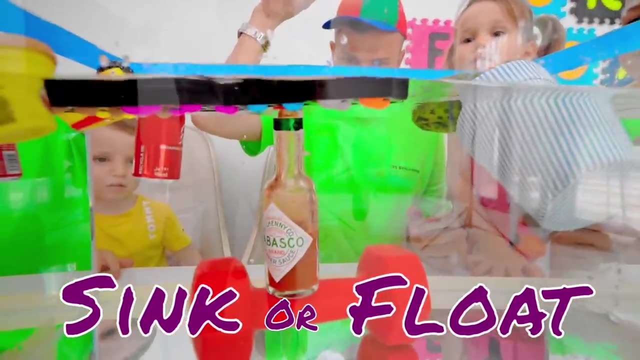 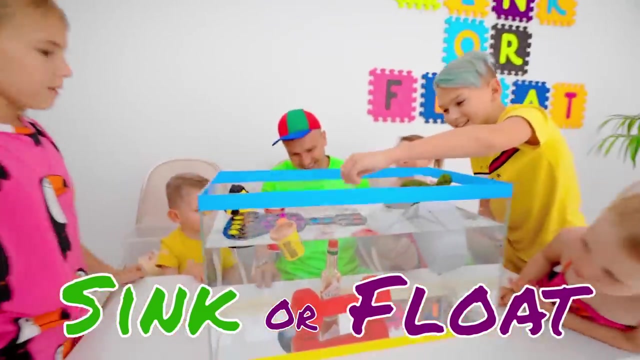 Wow, It's sauce, but the bottle is not full. What do you think? Sink, Float, Sink, Sink. It's not sink, It's not float, It's sink. Okay, what's next? What do you think, guys? 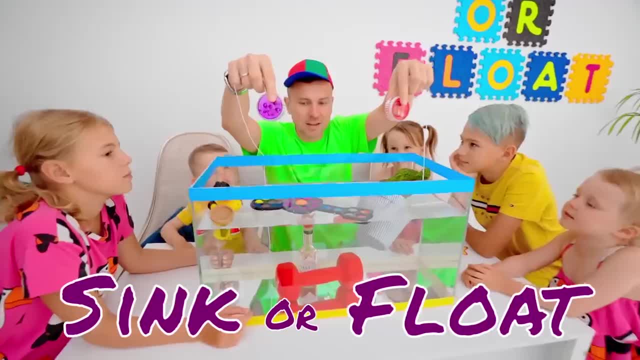 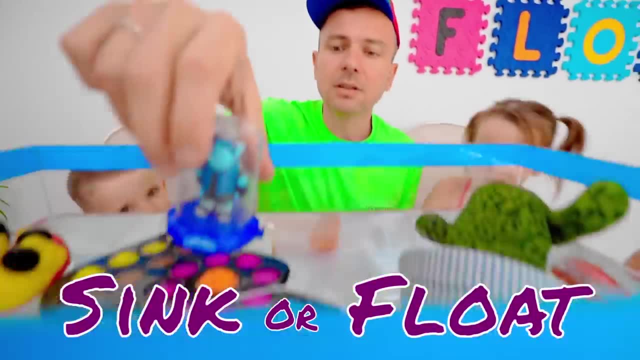 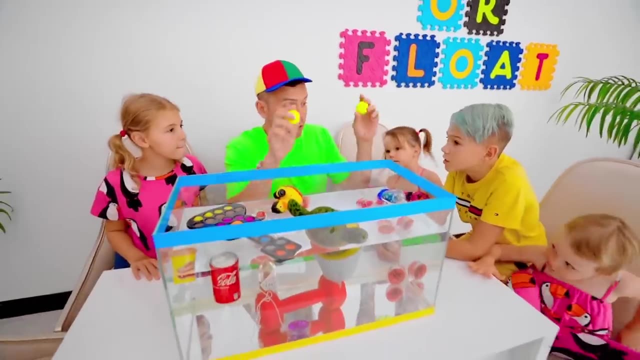 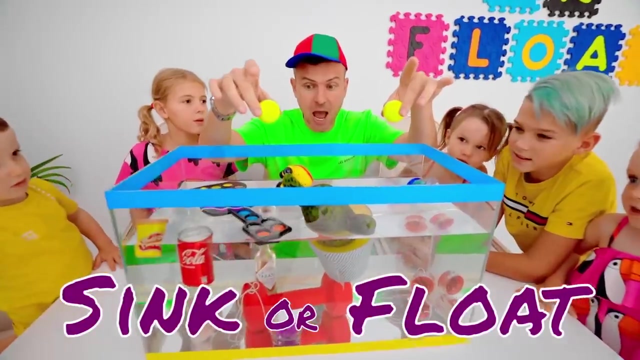 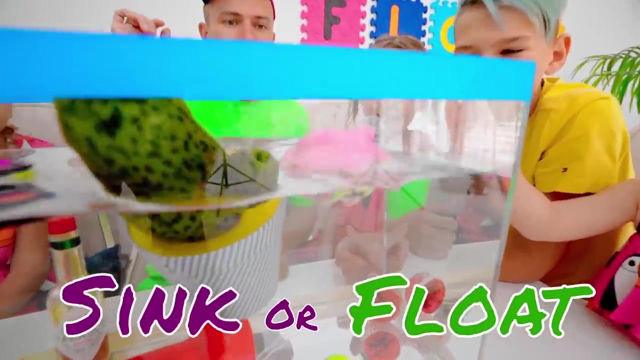 Float Float, Definitely float. Yeah, because it's plastic. What Float? Float Float? A lot of air. Dasha, what do you think? Sink or float? Sink Float, Sink, Yes, Sink Float. 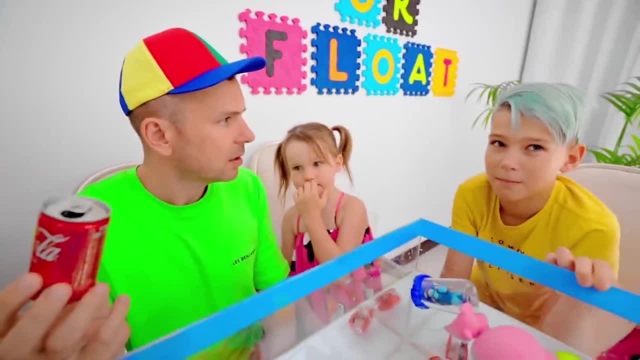 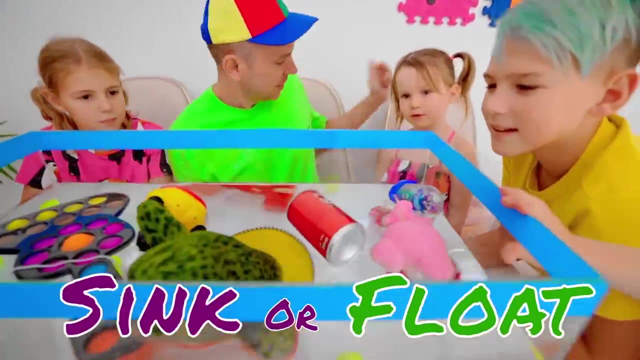 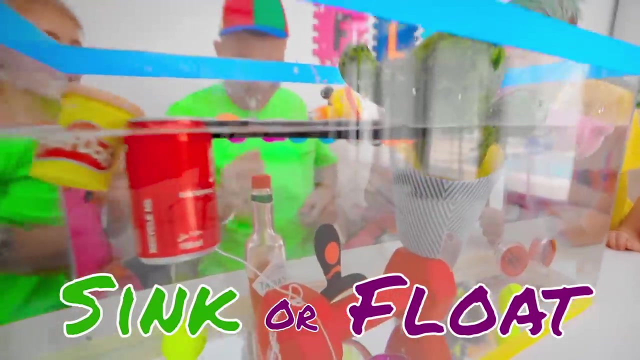 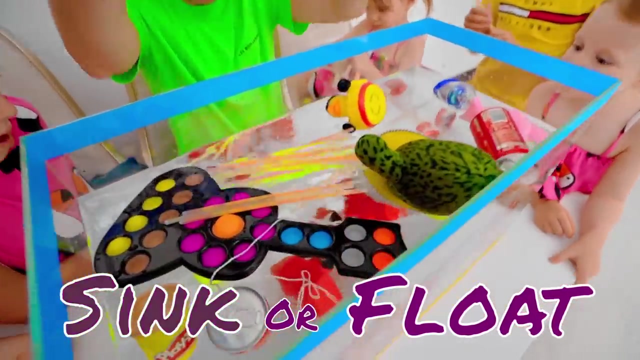 A can, An empty can. Why is it empty? Because Vanya drank it. Float. and then sink Float and then sink Float- Magnifying lens Float- Sink Sink Float, Sink Caramba, Sink Sink. 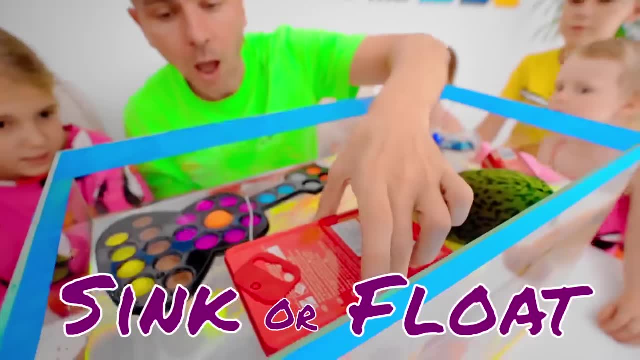 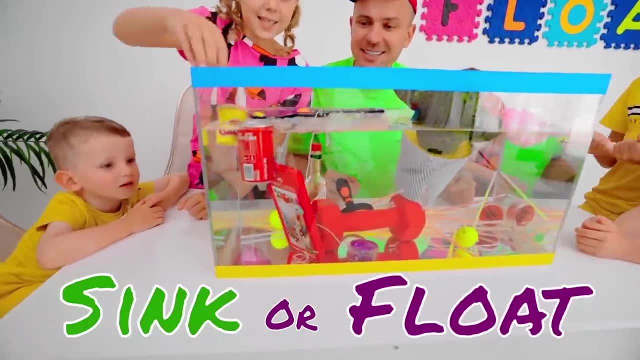 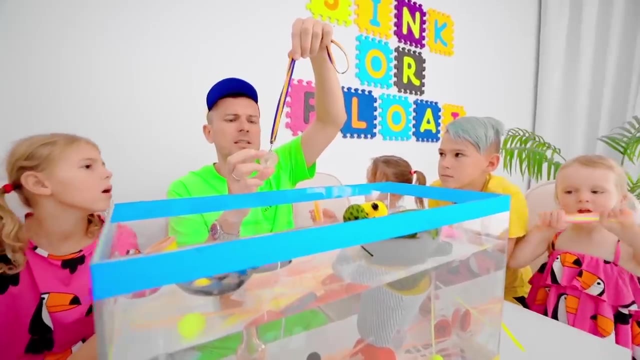 Float. What is that? Pencil case? Float, Float, Float. If you put like this Sink, What do we have? A medal? Who's this? Vanya Vanya, The best singer in the church? No, it's my football medal. 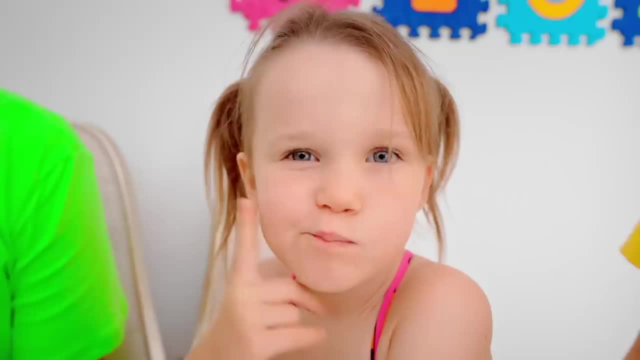 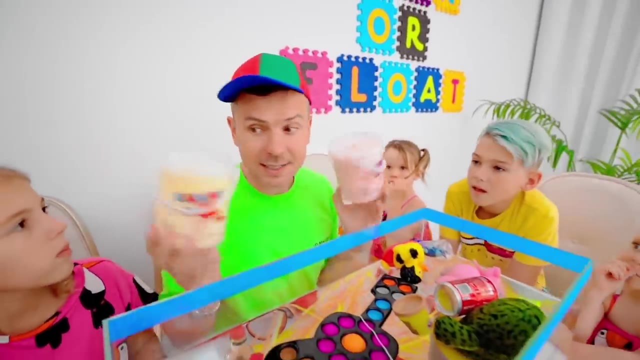 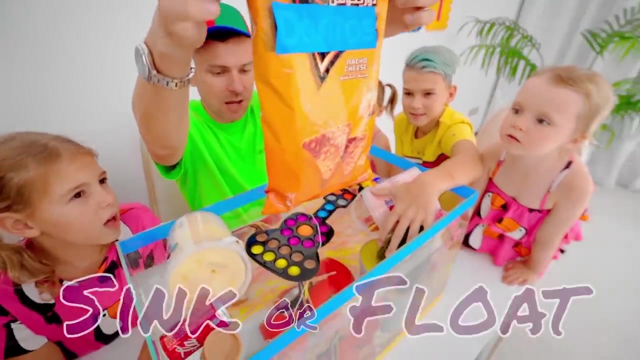 Okay, what do you think guys? Sink, Sink, Of course. Wow, Cotton candy, Two pieces. What do you think? Float, Float, Float, Float. Let's try One, two, three Float. I have another idea. 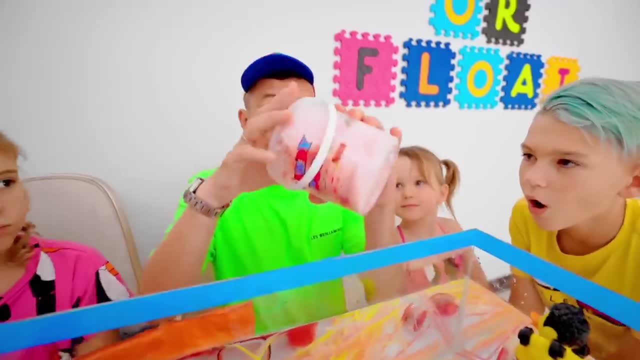 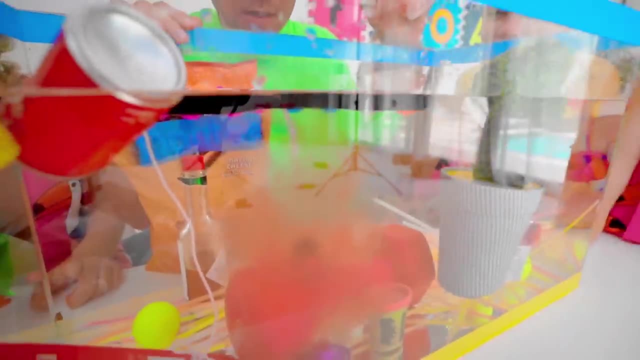 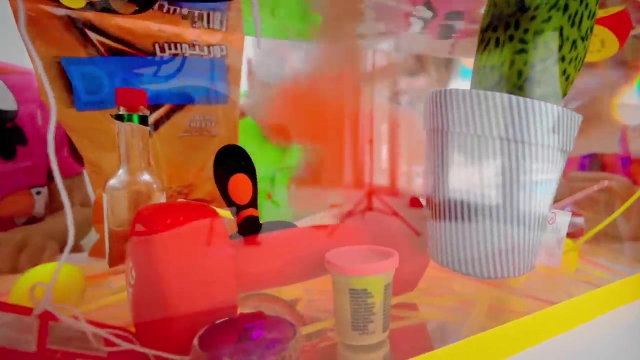 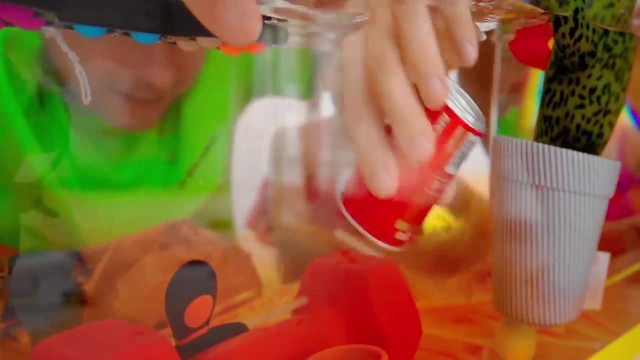 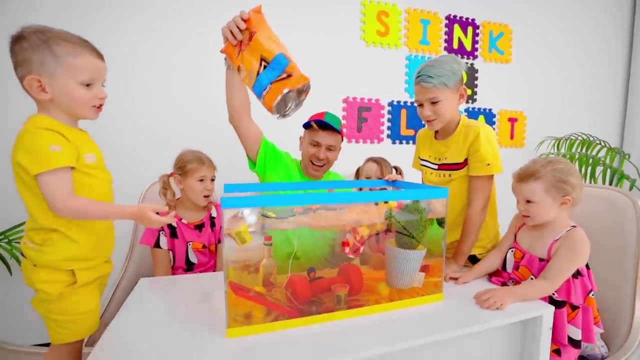 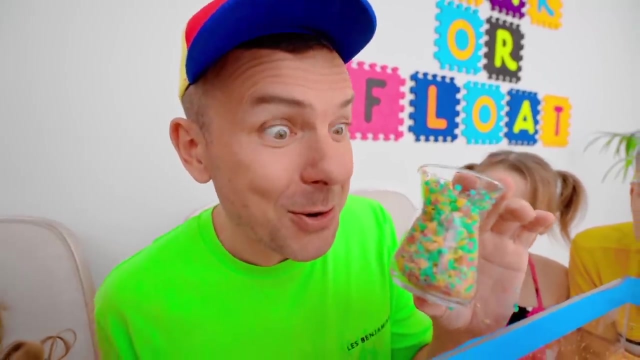 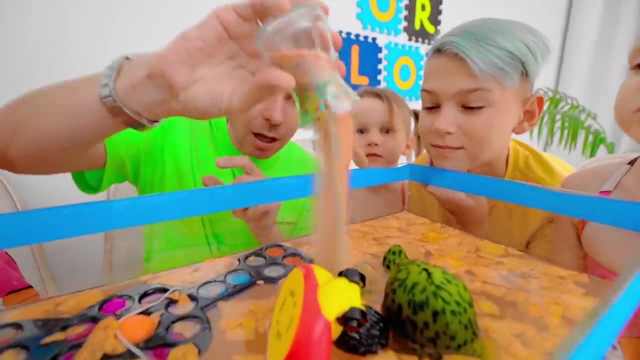 Now let's open everything we can: Cotton candy- It disappeared. Can I Wow, Woohoo, Wow Cheese, Did you like it? Yes, But I've got something interesting for you: Jelly, crack, Quack, Shhh. 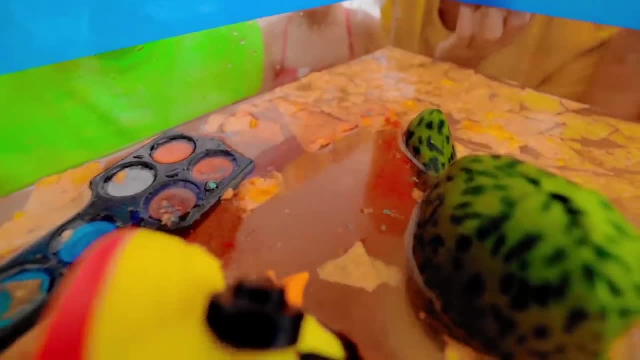 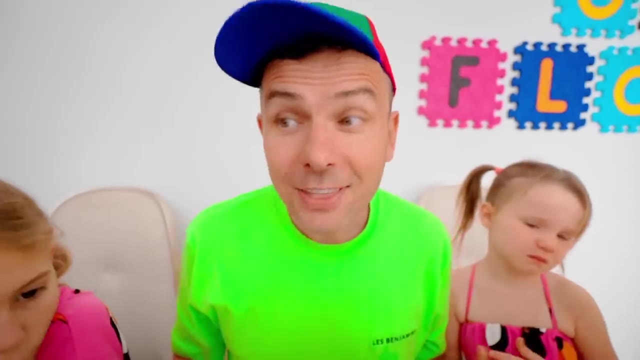 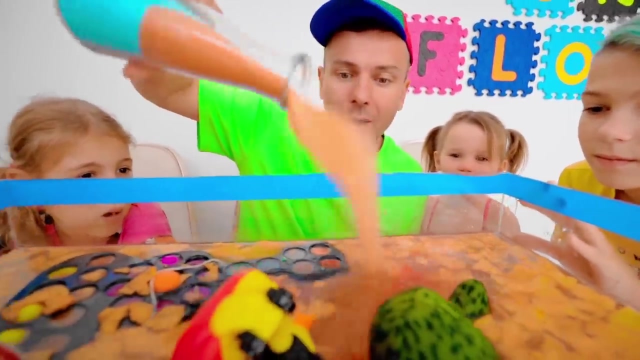 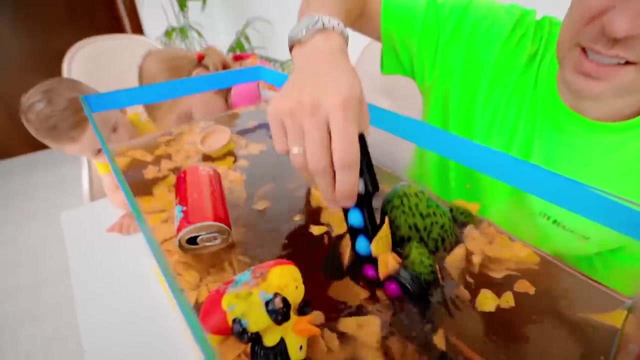 Hear that? Yeah, It's blowing. Yeah, And the last but not the least, the jelly bar Ready. Yeah, One, two, three go. Woohoo, Yeah, Hahaha, Yeah, It looks and smells like grandma's soup. 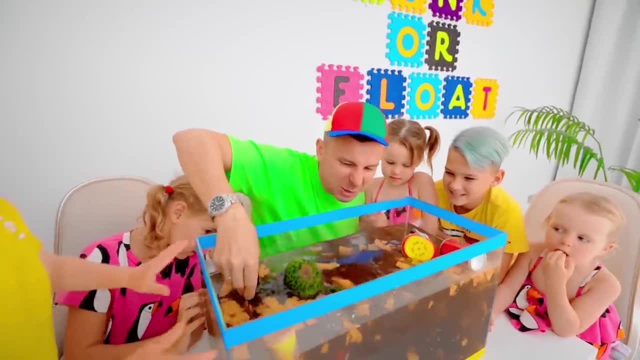 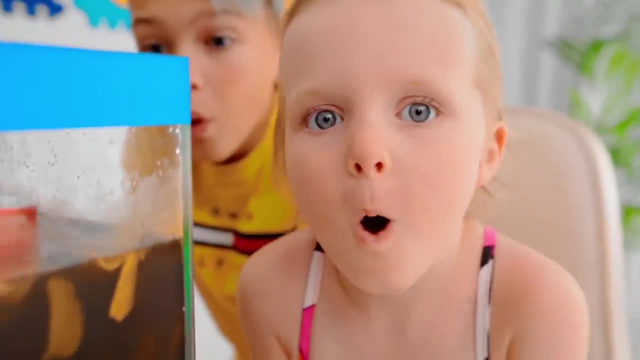 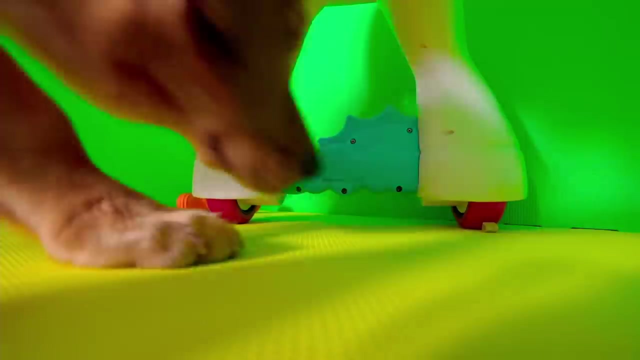 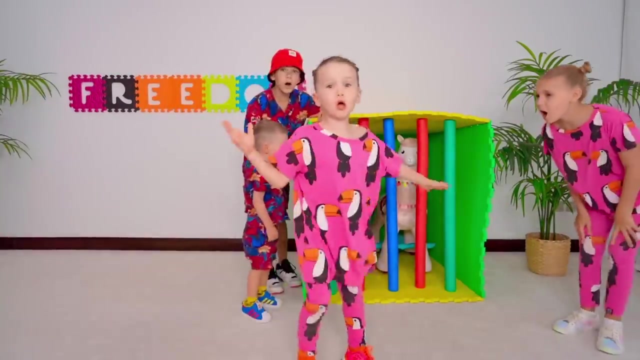 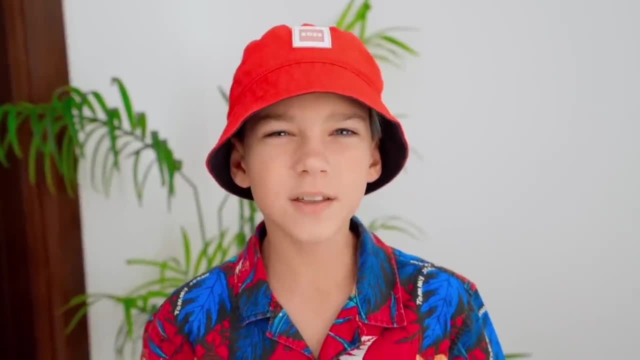 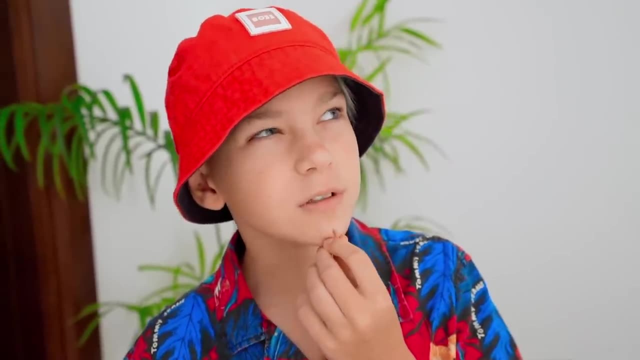 What should we do? Oh, I see that there are missing letters over there. Oh, I see that there are missing letters over there. Maybe we have to find them to free Luke. Maybe we have to find them to free Luke. But how can we do it? 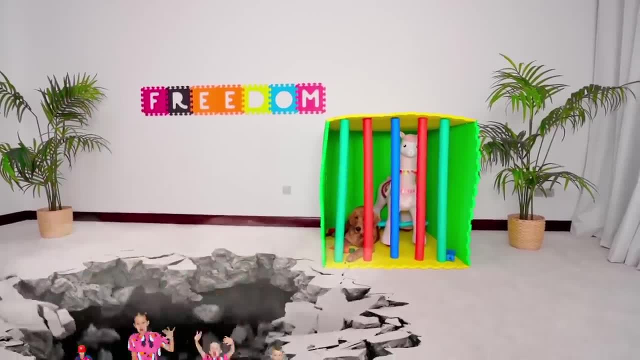 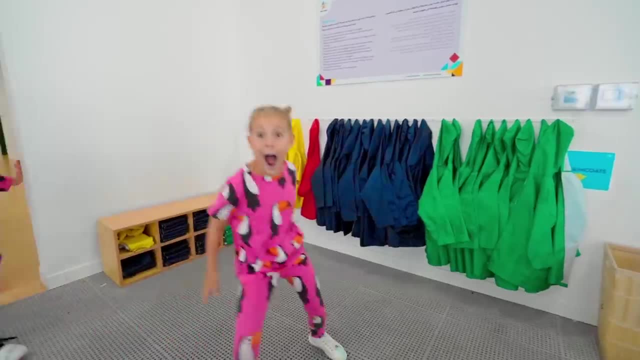 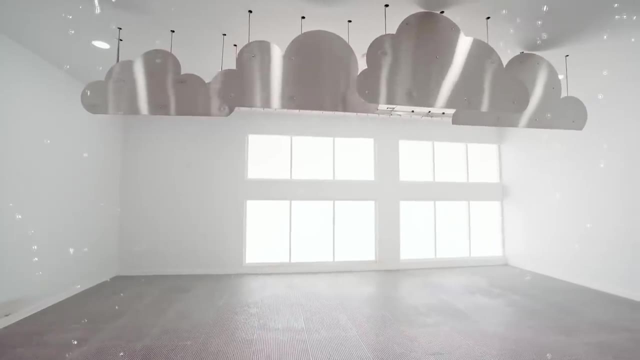 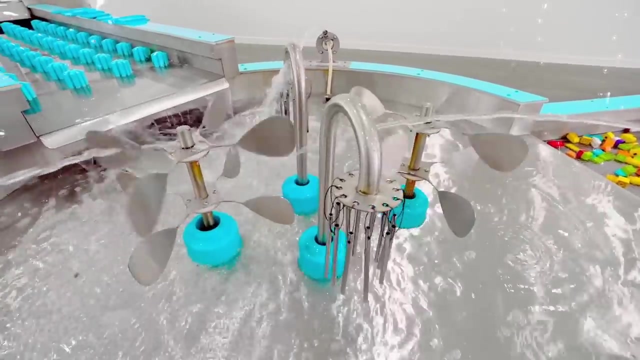 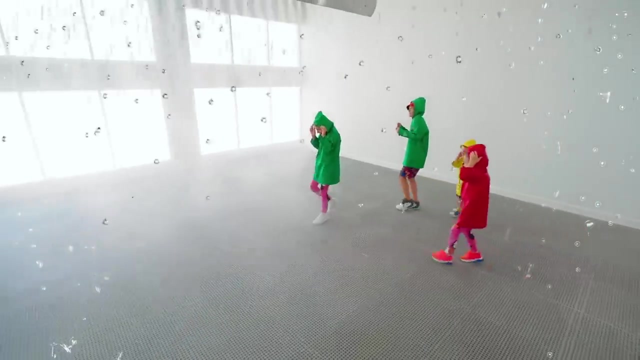 Is this a challenge? We need to save Luke. We need to save Luke, Woohoo, Wow, Oh yes, Wow, Wow, Wow, Oh yes, Woohoo, Oops, Oh, yo, yo, yo yo. 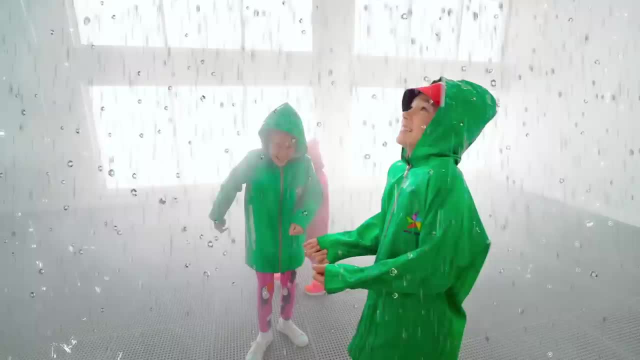 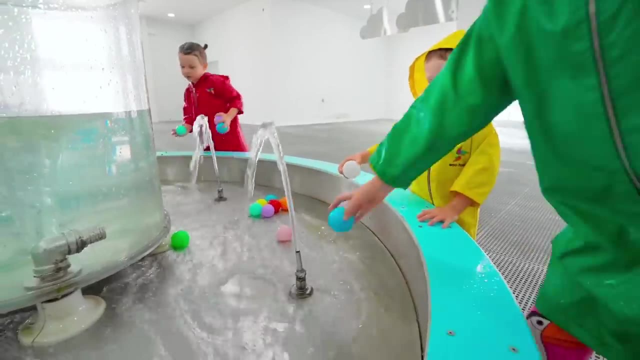 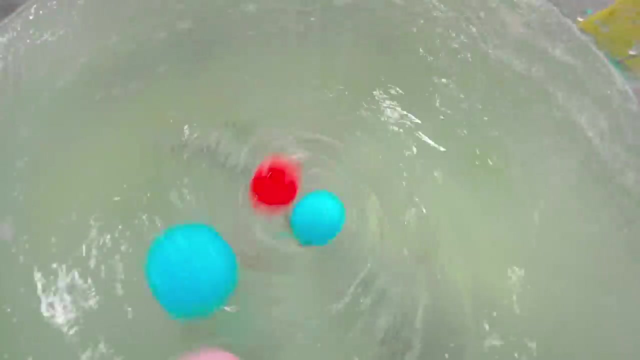 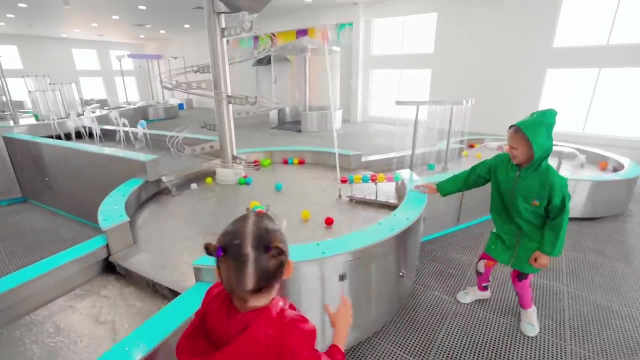 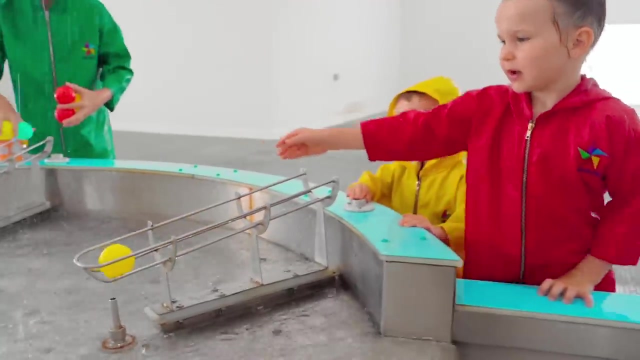 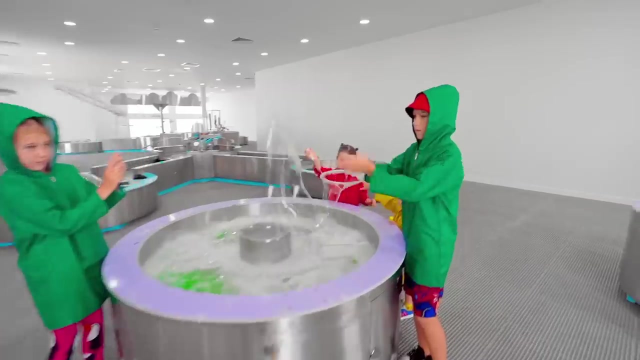 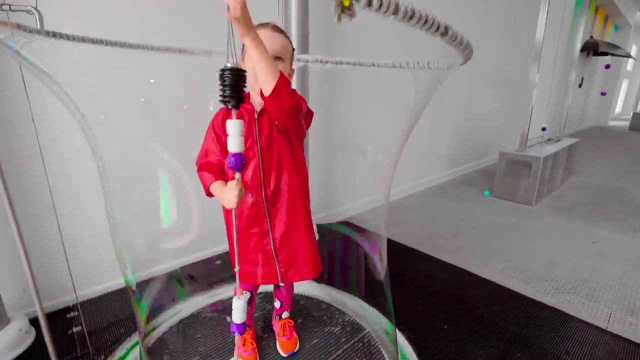 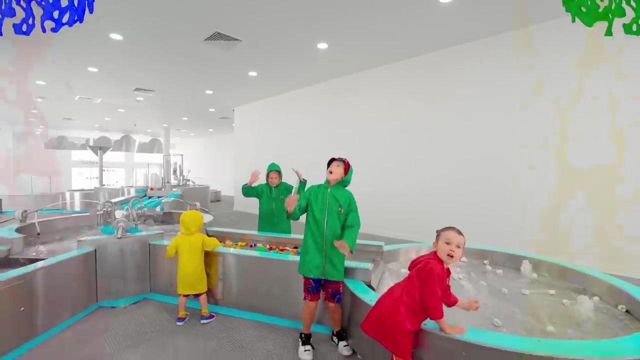 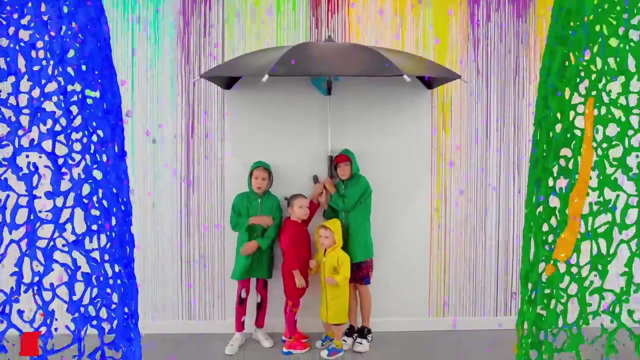 Hey, Where is Landon? A-ha, A-ha, A-ha. I will try to get it in the center. Wow, Wow, Wow, Excellent, Wow, It's all fun, but where is the ladder Ladder. 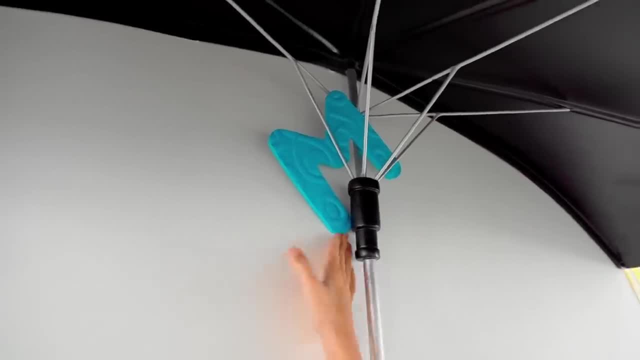 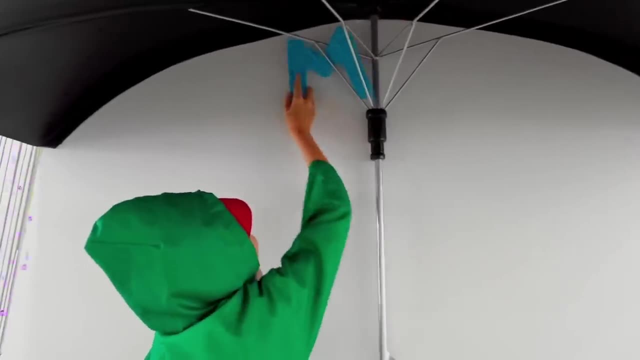 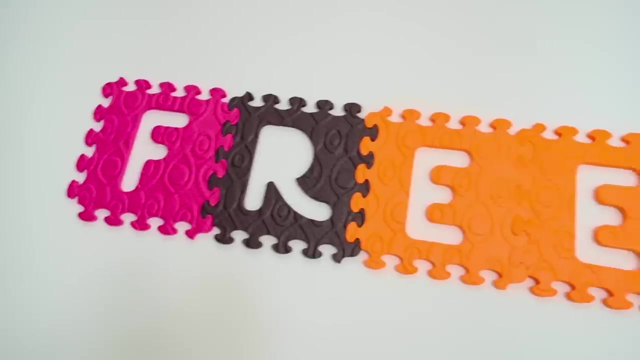 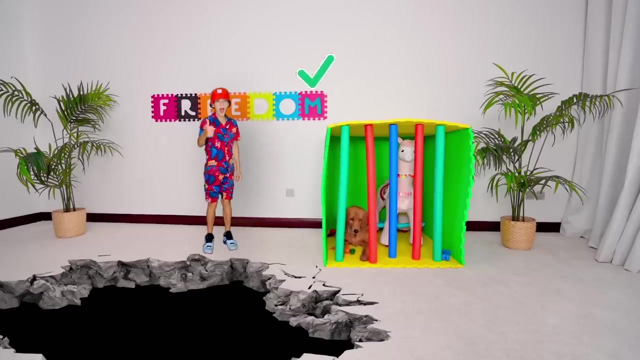 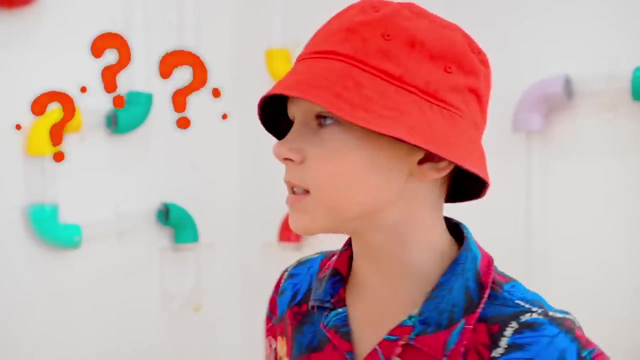 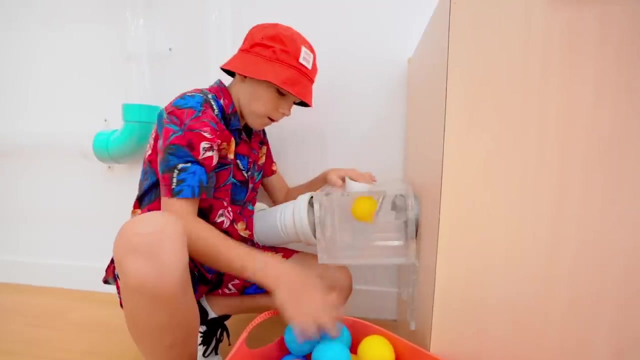 Oh no, I have an idea. M Awesome, M Woohoo, Wow, Wow, Wow. What is this? Where is the ladder? Hmm, Idea, Cool, Cool, Cool, Uh-huh, Woohoo. 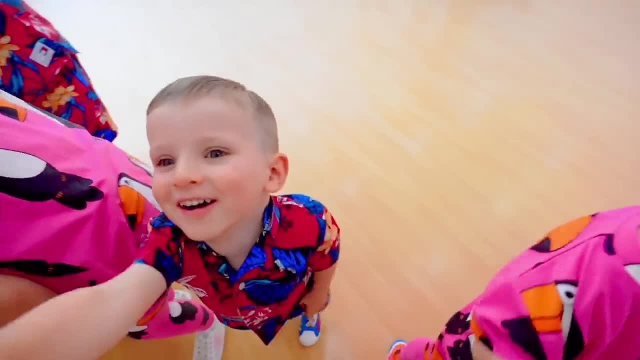 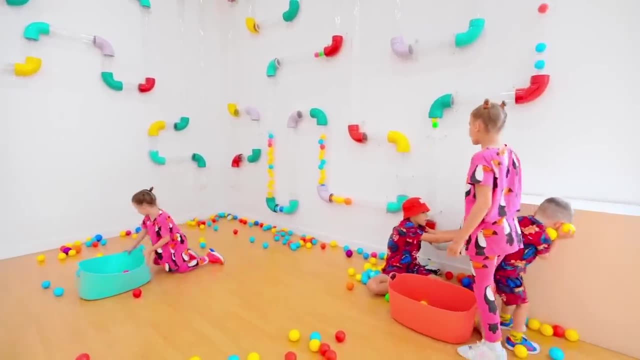 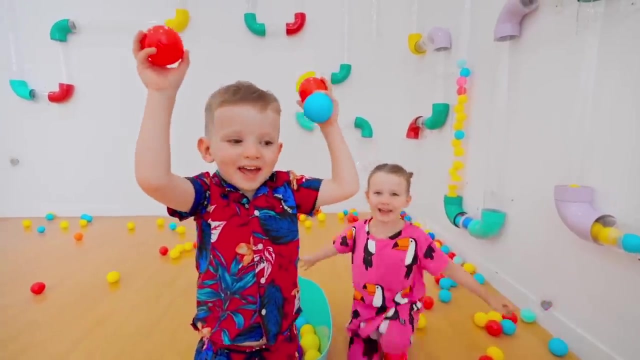 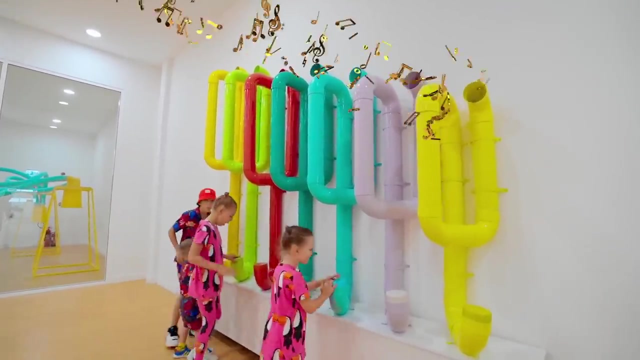 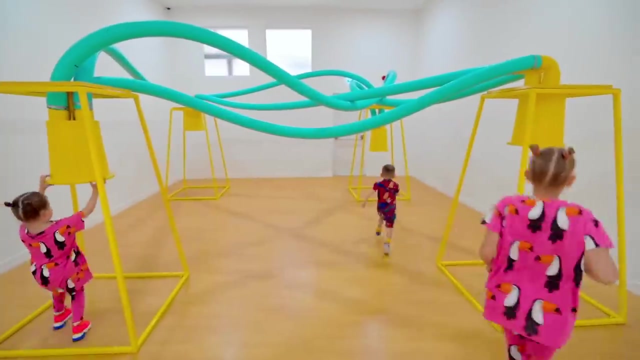 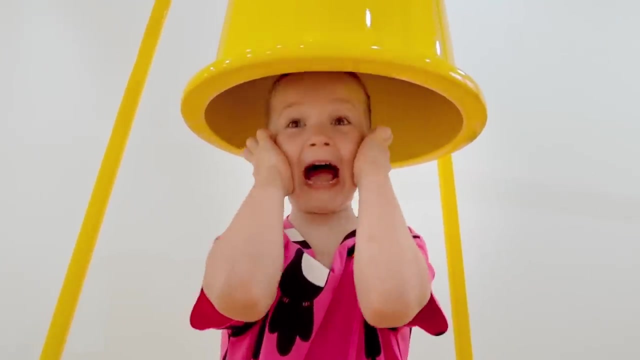 Wow, No, Woohoo, Woo, Woohoo. I found the ladder guys. Yay, I found the ladder M. That's it. G M N. Yay, G Woo Us, Hello, hello, hello. 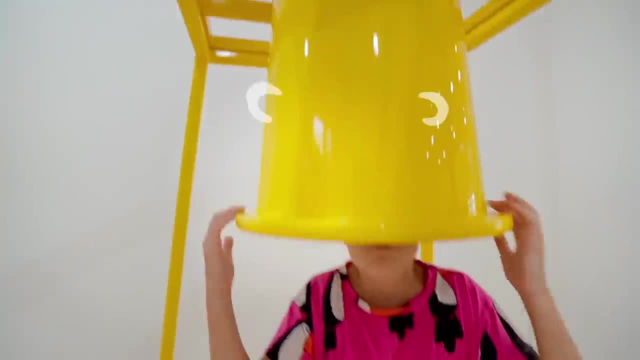 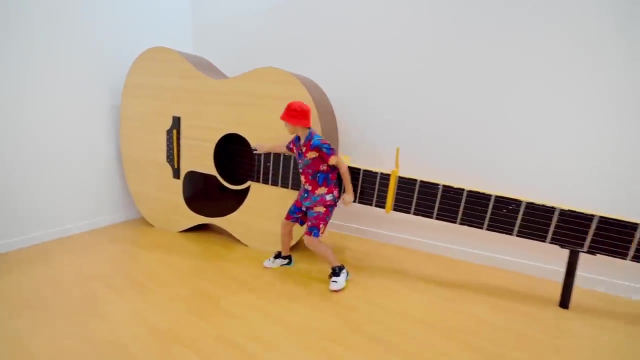 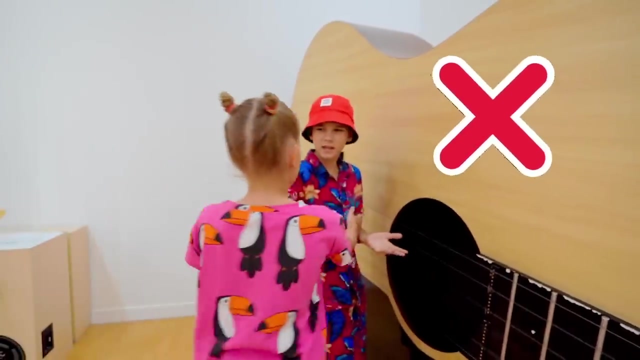 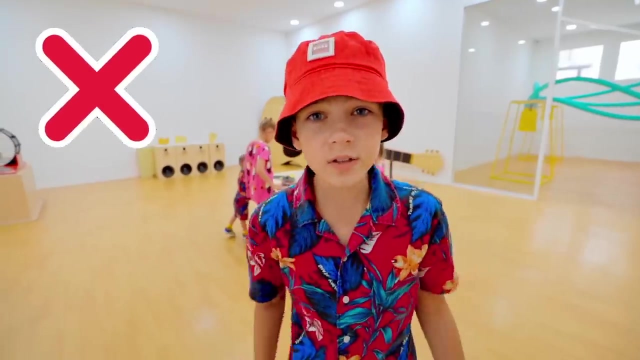 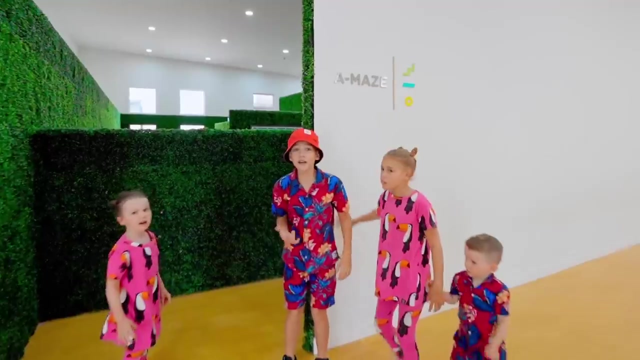 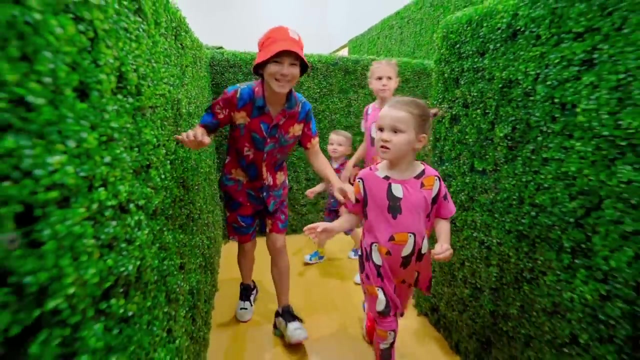 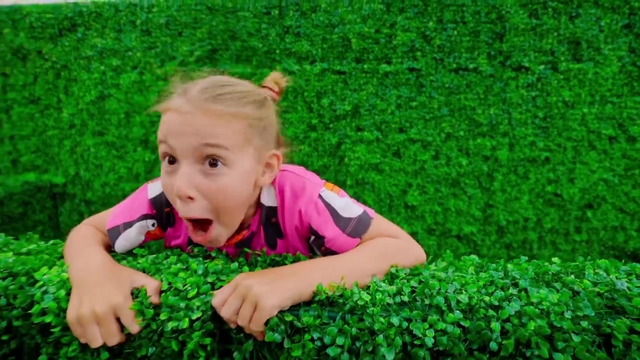 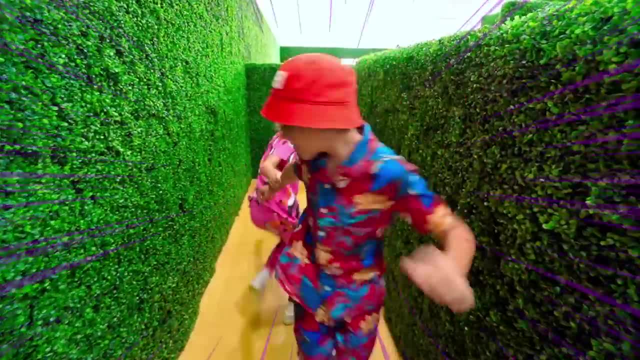 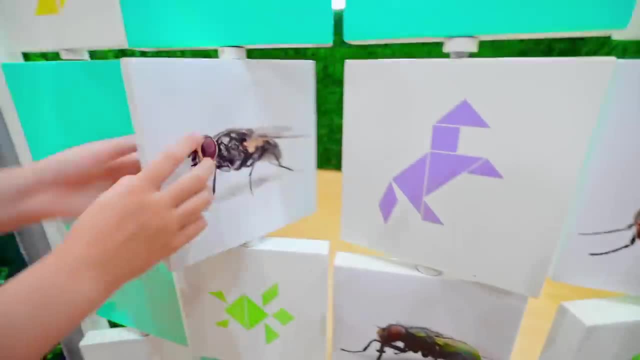 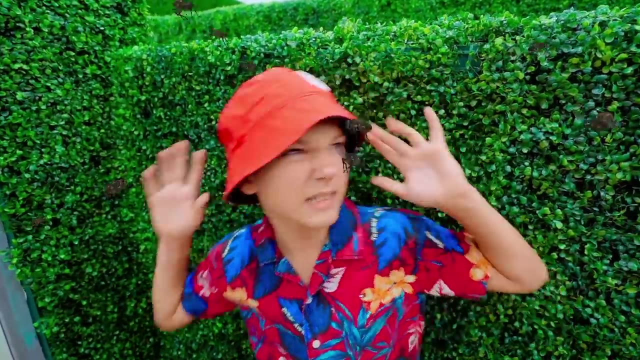 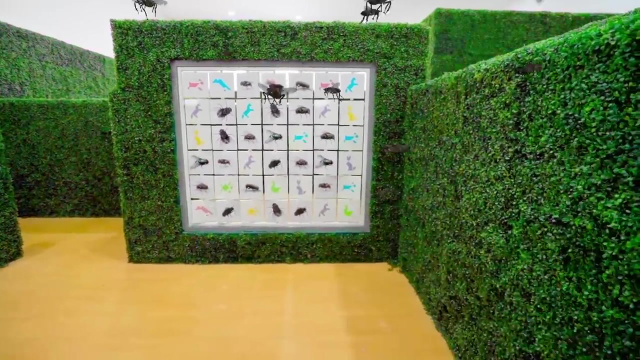 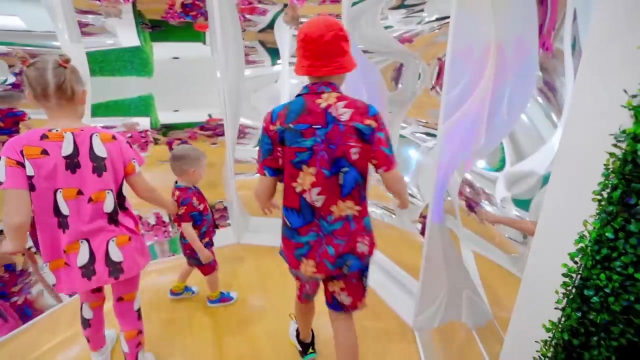 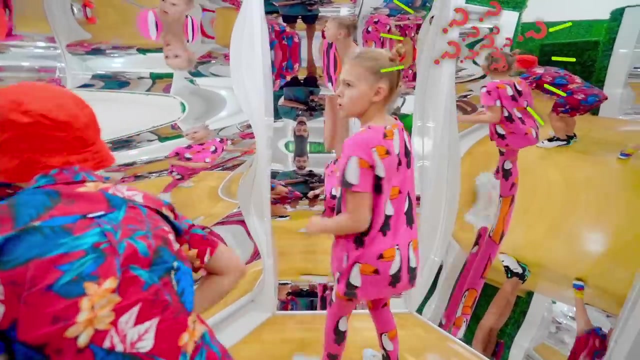 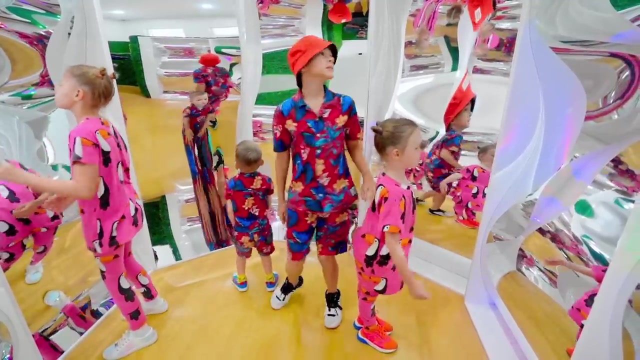 I can see a lantern. Let's go, Oops, Wow, Maybe a lantern is here. Wow, Oops. Why so many flags Fly, Go, go, go, Wow, Hey, Oh no, Where's the exit? Hey. 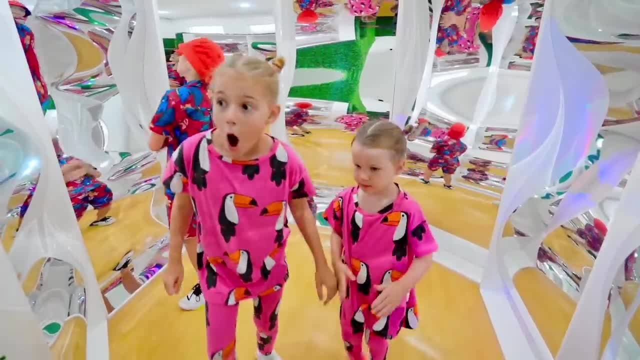 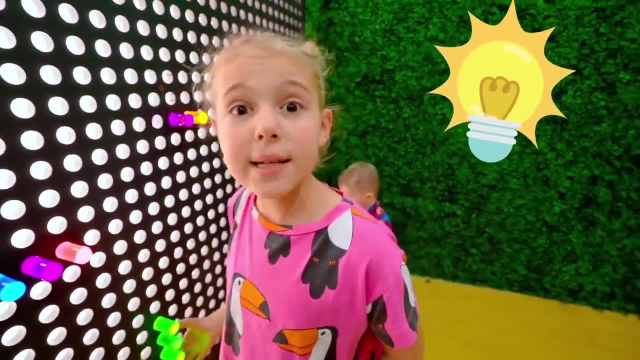 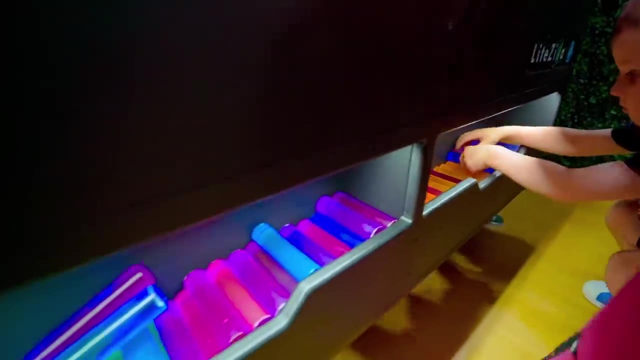 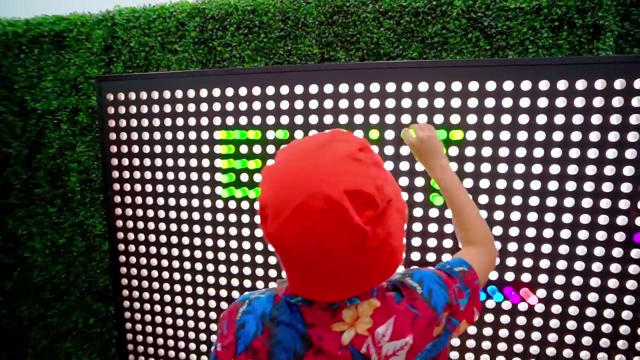 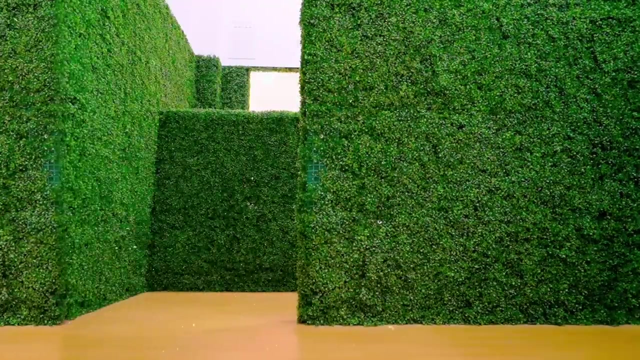 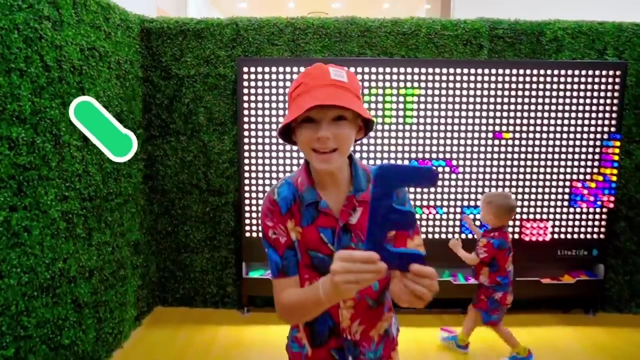 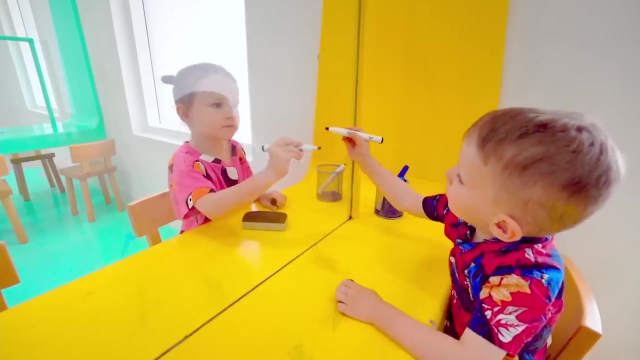 Hey, Oh yes, Wow, I have an idea. Let's write exit. I have an idea We can escape from here. Oh yes, Awesome, Wow, it's really easy. E E, E, E E Fantastic. 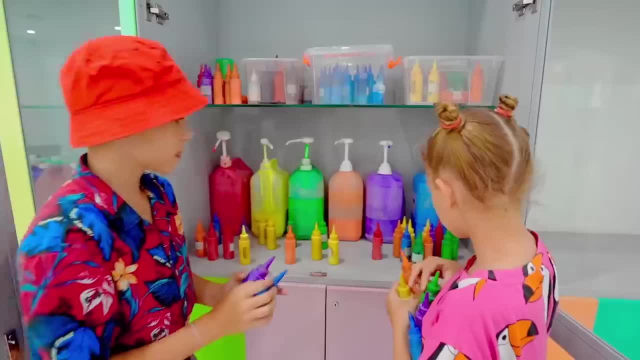 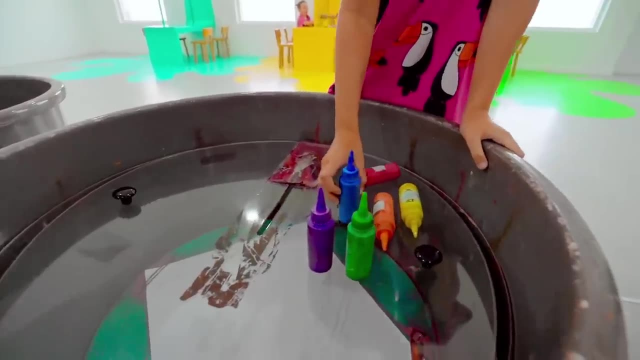 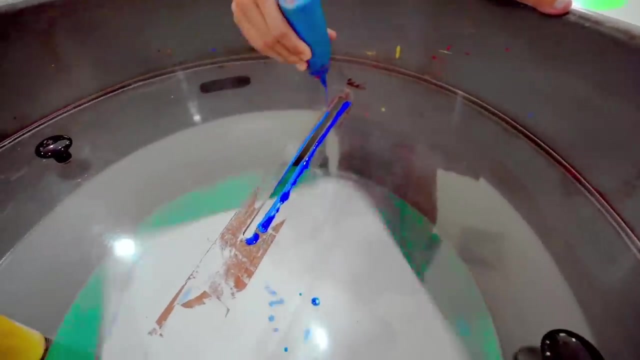 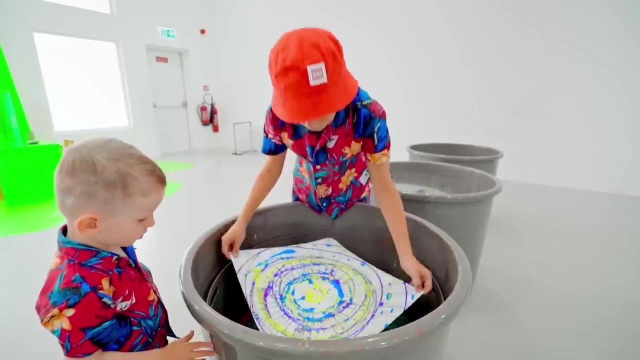 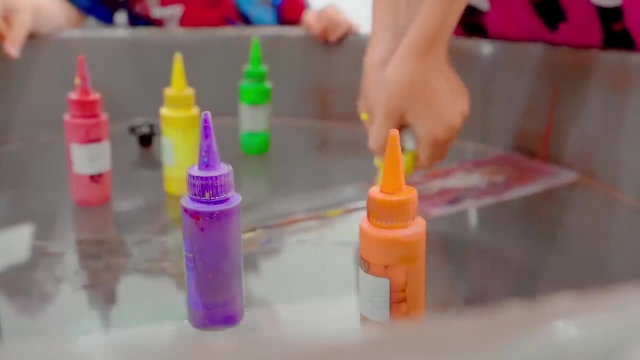 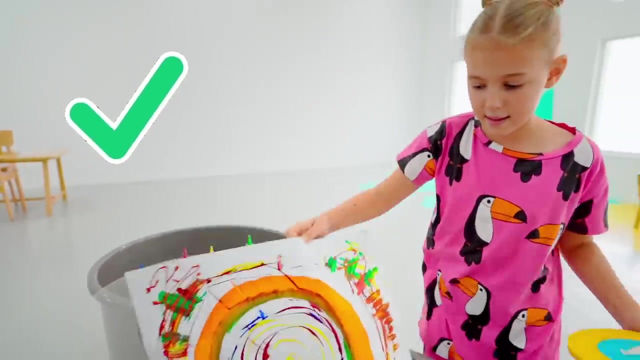 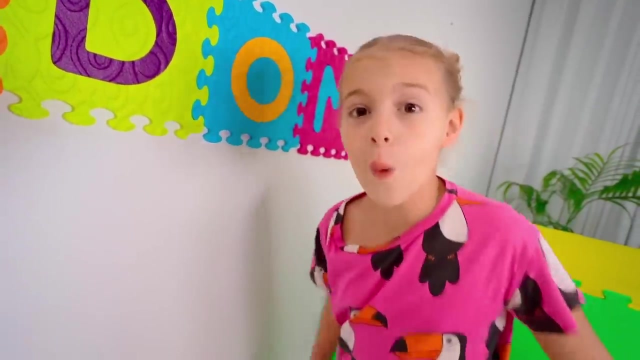 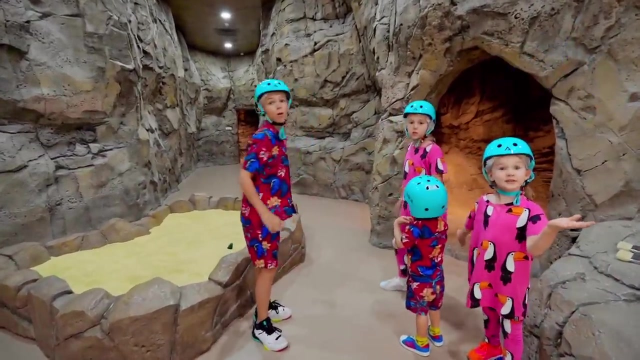 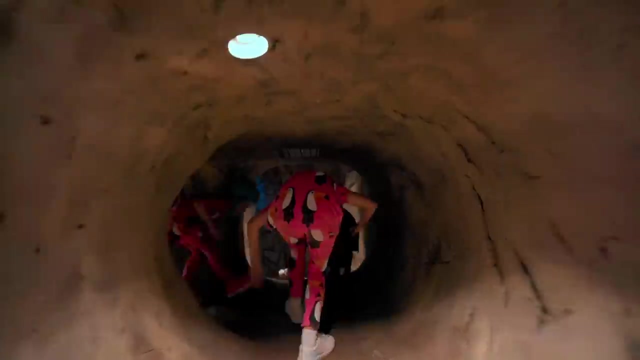 Wow, We will paint with this. We will paint with this. Yahoo, Wow, Excellent, Fantastic. I have an O, Awesome, O, O, O. Where's lantern? Let's find it. Oh, yes, Wow, Go, go go. 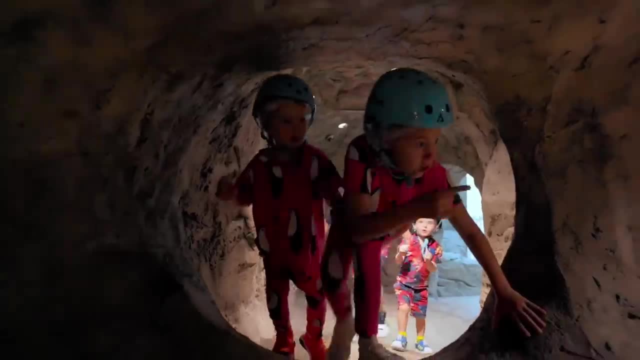 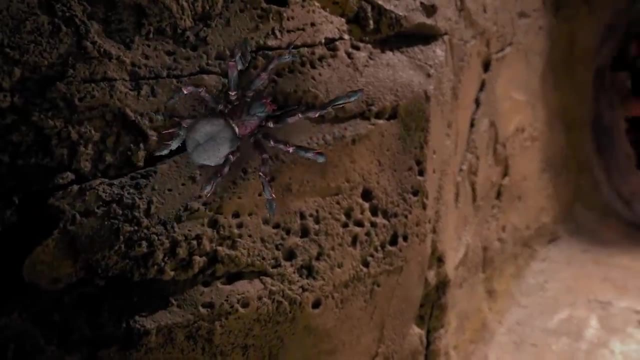 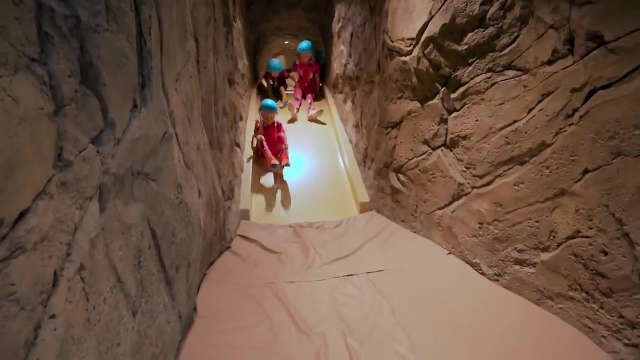 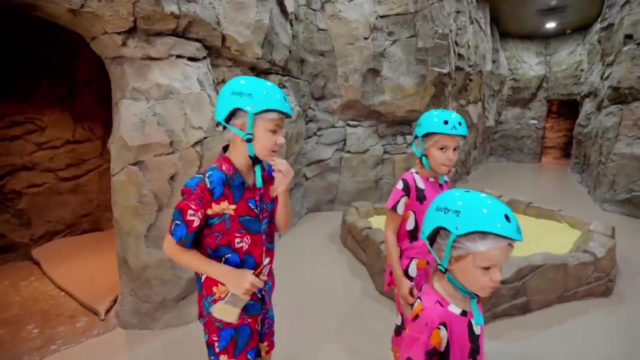 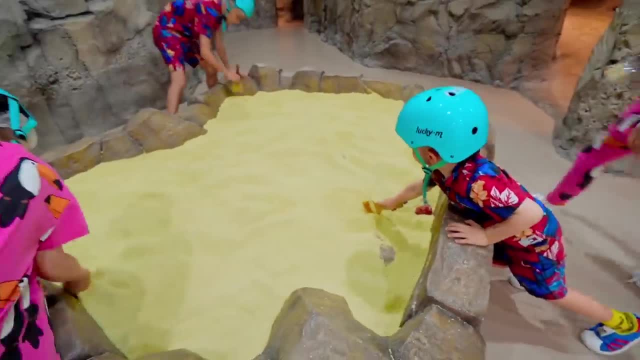 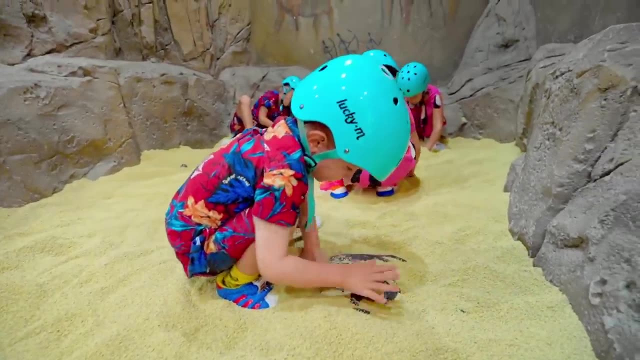 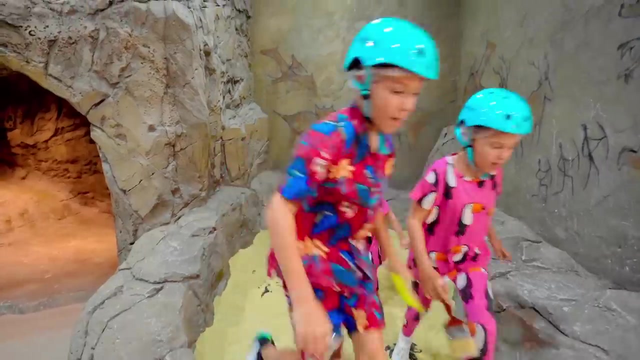 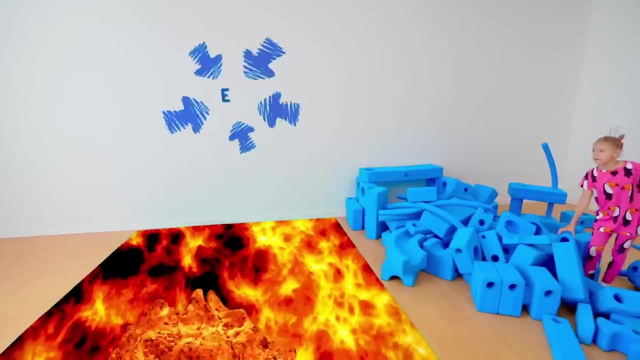 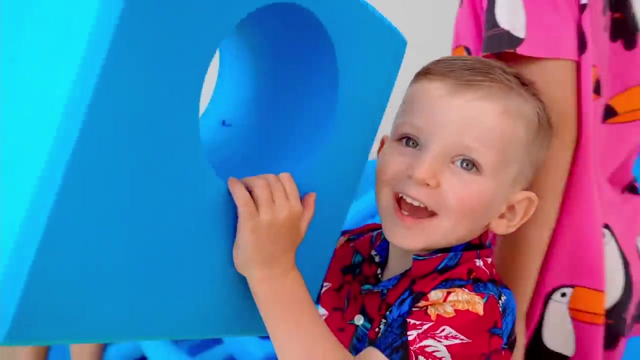 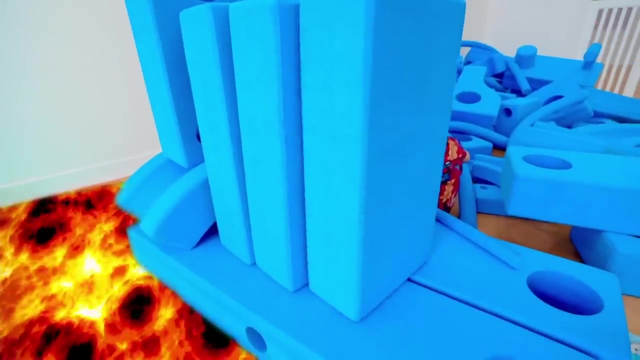 Let's find letters, Rock Letters. Hey, Hey, Hey, Let's go. Yahoo, Rock, Rock The looter. Oh no, It's lava. I have an idea. Let's build a tower. Yeah, I think it's high enough. 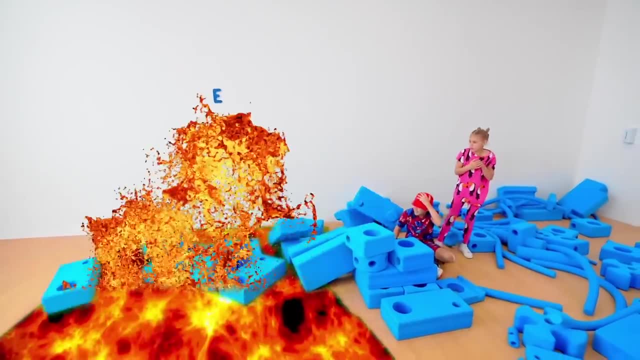 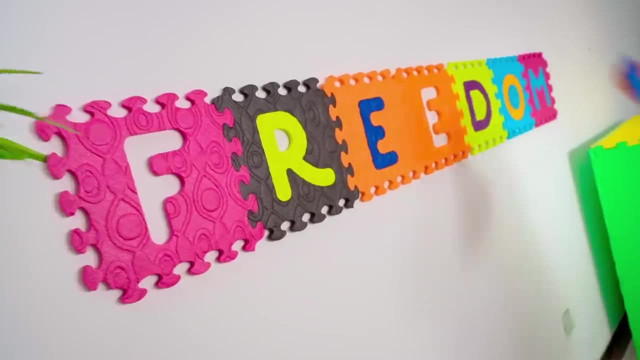 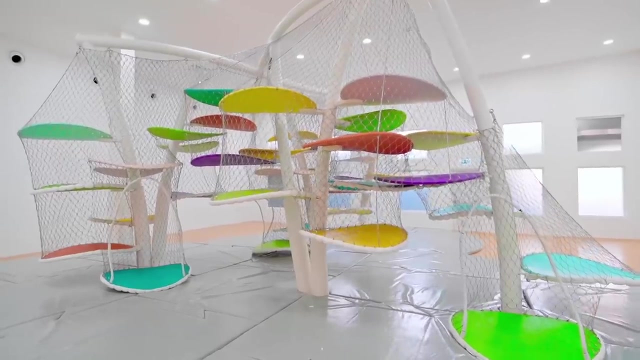 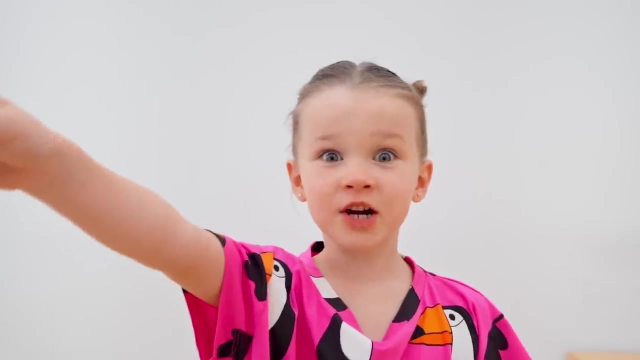 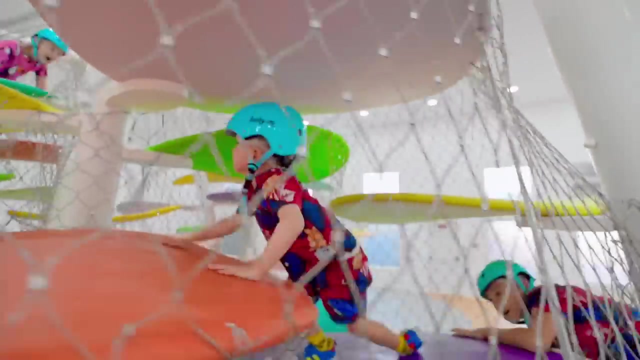 Oh yes, Wow, Wow, Wow, Wow, Wow, E, E, Wow, Wow, Ah-ha, Ahem, There's letter. Uh, oh, Oh, no, Oh yes, Wow, I got it. Fantastic Earth. 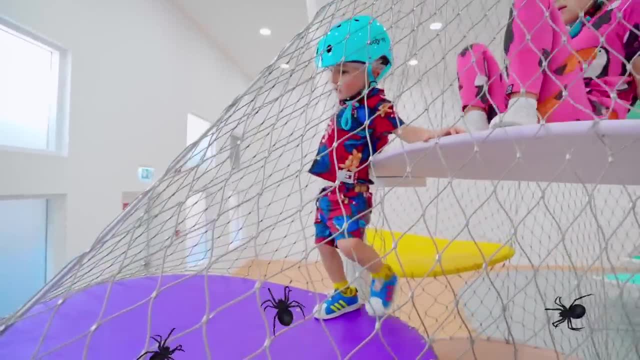 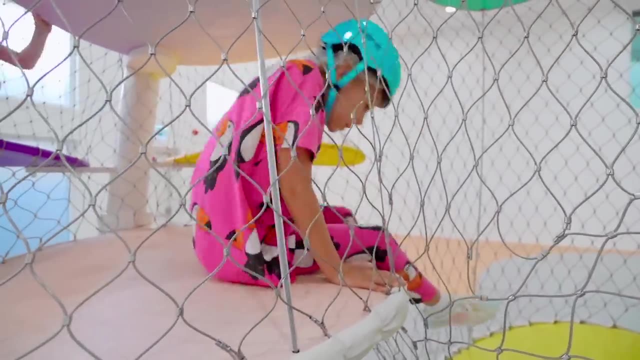 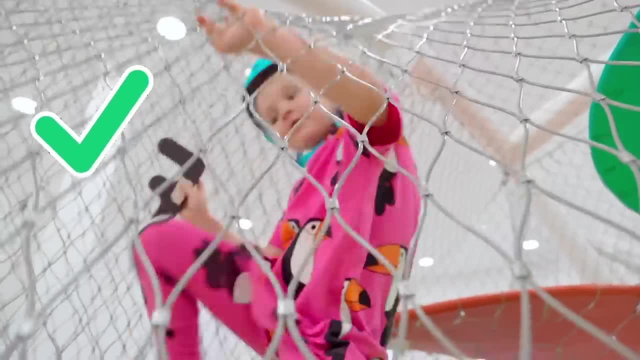 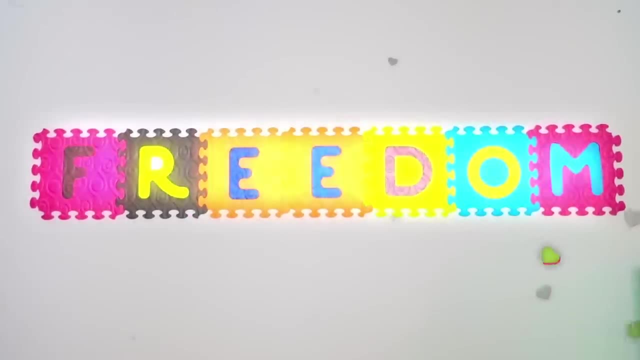 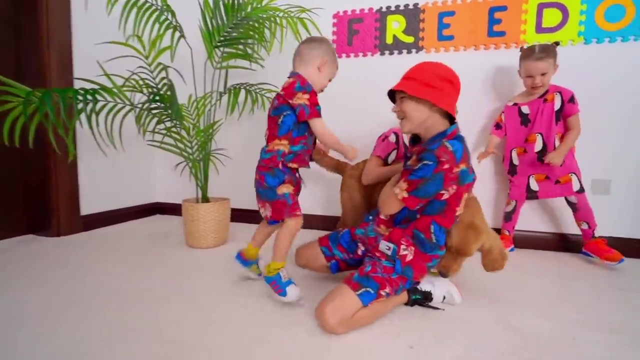 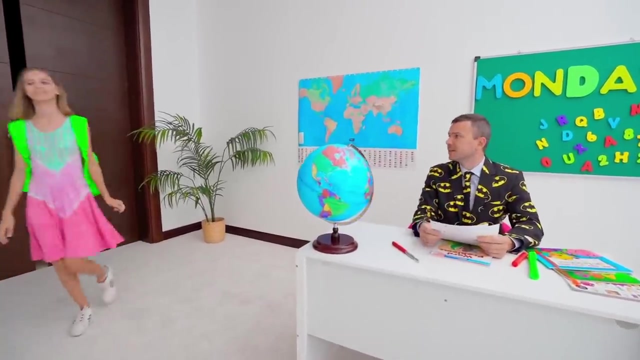 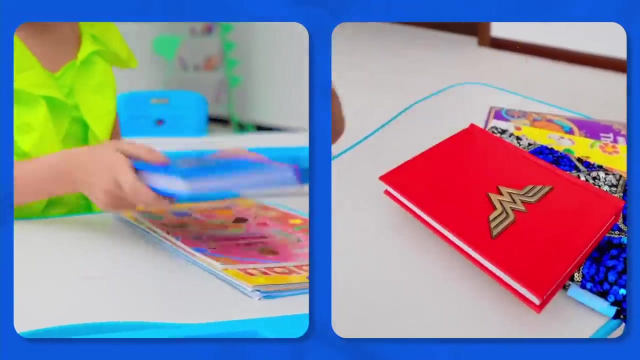 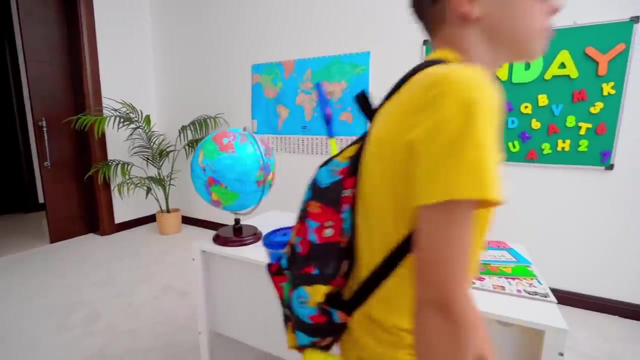 I got it. Fantastic Earth Freedom. Yay, Ho, Yay, Yeah, Yeah, Yeah, place, oh yes, fantastic, wow, wow, i'm ready. wow, oh, guys, meet our new student ivan. wow, oh no, hey, be careful. hey, excuse me. 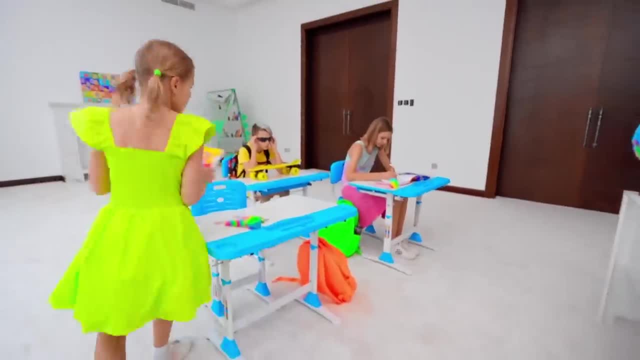 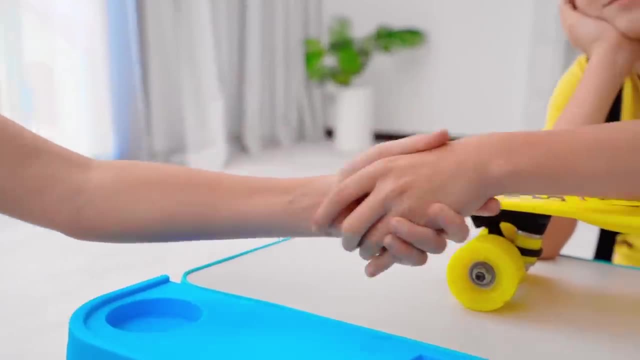 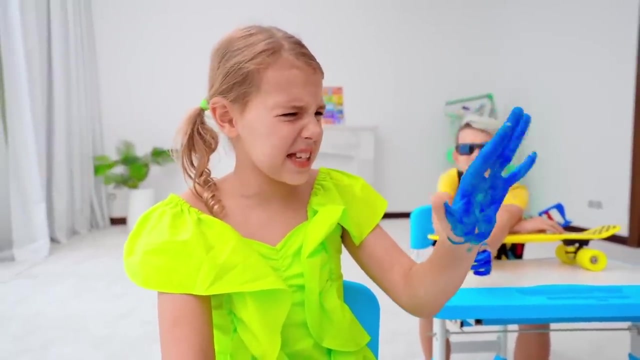 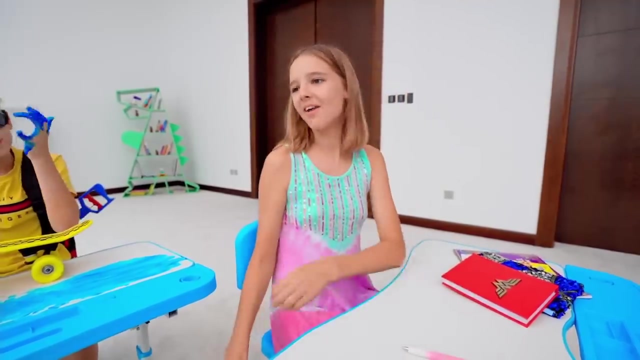 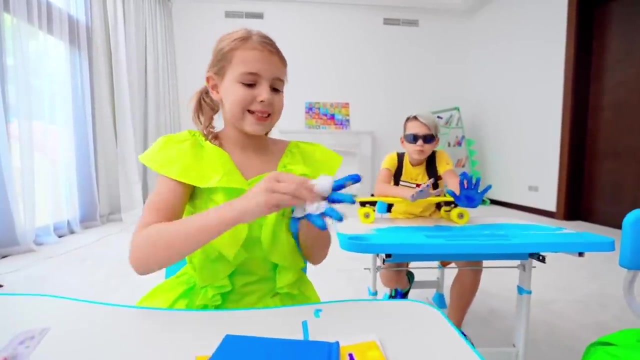 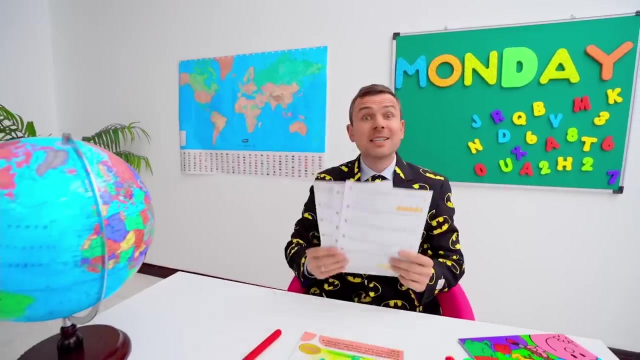 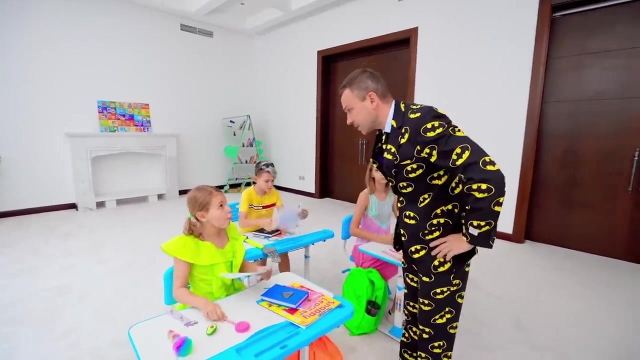 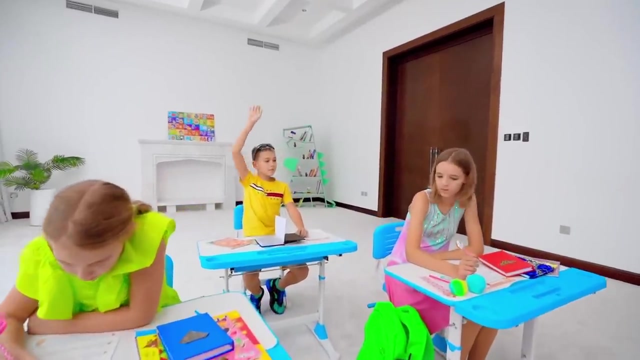 sorry, are we good, sure? yes, oops, oh no. what is that? oh no, what should i do? don't worry, i have something for you. excellent, thank you, wow. thank you, alice, you're welcome. it's time for this. wow, you have 10 minutes. oh no, oh no, excuse me, i forgot my pen, oops, no worries, i have a spare one. 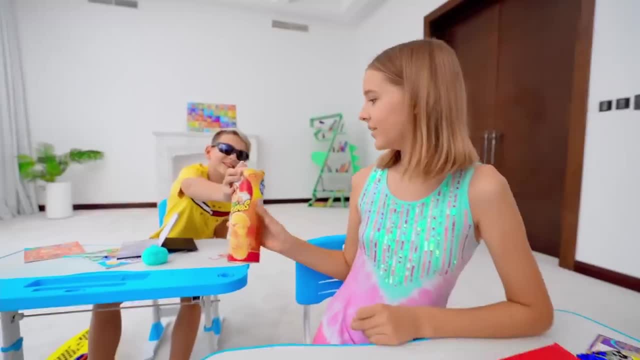 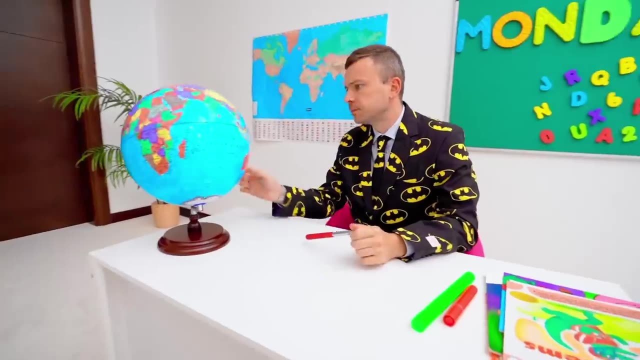 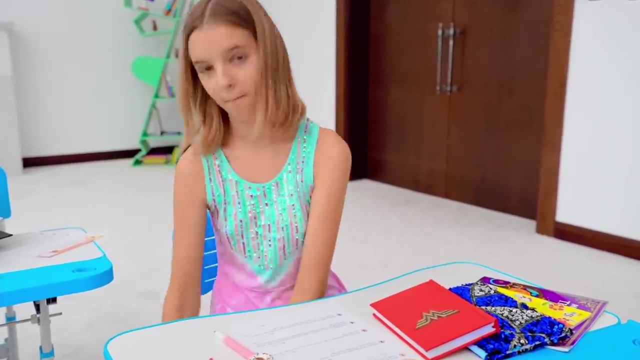 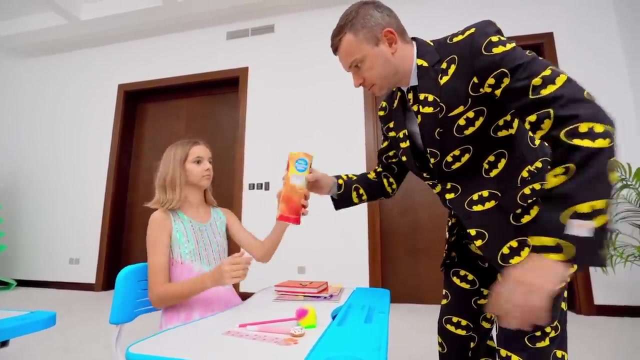 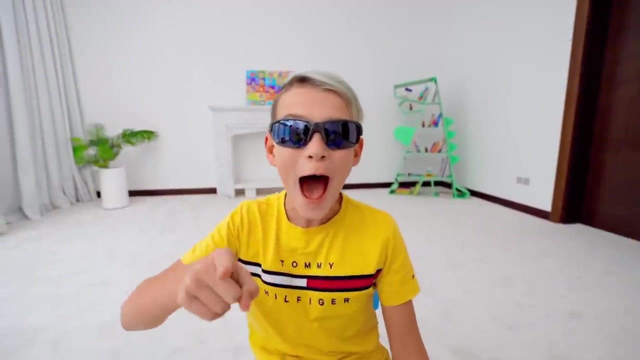 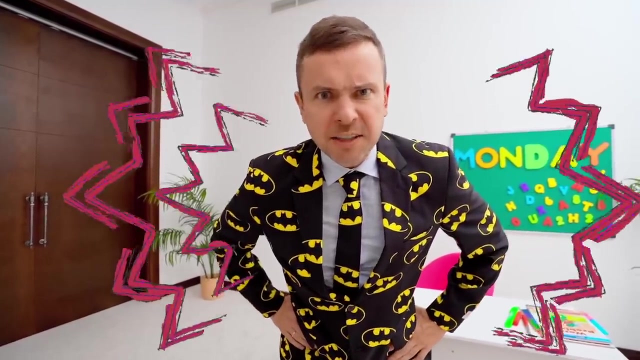 alice, thank you for the pen. this is for you. thank you, what's that? oops? hey, junk food is forbidden. give it to me, okay. wow, wow, ivan gave it to me. pranks are not tolerated in my class. it will not happen again. get back to work. 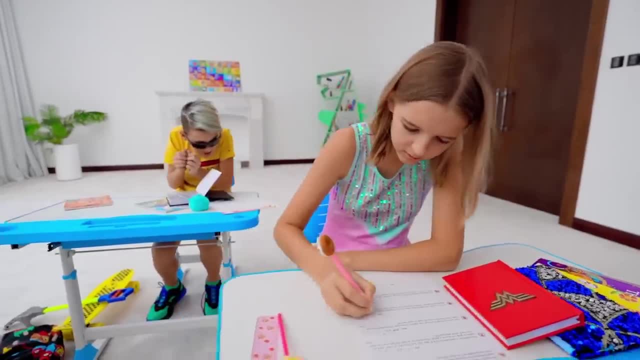 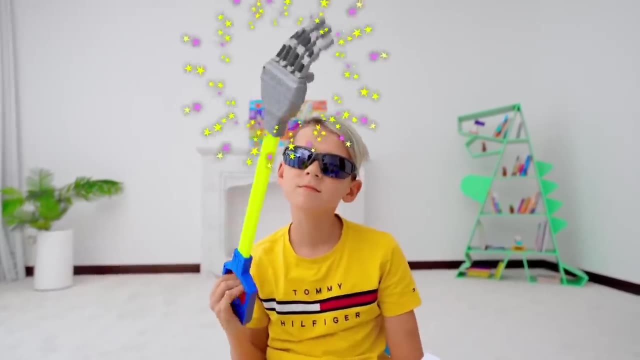 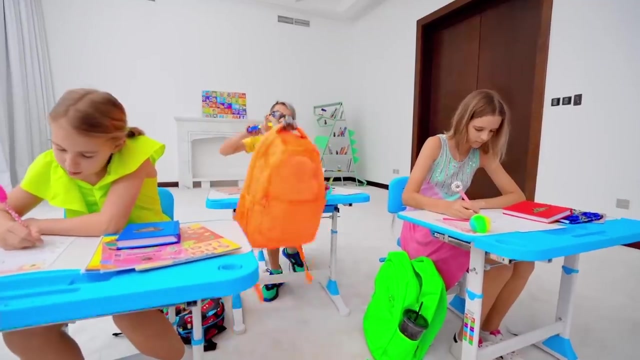 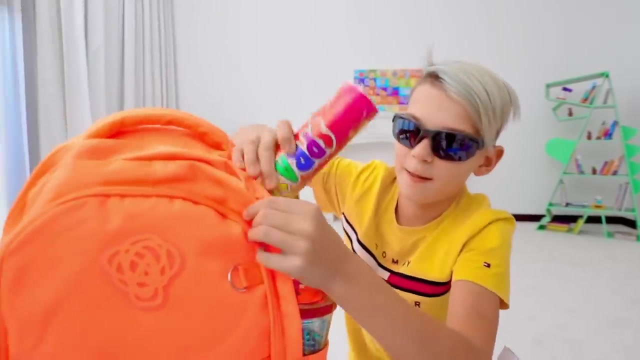 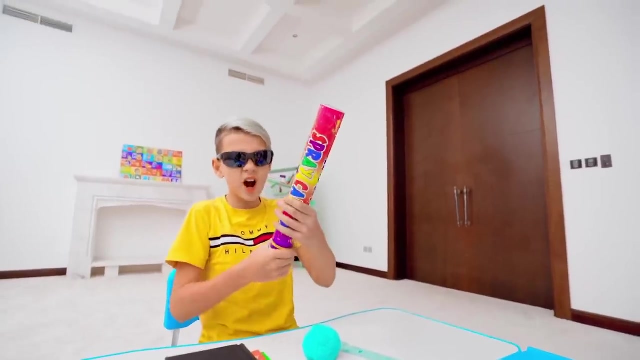 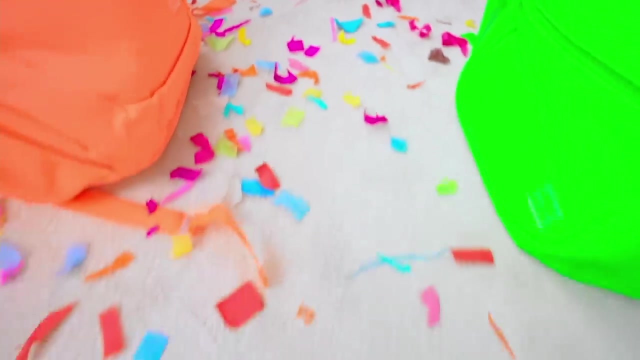 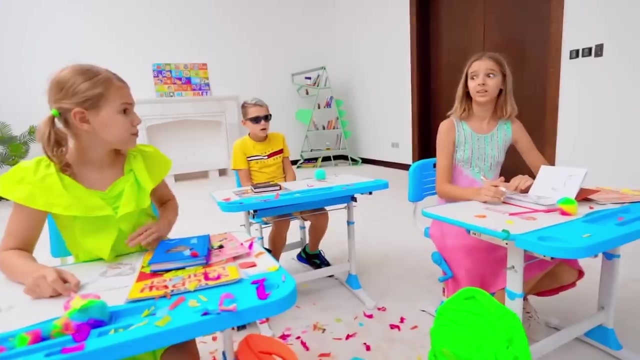 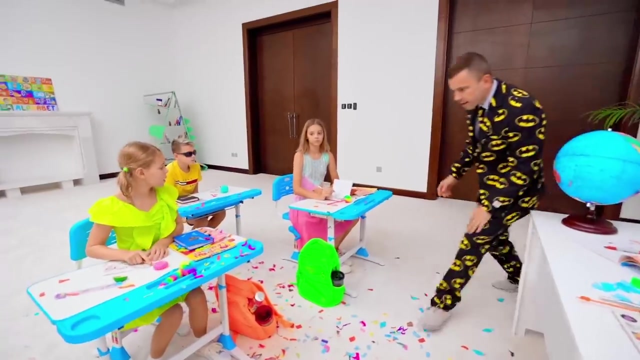 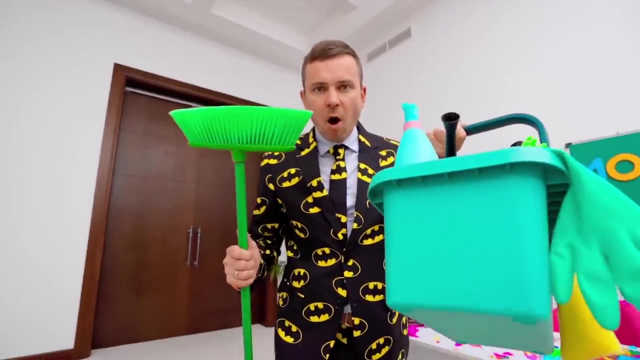 it sure will. oh no, hmm, no way, idea. wow, wow, wow, oh no, surprise, surprise, No way. Who did this? It's not me. Check there. Wait a minute. What's this? I've never seen it before. Clean all this mess. 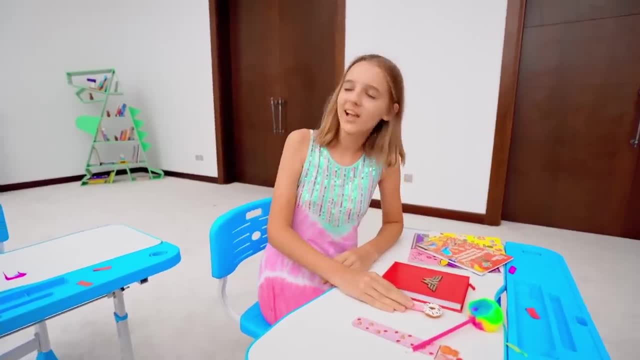 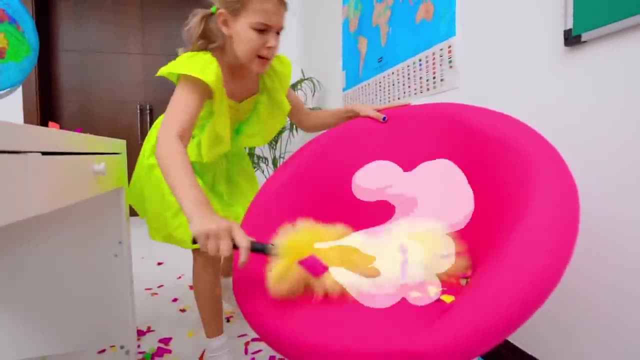 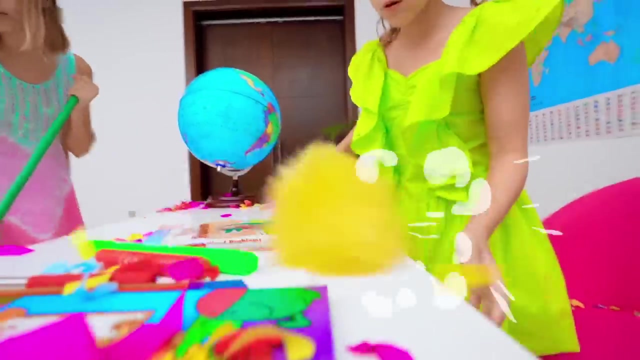 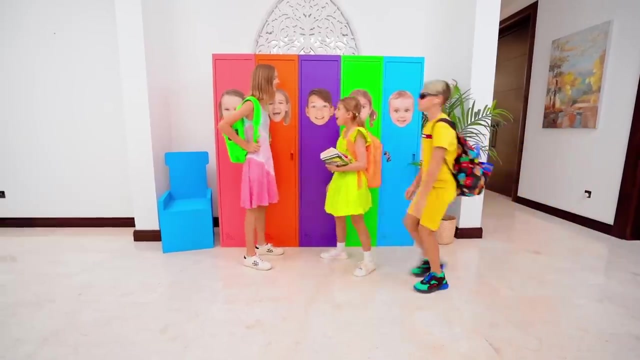 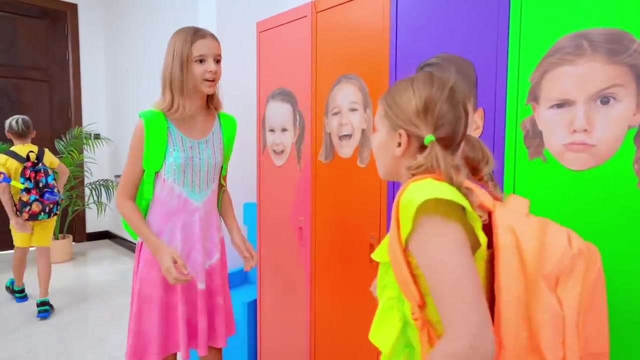 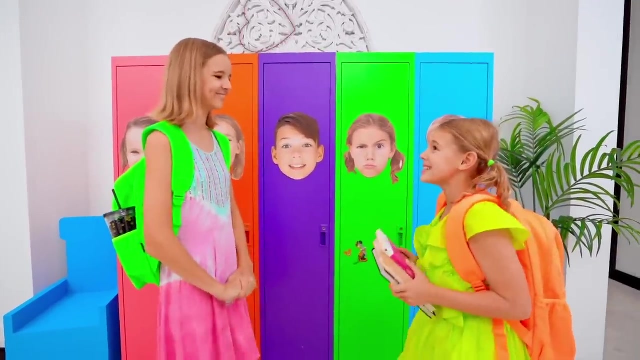 Enjoy, Don't worry, I'll help you. Yahoo, Yes, Oh, yes, Excuse me Ouch. What are you doing on the island, Are you okay? I'll help you. Thanks Here. Thank you, my bestie. 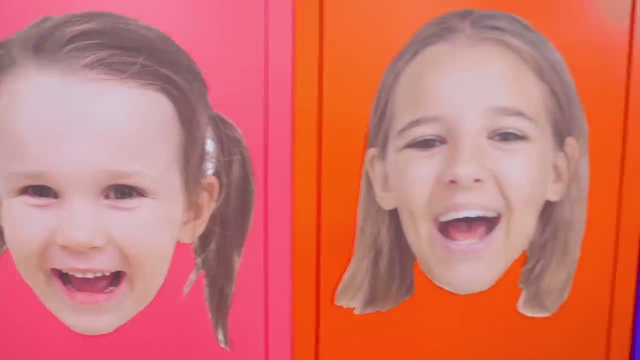 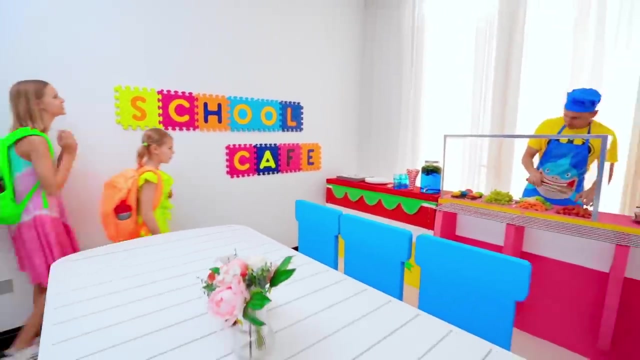 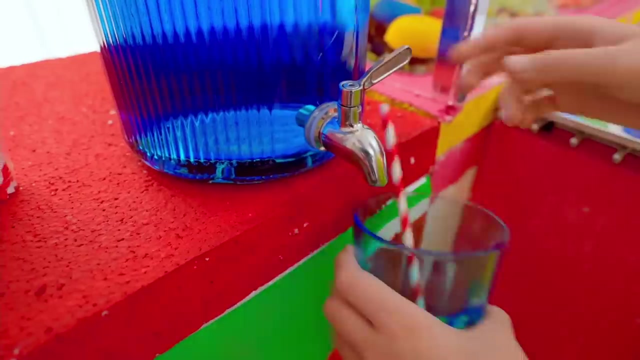 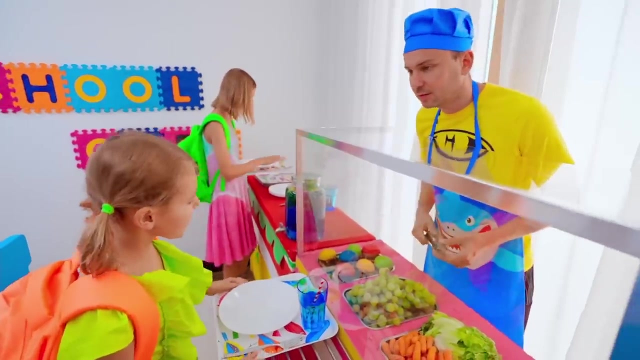 Let's come to the school cafe. Yay, Wow, Excellent. Ivan is so annoying. I know He sucks Hi. Hello there, What do you want? Can I have a burger? Yeah, sure, Give me a plate. 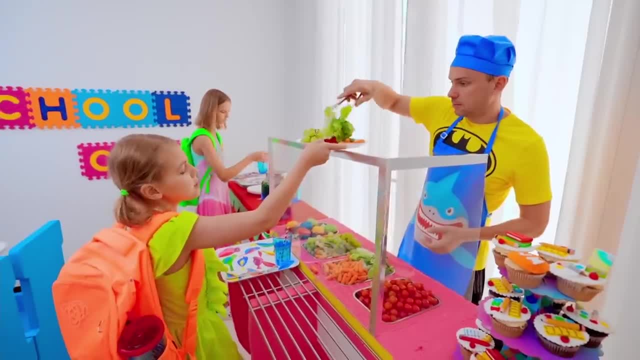 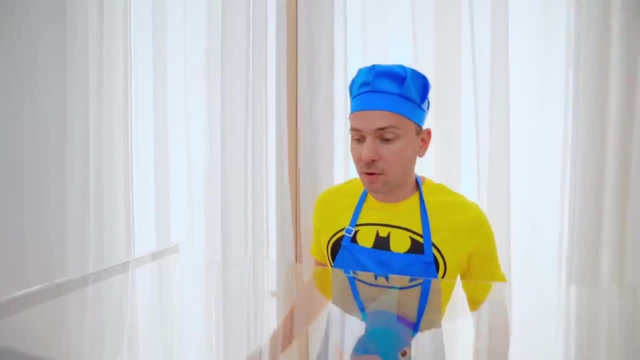 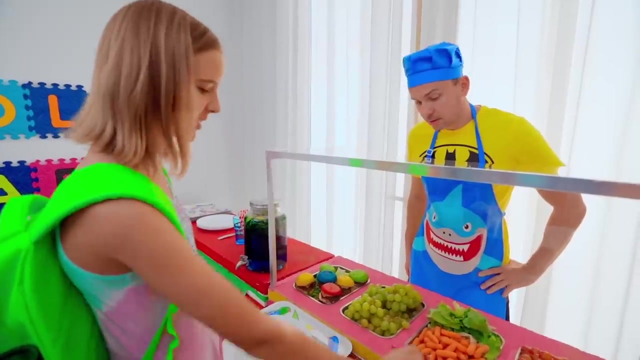 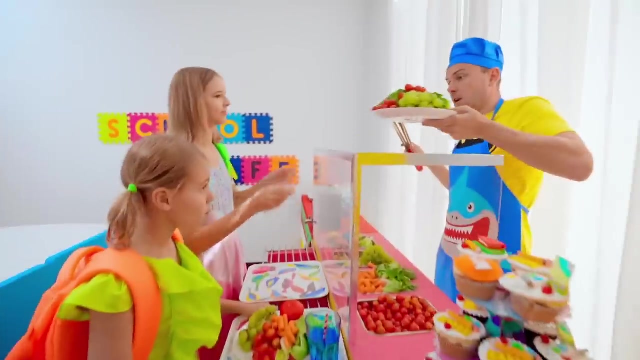 Grape carrots and lettuce And tomatoes. Here you go. Thank you, Hi, Alice. What's for you? Can I have the green burger and the yellow one? Grape carrots, lettuce and tomatoes. Two burgers, Yeah, Okay, Here you go. 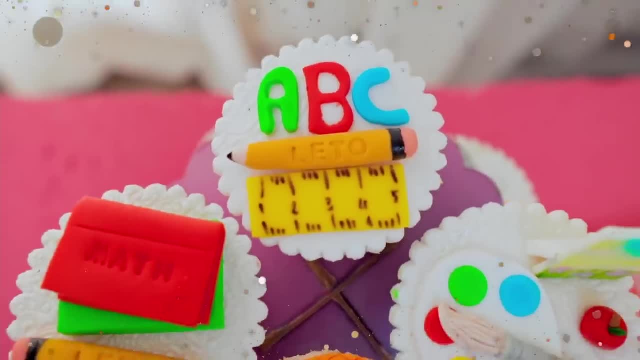 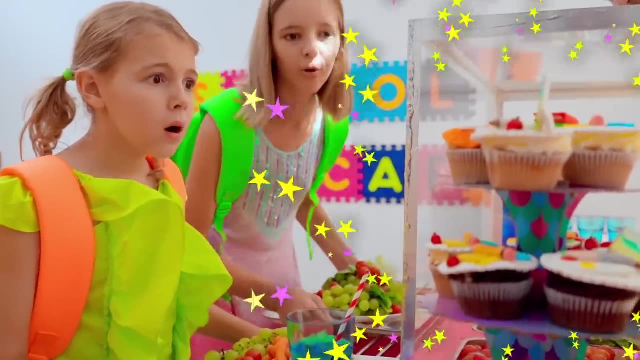 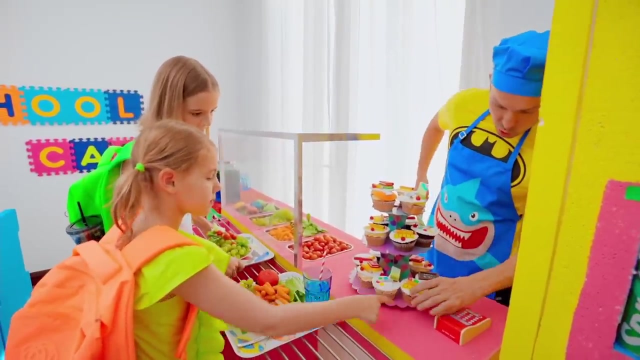 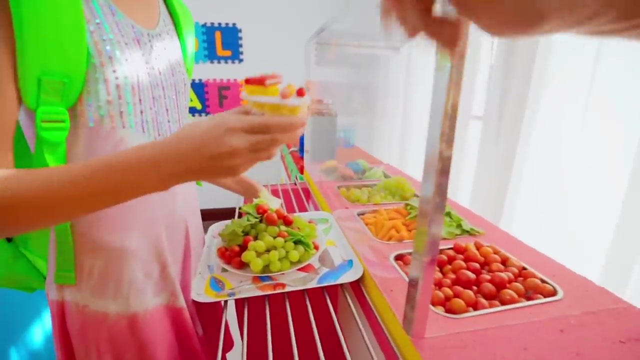 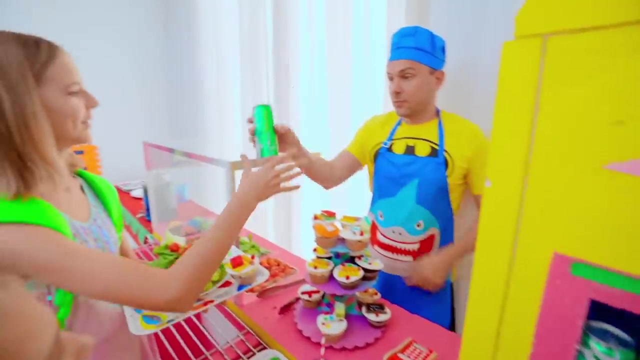 Thank you. Wow, Wow, What's this? It looks so nice. Choose one. Can I choose this? Sure, This one, Here you go. Thank you. Can I also have one soda please? Sure, Here you go. 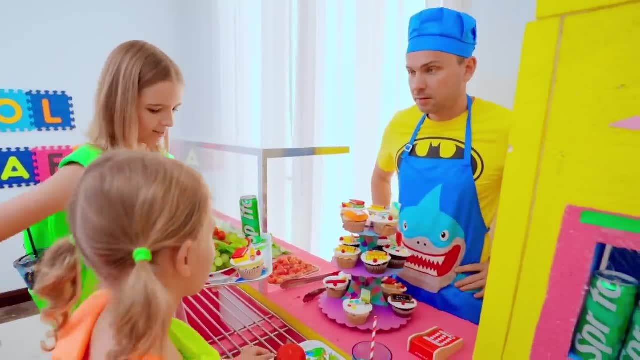 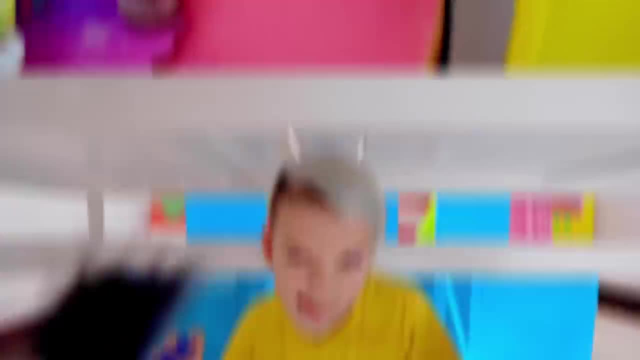 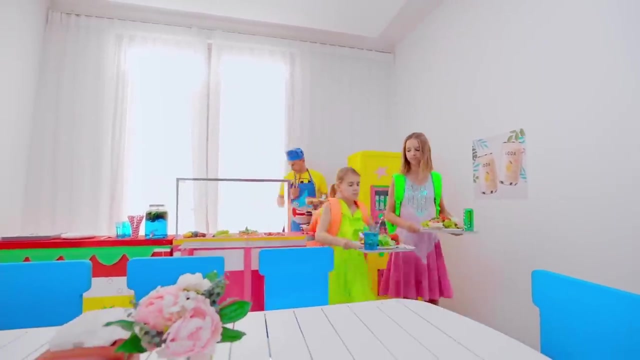 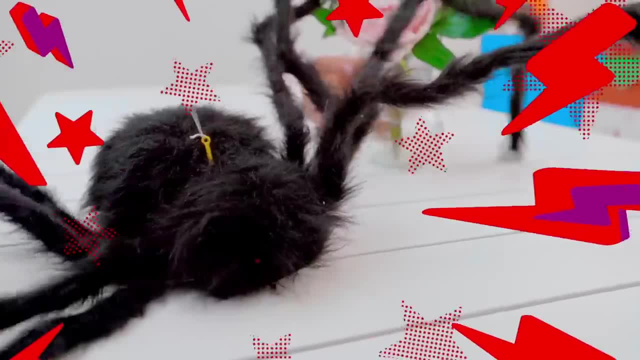 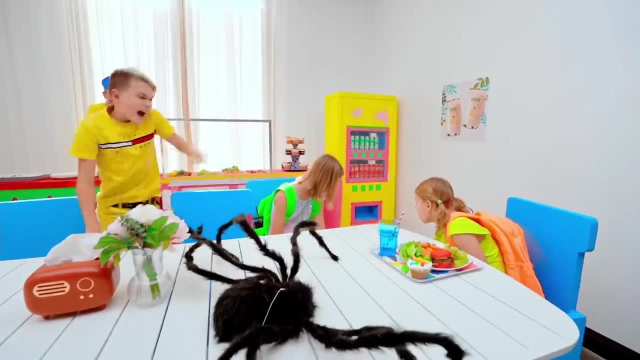 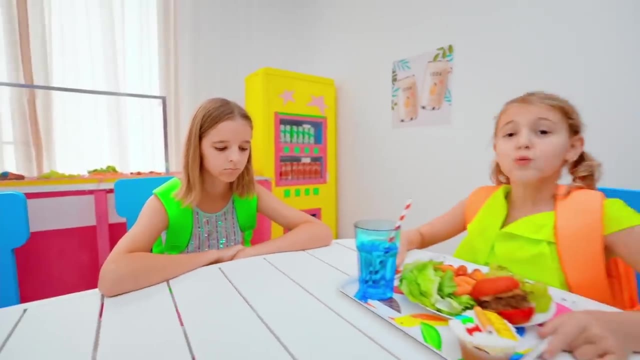 Oops, Oops, No way, Oh no, My food, My 300 bucks, Haha, Gotcha, Excuse me, Don't worry, I can share. Thank you, You're my bestie. Bleh, You're my bestie. 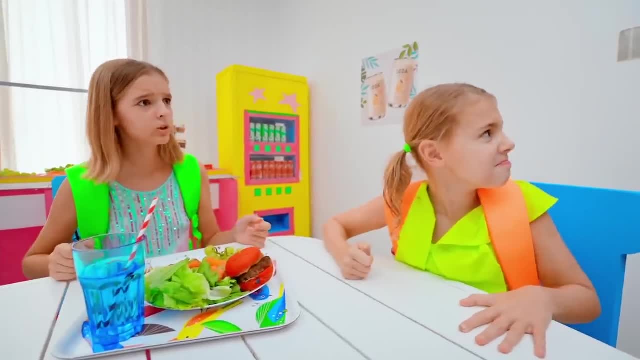 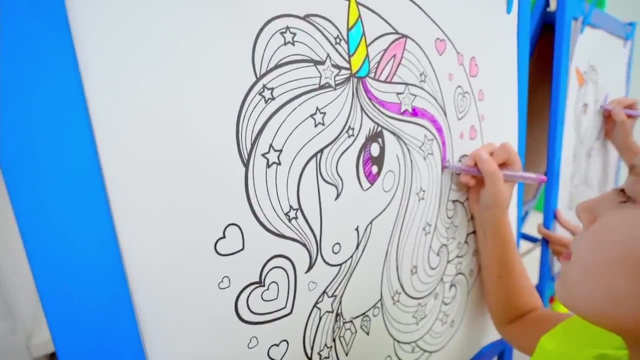 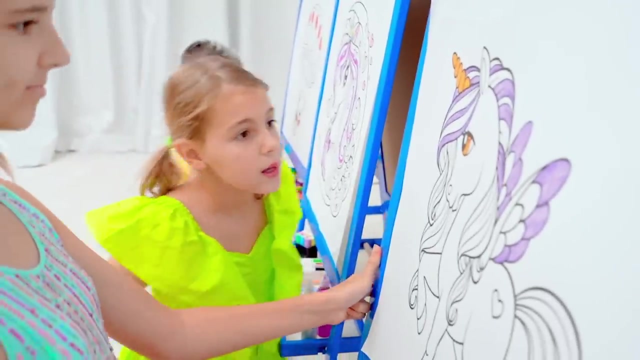 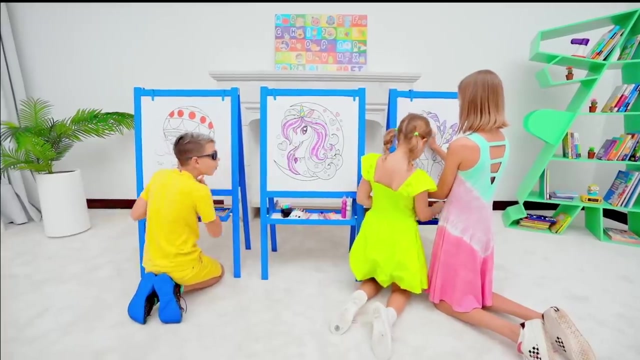 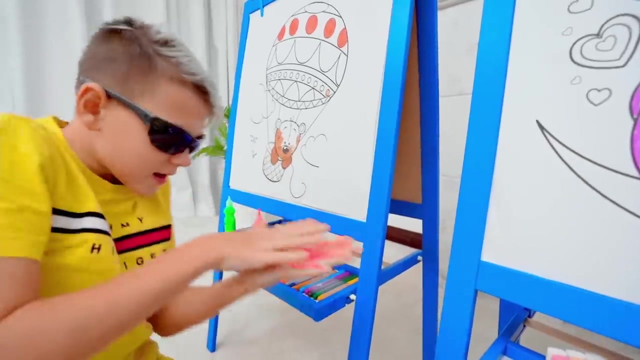 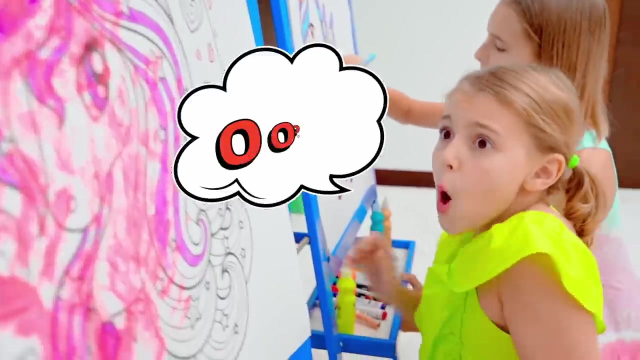 Hey Ivan, I read this. Maria, look How do you like it. Wow, It's so nice. Can I help you? Sure, Hey, Aha, Wow, Oops, Puyo, Puyo, Puyo. Oh no, My drawing. 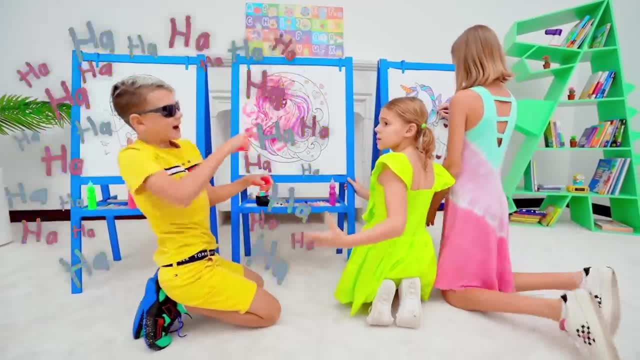 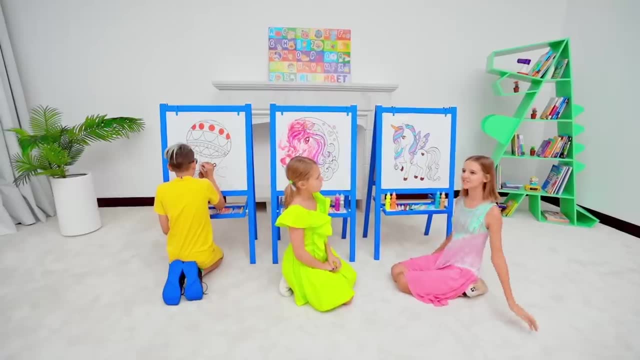 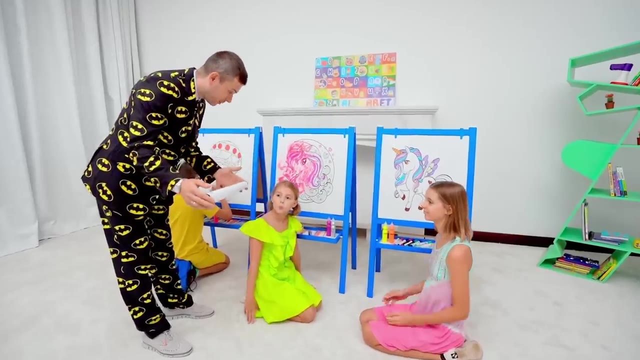 Oh no, Hahaha, Huh, Don't worry, We can take a new sheet and I'll help you. Thank you, Mr Teacher, come here. Hello, We need a new sheet because this one is ruined. Sure, I have something for you. 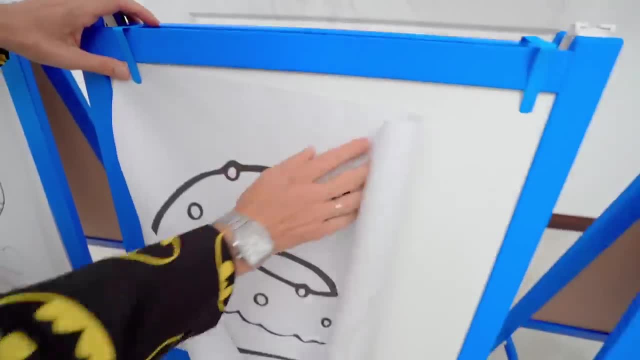 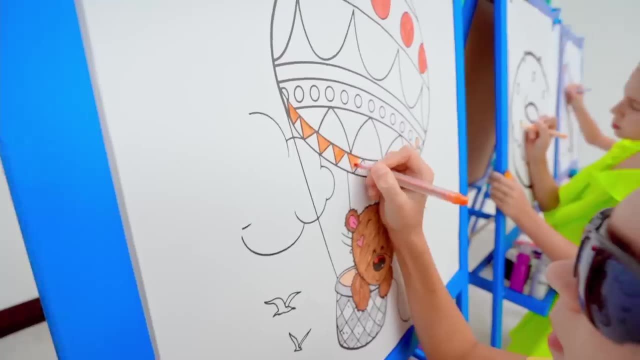 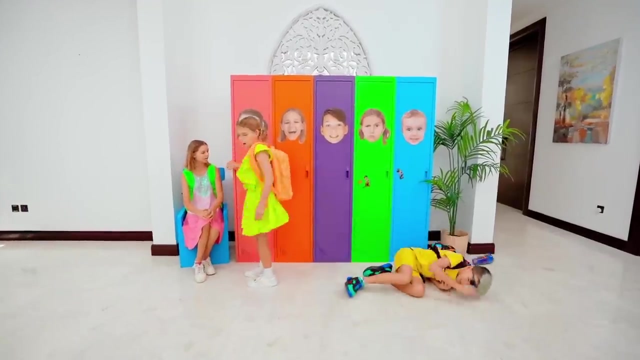 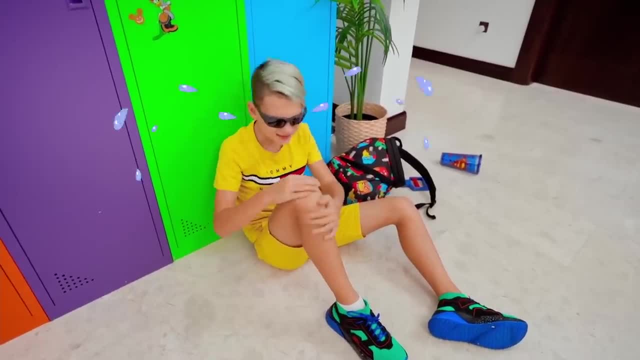 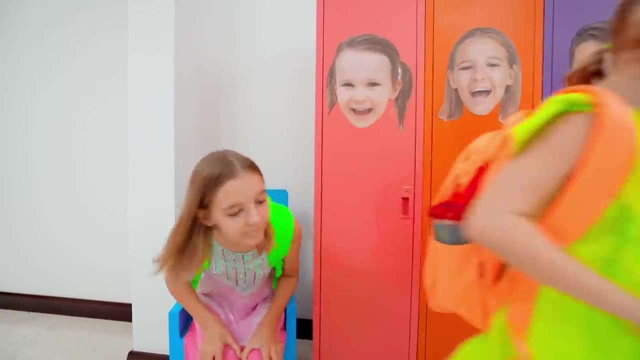 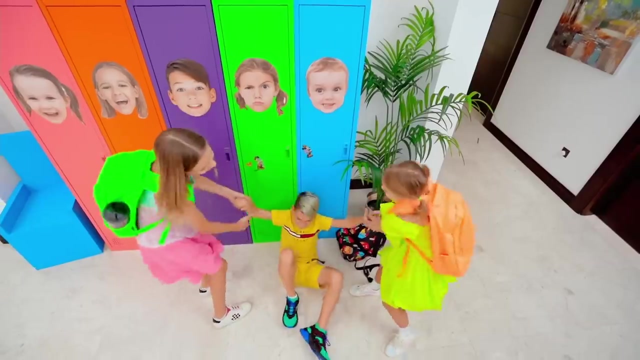 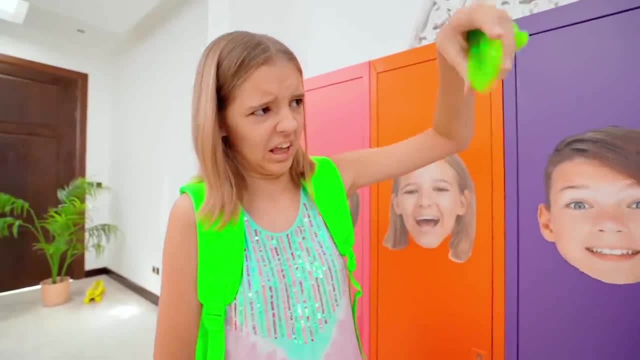 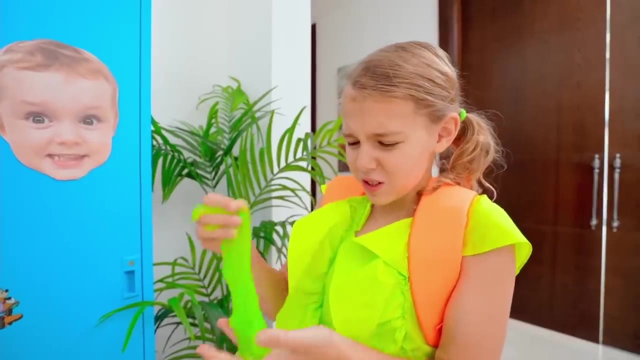 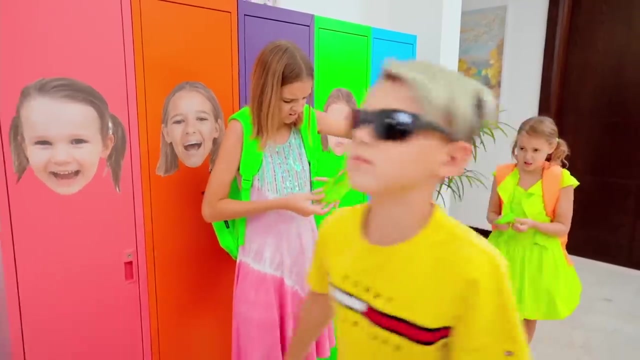 Ew, What's that? Puyo, Puyo, Puyo, Puyo, Puyo, Puyo, Ew. Hahaha, Ivan, what did you do? Thank you for helping. Thank you for helping. Wow, Wow, That's it. 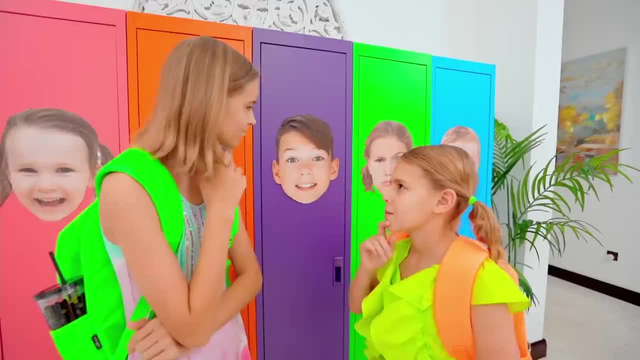 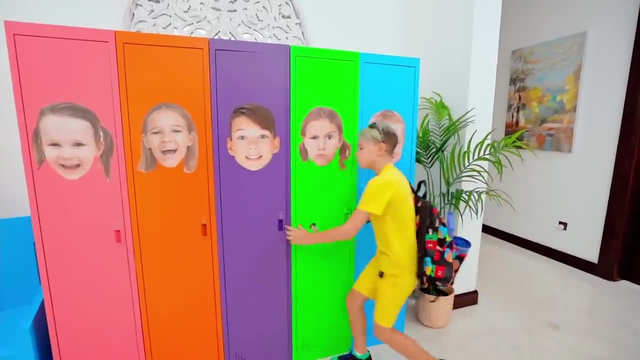 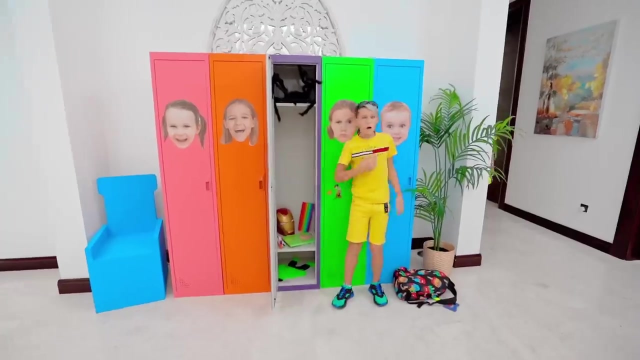 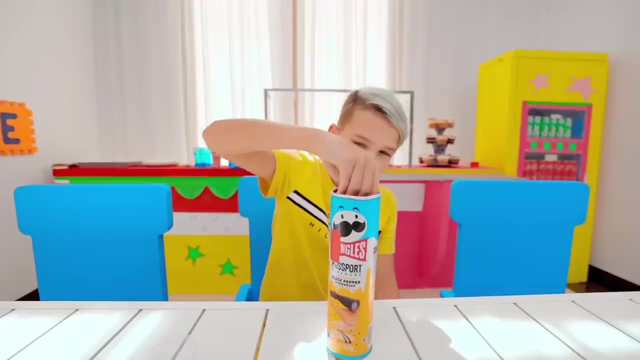 But how should we do it? Hmm, Aha, Yeah, Hahaha, Woops, Woops, Oh, What is this? What is this? No way, Little baby got scared. Hahaha, Hahaha, The Wonderful World. 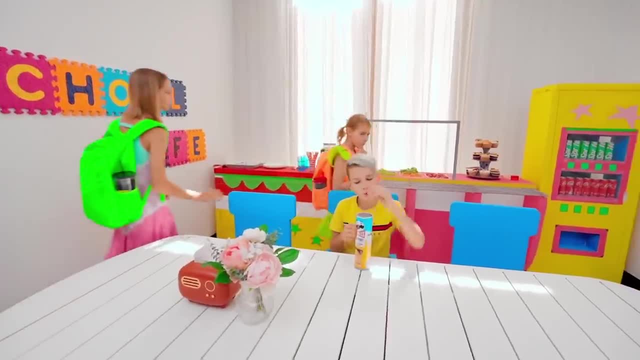 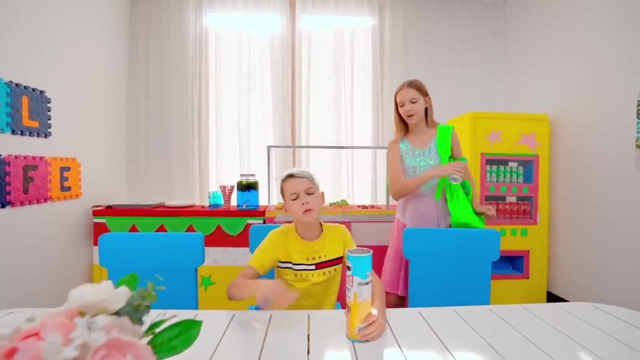 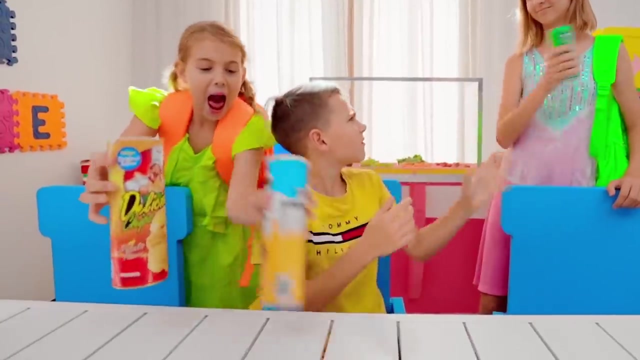 The Wonderful World. Aha, Oh yes. Yes, Ivan, could you please help me open this, can? I'm not strong enough. I'm not strong enough. Give me that, you little. Give me that, you little. Oh yes. 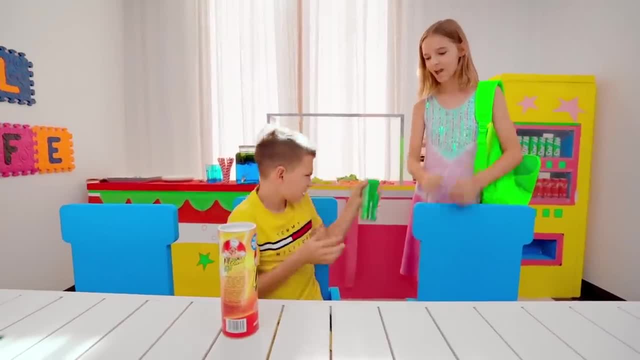 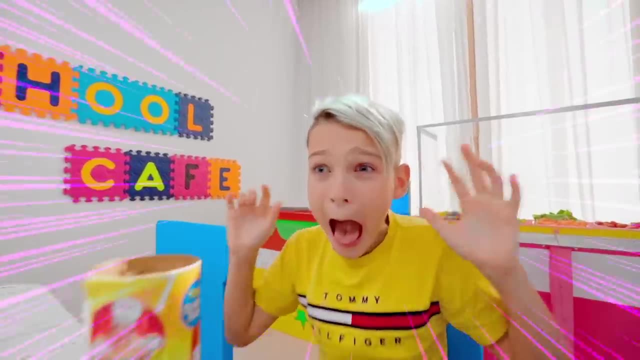 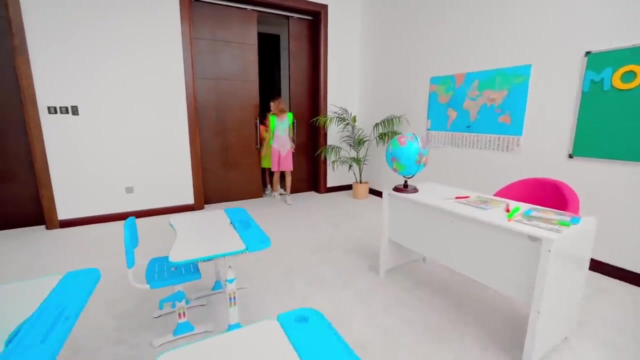 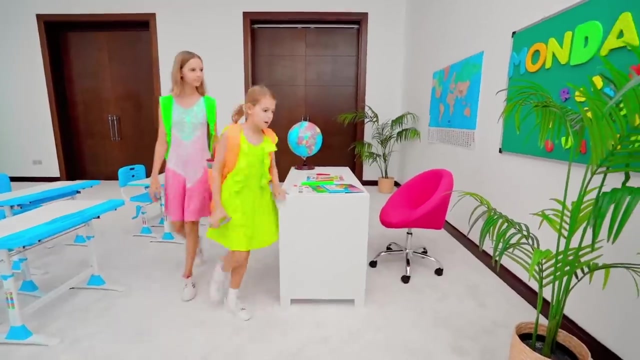 Oh, yes, Wow, Thank you, Bye. Oh no, Hahaha, Loser, I have an idea. This will help us. Let's go. We need to hide a camera here. We need to hide a camera here. 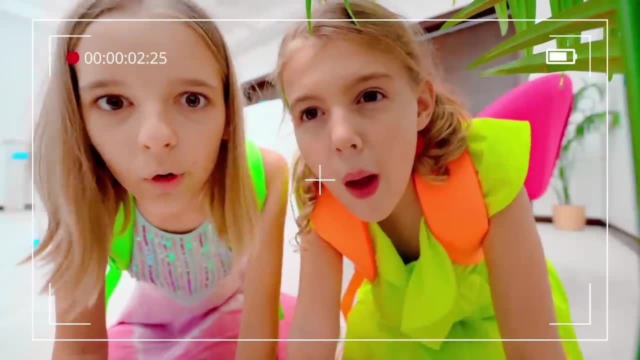 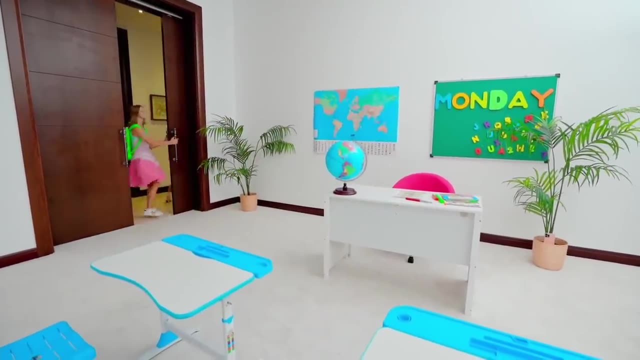 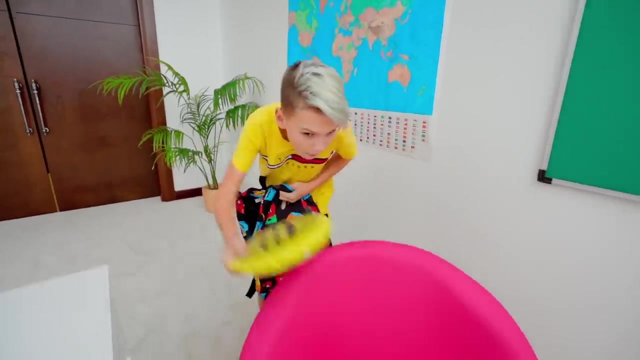 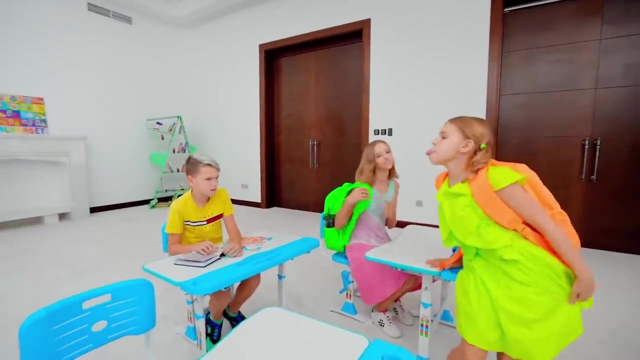 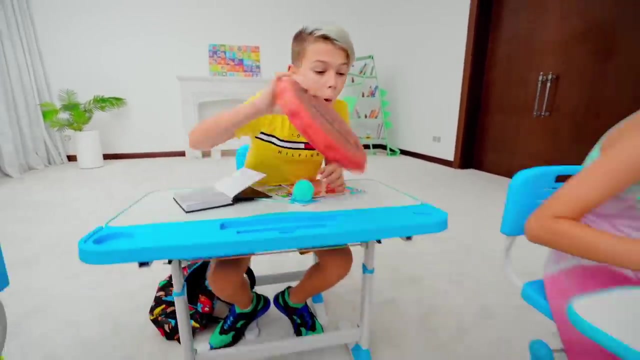 Fantastic. Okay, it works, Let's go. Woohoo, Woohoo, Woohoo, Oh no, Oh no, Won't you prove it? Uh-huh, And together with this little woman, we will get the業.